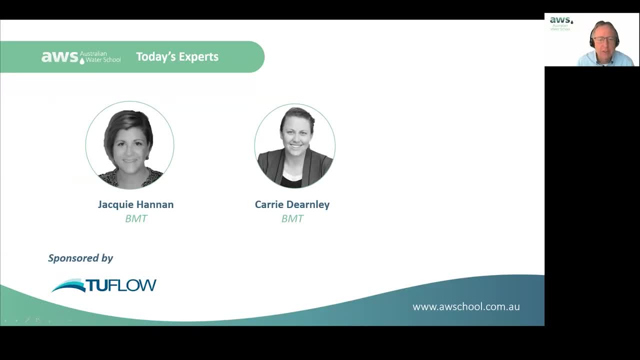 All right, let's have a look at who will be talking to us today. Jackie and Carrie and their colleagues Do come on screen everyone. Thanks, Carrie, Thanks Jackie And Anne and Tegan and Bill. their colleagues, Welcome everyone, So appreciate it. 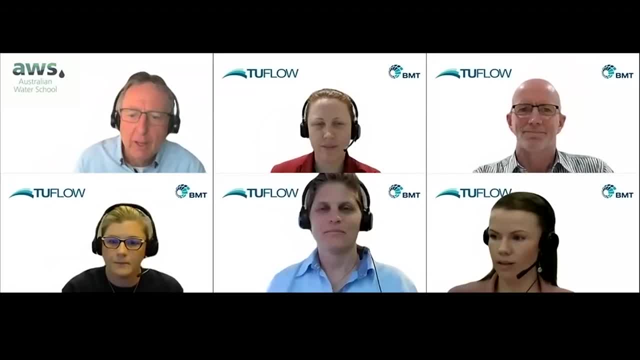 So, Carrie and Jackie, you're going to be presenting, And Bill and Anne and Tegan will be ready and raring to answer your questions and comments. in the background, Carrie, Jackie, tell us where you're from, Jackie. So I'm in sunny, Sydney, Australia. 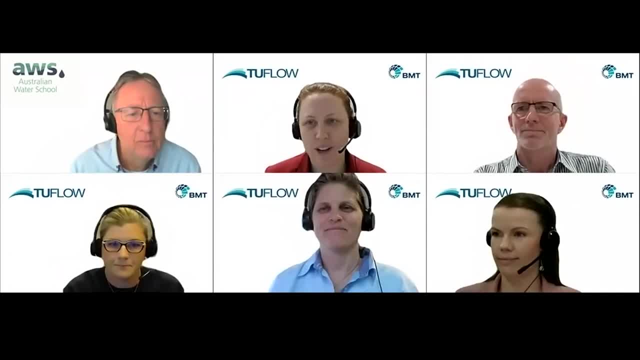 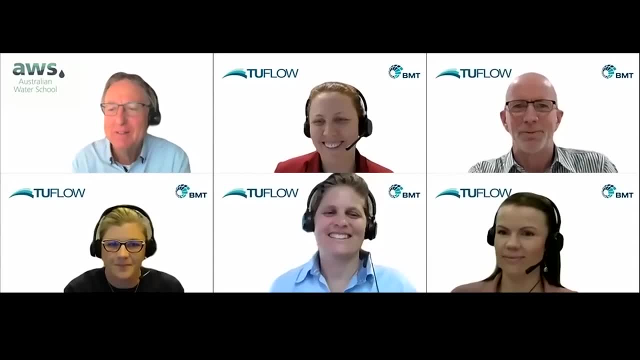 Right, OK, And Carrie, I'm in Brisbane, Australia, probably sunnier than Sydney, Right, A little bit of competition there. And where are you, Bill? I'm up in Brisbane enjoying the sun, Enjoying the sun, And Tegan. 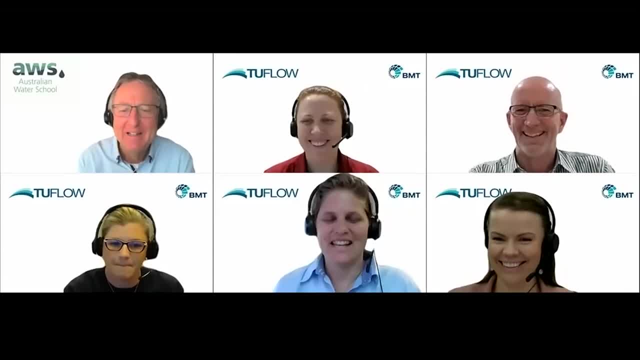 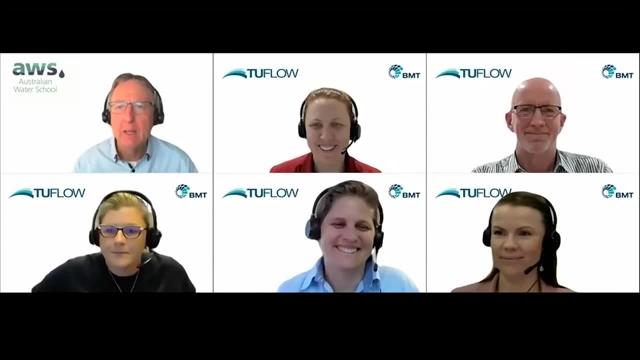 That's right, I'm just behind Carrie And Anne As well. I'm in Brisbane. Oh, well done, Well done. I'm in drizzly wet, cold, cloudy, foggy, windy Adelaide Hills. Yes, right, But we're going to make it a fantastic day though. 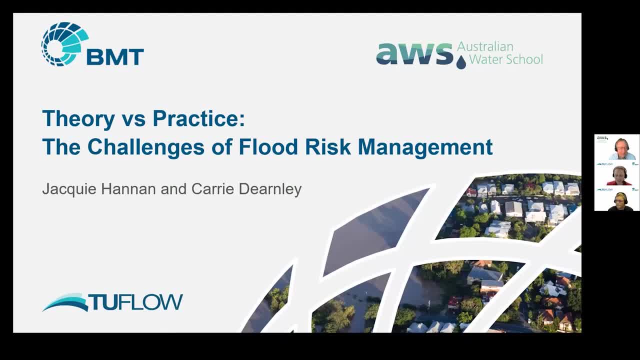 Right over to you then, Carrie. Thank you, Trevor. All right, So yes, we're talking about flood risk management today, And I think it's something that we intuitively feel should be quite easy, But once we get stuck into it, we find it's actually much more challenging than we expect. 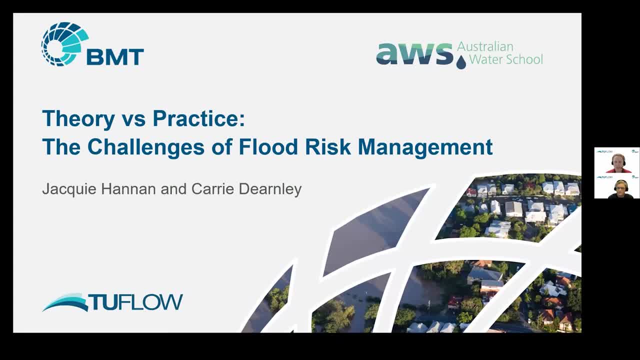 That we have faced lots of decisions and need to make recommendations that are really hard, despite there being some great guidance around. So Jackie and I are going to be talking to this topic today. So the best practice approaches, but also what happens in reality and how to deal with those challenges. 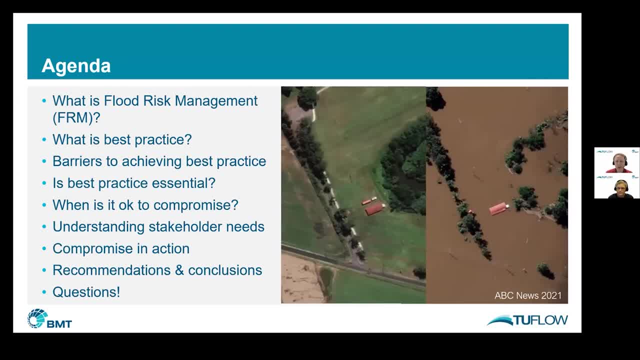 So these are some of the topics we're going through. Jackie will be starting and she'll introduce you to the principles of flood risk management, What constitutes best practice- But then she'll start to bring in some of those sticky points. So what are the barriers to achieving them? 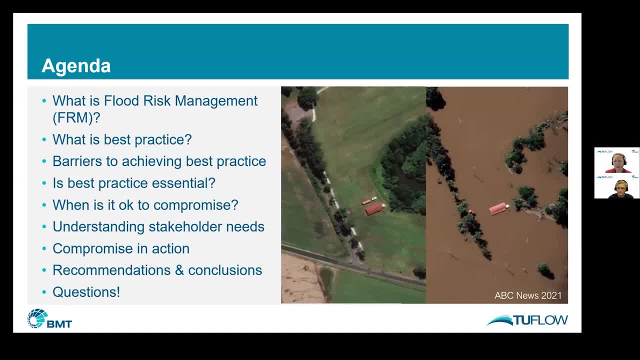 What are the barriers to achieving that best practice? I'll take over from there and let you know when is it OK to compromise, if at all. So we'll come back to those poll questions that Trevor just reported on, And from there we'll bring in a few other issues. 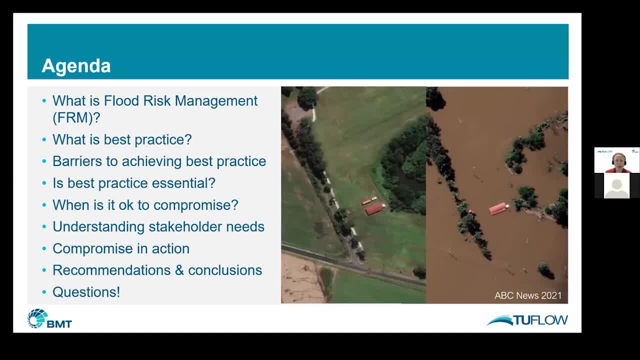 So stakeholder needs are a really important part of flood risk management, and particularly if we want to start compromising. And then, finally, I've got a couple of examples to work through so you can start to understand this framework that we put forward for you. This idea of reconsidering some of the decisions that are being made. And then, finally, I've got a couple of examples to work through so you can start to understand this framework that we put forward for you, This idea of reconsidering some of the decisions that are being made. 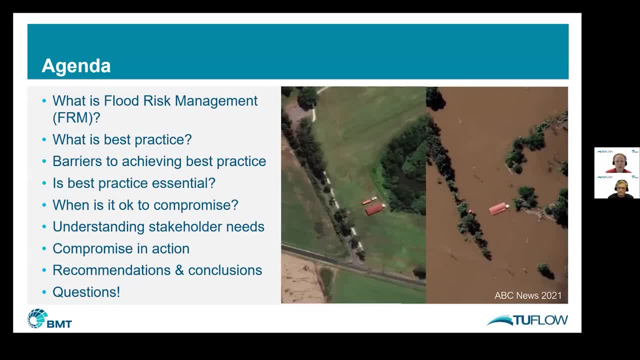 And then, finally, I've got a couple of examples to work through This idea of reconsidering some of the decisions that are being made And hopefully use those learnings in the future. And we'll wrap up and then have some time for questions. 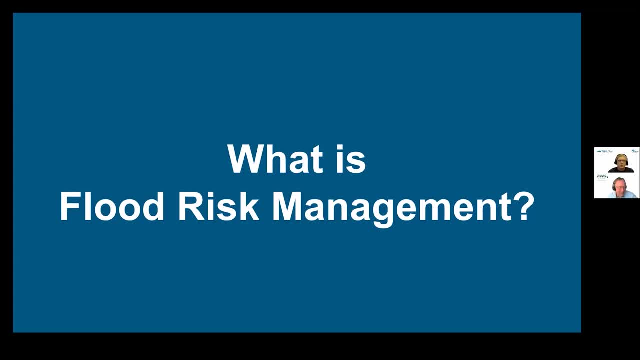 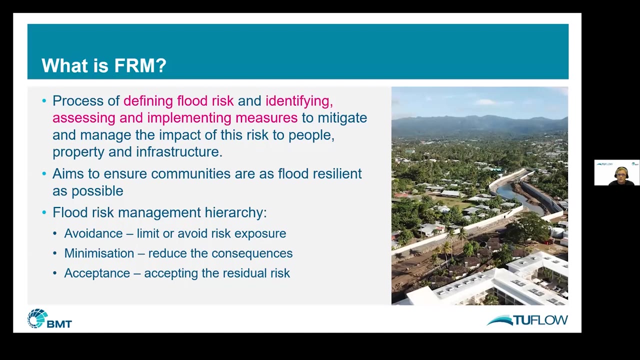 Thanks Jackie, Thanks Carrie. All right, so before we jump into talking about best practice, I suppose it's good to firstly give a bit of background, to define what flood risk management actually is. So, basically, it's a process of defining flood risk and then identifying, assessing and implementing measures to mitigate and manage the risk. 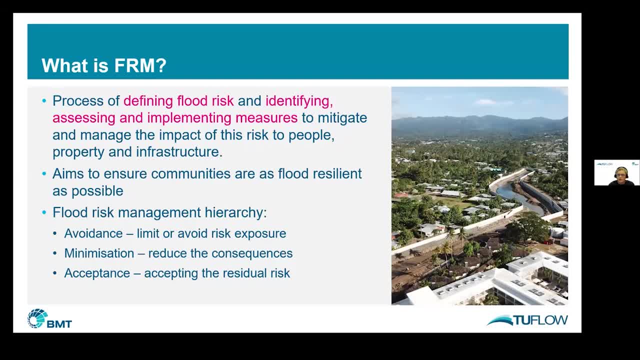 risk to people, property and infrastructure. it aims to improve community resilience using a broad risk management hierarchy that involves avoidance- so limiting or avoiding risk exposure. minimization- so reducing the consequences of the risk. and also acceptance- so accepting that there's some residual risk and understanding how to manage that. and flood risk management involves a number of key. 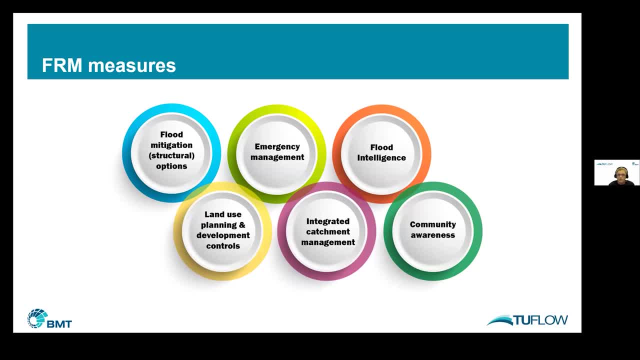 components with different measures that we can adopt. so there's flood mitigation options, which might be structural works. there's land use planning and development controls, emergency management, integrated catchment management, flood intelligence- so flood forecasting and warning systems. and also community awareness, which is really important, making sure. 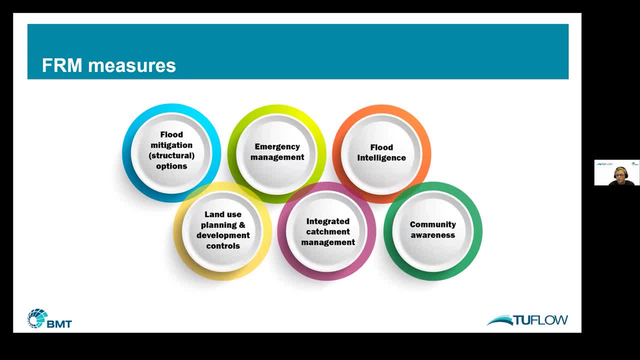 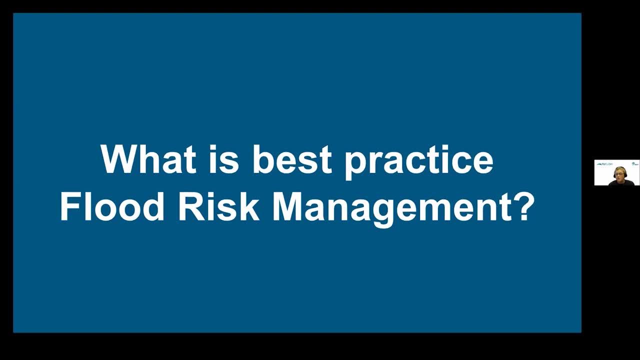 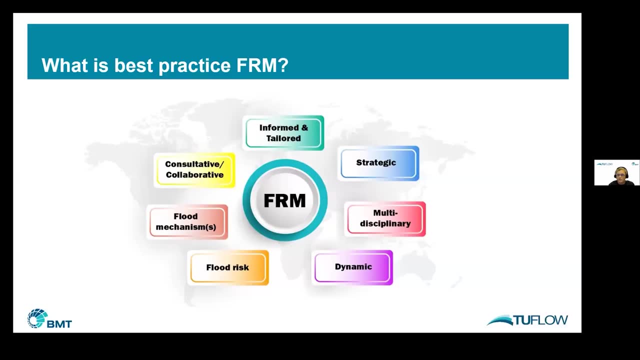 the community are aware of their flood risk and what to do before, during and after a flood, so management of the floodplain should be based on best practice. but what does this actually look like? so, essentially, when we talk about best practice, we're really referring to a set of 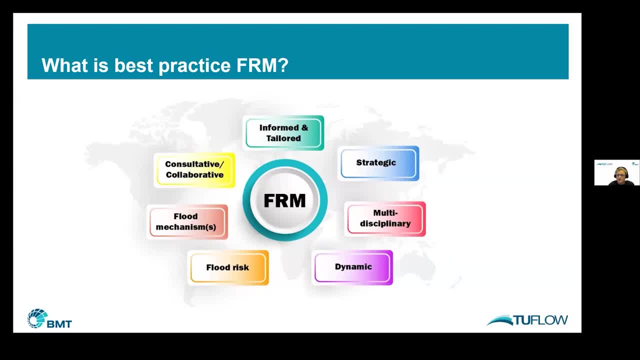 underlying principles that need to be considered when undertaking studies and formulating management plans for the effective, strategic and sustainable long-term benefit of the community and the environment within floodplains. so, from our experience, there are several key components of the floodplains that we consider contribute to best practice flood risk management. 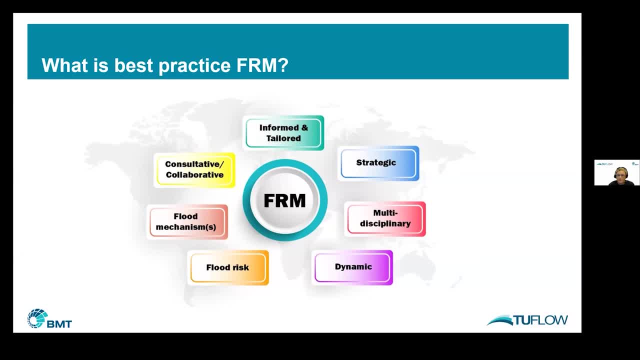 at a high level. this includes the components on the screen, so that is, it should be based on an understanding of the flood risk and the flood mechanism impacting an area, and it should also be based on an approach that is consultative and collaborative, informed and tailored strategic. 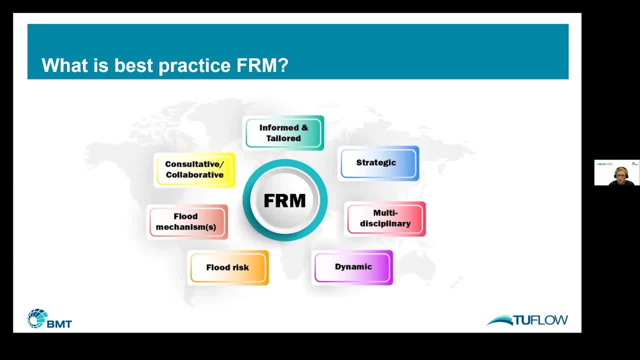 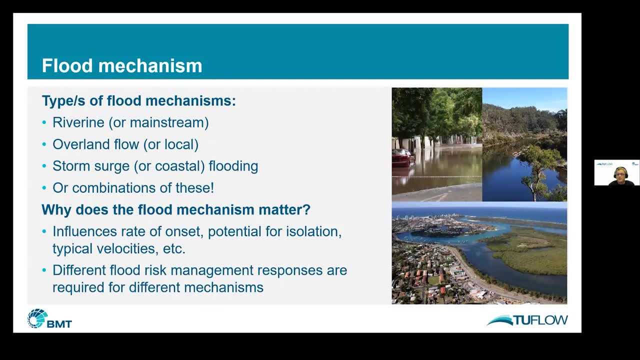 multi-disciplinary and dynamic, so i'll now go into a little more on each of these components. so, firstly, it's important to consider the types of flood mechanisms impacting an area. so what's causing the flooding? where does the water originate and where is it going? and why does this matter? well, it influences the rate of onset, the potential. 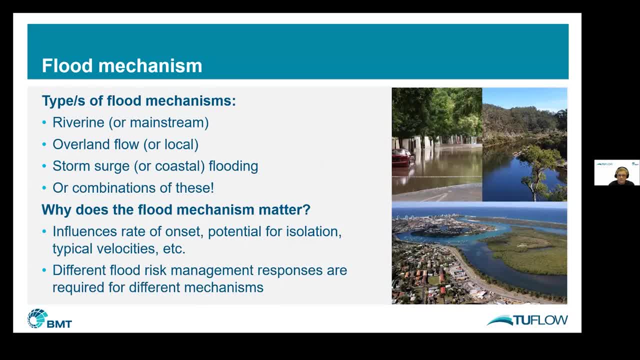 for isolation. you know the flood characteristics, the depth, the velocity, and there's also different flood risk management responses that are required for different mechanisms. so, for example, when we consider over sır, logical solutions to flood risk desenap easily. for, for example, when we consider over-threatening flood risk preparation methods for coming material analysis areas. so firstly, it's important. 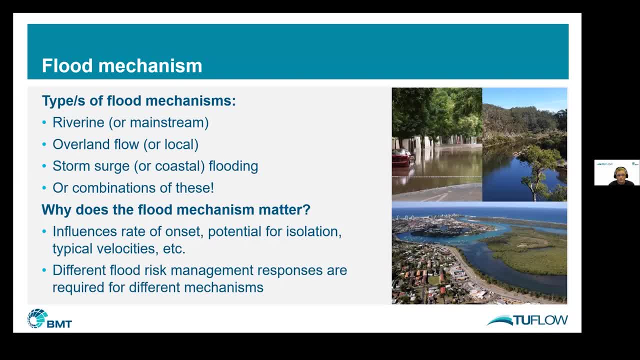 overland flow flooding. we often call that flash flooding, so there's typically a quicker rate of onset. the flood waters recede quicker, so there's often less warning time and less opportunity for evacuation, whereas if you've got a town in the downstream area of catchment and it's affected, 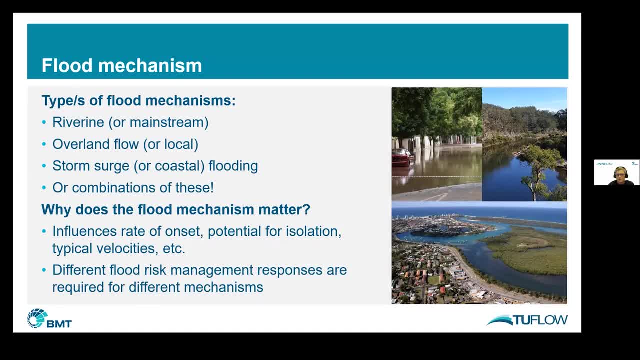 by riverine flooding. there's often greater flood warning systems available. there's often longer time from the start of the rainfall event to when the flooding will impact that town. so you know, we we need to have an understanding of the flood mechanism and really tailor our responses to our 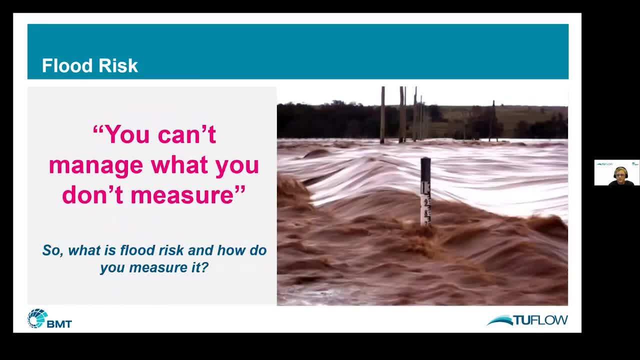 understanding of these mechanisms and, secondly, best practice. flood risk management begins with some sort of foundational understanding of the flood risk to people, to property, so that this can be assessed, communicated and, where possible, mitigated. you but really, what is flood risk and how do we measure it? 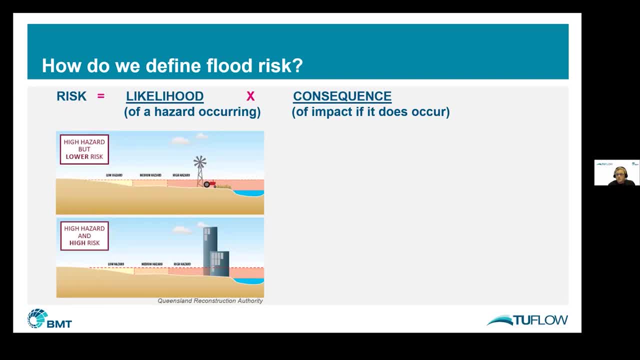 so best practice adopts a flood based, flood risk based approach that defines flood risk as a combination of the likelihood of occurrence of an event and also the consequences or impact if that event occurs. so, in terms of likelihood, best practice would consider a full range of flood events, from your more frequent events to extremely rare events like the probable maximum flood. 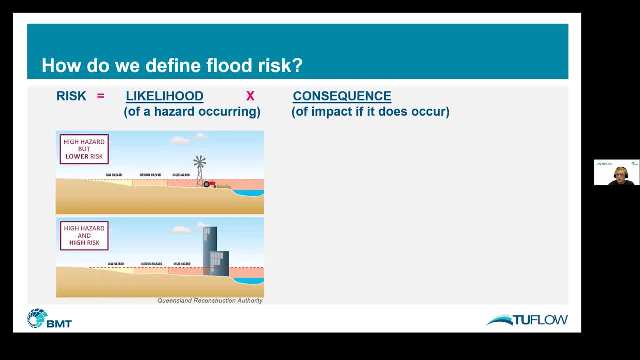 Flood Information and recognizing that there's a range of different consequences and risks, that Flood Information Can vary between events of different magnitudes, and we really want to consider the full extent of the cinq Flood information, Flood Support, ricード estrategias, prominence flood plan, all the way up to the extent of the probable maximum flood flood eligible flood risk. 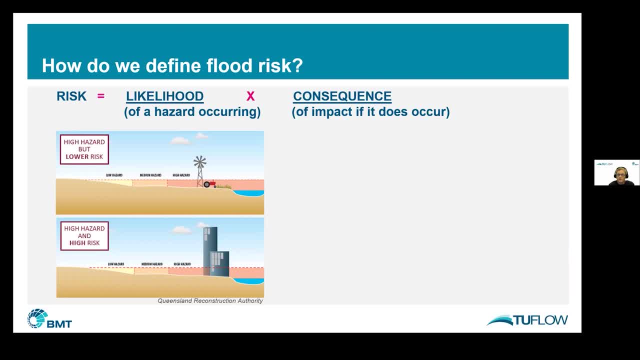 in terms of consequences. risk requires are risk receptor, so someone or something that's impacted by the hazard, and therefore it's important to note Flood дong And therefore it's important to note that there's a difference between flood hazard and flood risk. So you can see on the screen there's two areas: a more rural environment and a more urban environment. 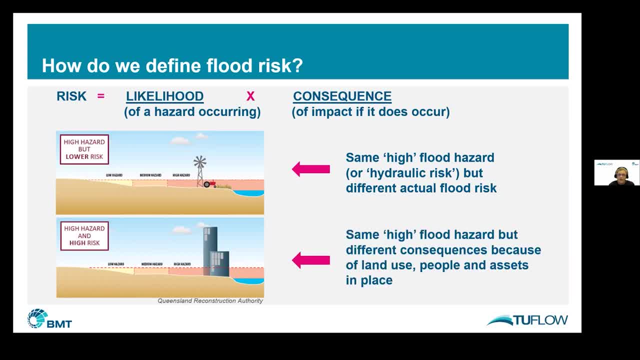 They have the same high flood hazard but different actual flood risk because there's different consequences due to land use, due to people and due to assets in place. So really best practice recognises that flood risk to communities is created by this human interaction with the flooding. 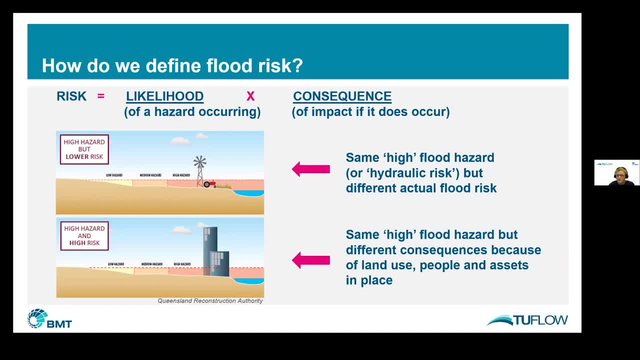 And it's this risk that will vary with the frequency of exposure to the hazard, the severity of the hazard and the vulnerability of the community and its supporting infrastructure. So we really need to have an understanding of this interaction in order to inform our decisions on which treatments to use in managing the flood risk. 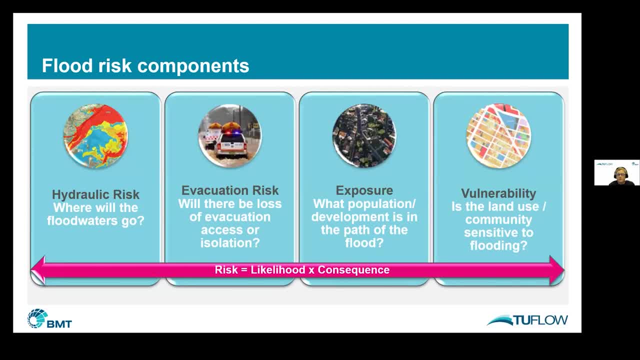 And so we really need to have an understanding of this interaction in order to inform our decisions on which treatments to use in managing the flood risk. And then, in defining flood risk, we need to assess a number of different components that contribute to the risk, not only to define the risk, but also to formulate appropriate management measures. 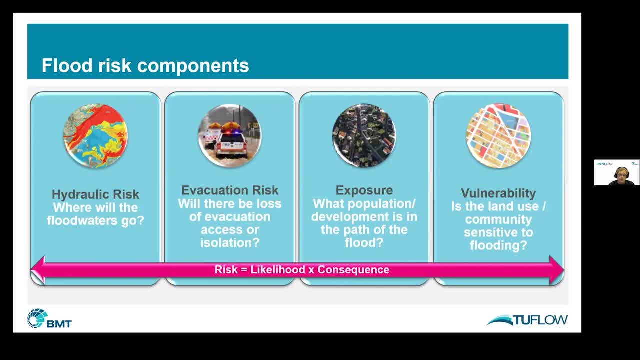 So, firstly, we have the hydraulic risk component. So where will the floodwaters go? You know who's getting wet, How fast is the water moving, Or what's the flow velocity? How deep is the water? What are the flow conveyance characteristics? Is an area in a floodway or a flood storage area? 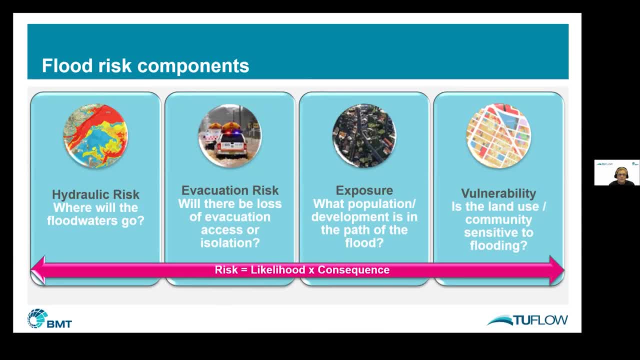 Or where's the flood hazard. And then, secondly, we need to consider the evacuation risk component. And then, secondly, we need to consider the evacuation risk component. So will there be a loss of evacuation access or isolation, So are areas physically surrounded by water? 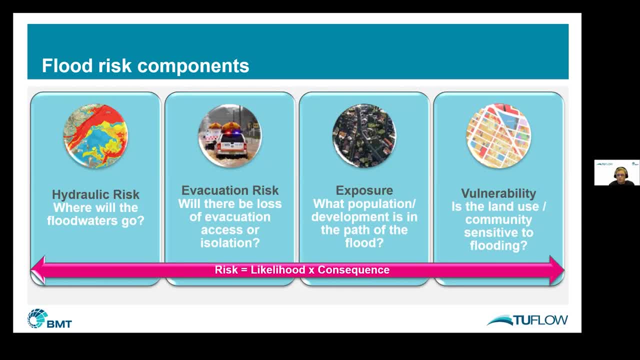 Is there a loss of access and evacuation routes? How quickly will the water, floodwaters scolds? Is there a loss of access to the effect of flooding, health barriers or water刚 Called projects such as Fρεmming or Kees and Niagara, but we are Hurricane. 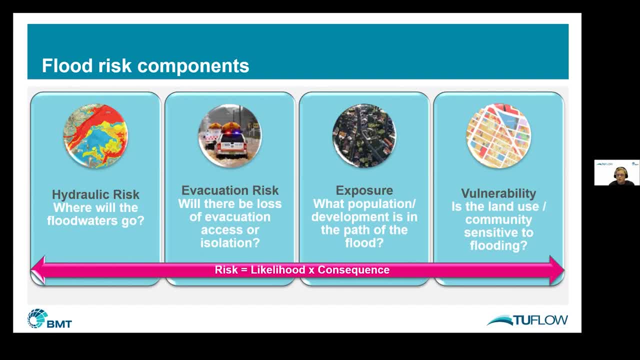 infrastructure. Do we have time between the warnings and the flooding reaching a location to evacuate? Do we have time between the warning and the flooding reaching a location to evacuate? And if we need to evacuate, how? So could that be onion? So can you add a line? or how do you indicate a cooling behaviour or going to thatû? 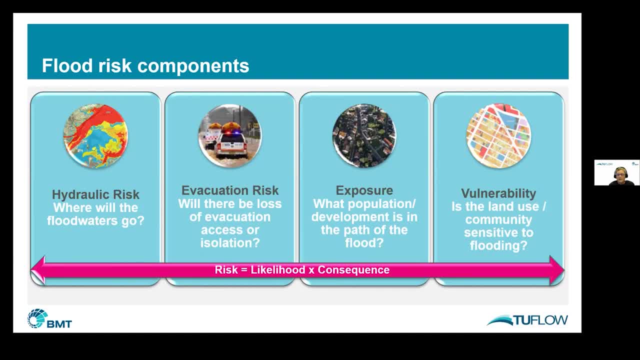 Yes, how will we go? will we go on foot or by vehicle, and is it safe to do so? we also have the exposure. so what population or development is in the path of a flood? how many people and properties will be impacted? will there be failing structures? 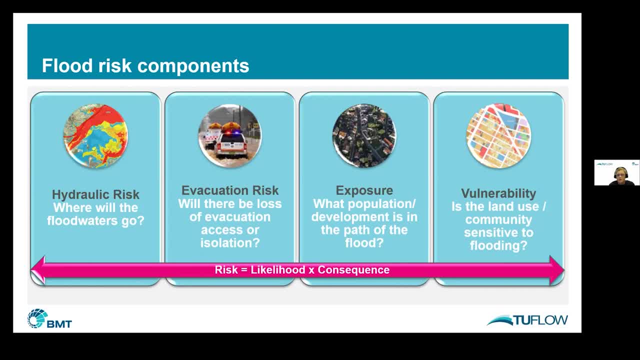 or infrastructure? will there be a loss of service and amenity? water power, you know, food supplies, medical assistance and, finally, what's the vulnerability of the community? is the community resilient and tolerant to flooding, or are there vulnerable land uses or people? so where are vulnerable uses located? are there hospitals and child care centers? 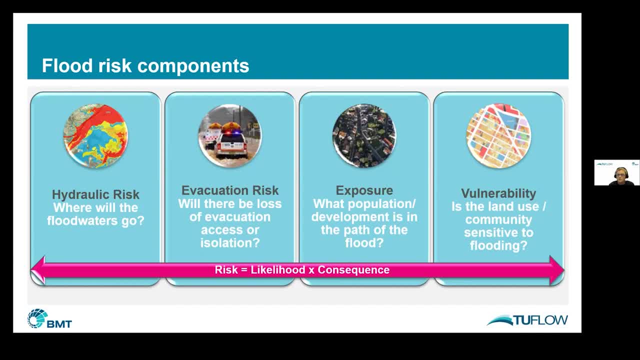 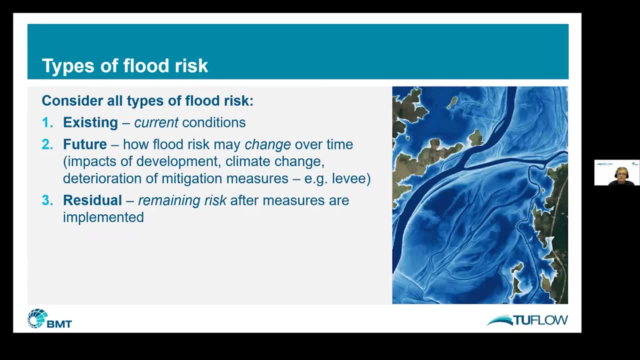 are there aged care facilities? so all of these components need to be considered to have a clear picture of the flood risk. and i suppose, lastly, there's different types of flood risk. so there's really three different types of flood risk that we consider. so, firstly, we have the existing flood risk, so this is based 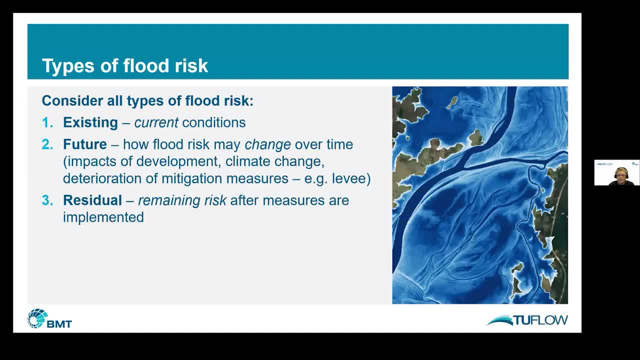 on the current conditions. the current catchment floodplain, climate development conditions and knowing the existing flood risk to the community provides the basis for making informed decisions on whether the risk is tolerable, whether to treat the risk and, if so, how do we do it. secondly, we have the future flood risk, so how will the flood 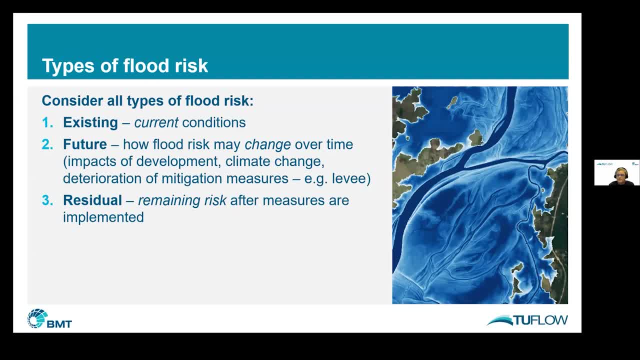 risk change over time. you know we need to consider the future catchment climate development scenarios and then i suppose knowledge of the future flood risk can feed into strategic land use planning, for example, so we can inform decisions on where and how to develop the floodplain to ensure that. 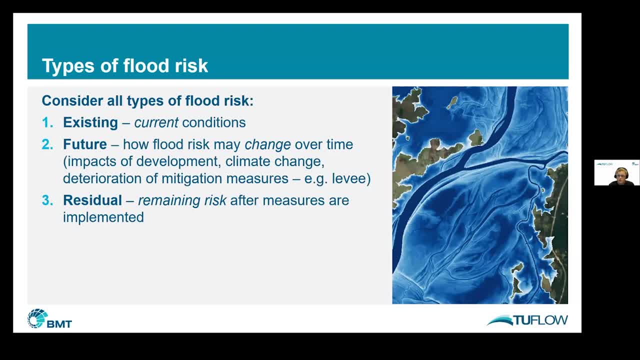 the risk to new development and its occupants are acceptable, or where not to develop, so where new development may impact flood behavior and increase the risk to existing development. or are there areas where the flood hazard's too high and we just can't manage the risk, so we shouldn't put. 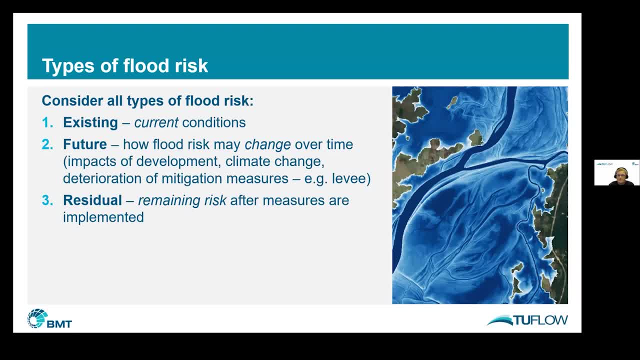 more people there, and so that's particularly true of additional factor. finally, there's the residual risk. so this is the risk that remains once measures are implemented, and so, unless you're going to be designing or tailoring your flood risk management plan to the probable maximum flood, then- and you're also assuming that works won't fail if you- 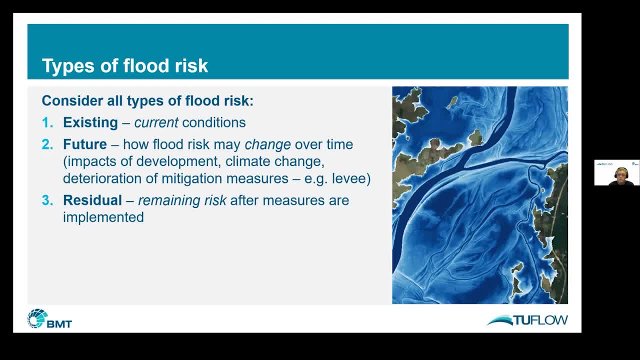 do implement them, then there'll always be a flood risk to the community and this risk will remain, you know for for that community and we need to really look at emergency management and recovery planning, and this can be supported by systems and infrastructure to reduce the residual flood risk. 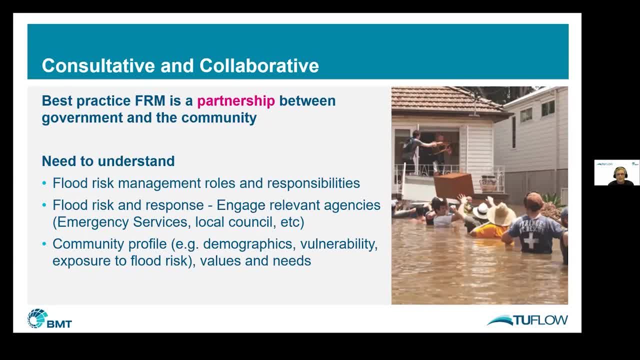 so now we've talked about defining the flood risk and different mechanisms, and then i suppose there's really a number of key components of flood risk management best practice that we really talk about in terms of our approach. so best practice- flood risk management- should be consultative and collaborative. 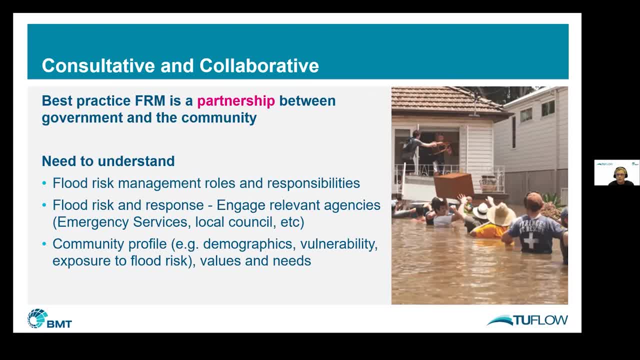 where possible, it should be a partnership between the government and the community, using a range of measures to reduce the risk to the community. so decisions on managing the flood risk should be made in consultation with stakeholders in the community that are actually impacted by the floods, and in doing so, this helps. 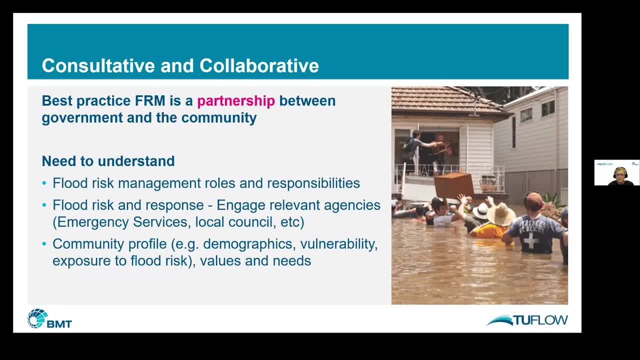 flood risk managers to understand the roles and responsibilities of those involved with flood risk management, also what the flood risk knowledge and response is of the community. so we really should always recognize the value of local knowledge and those with boots on the ground who experience and respond to the floods, and also we need to have an understanding of the community. 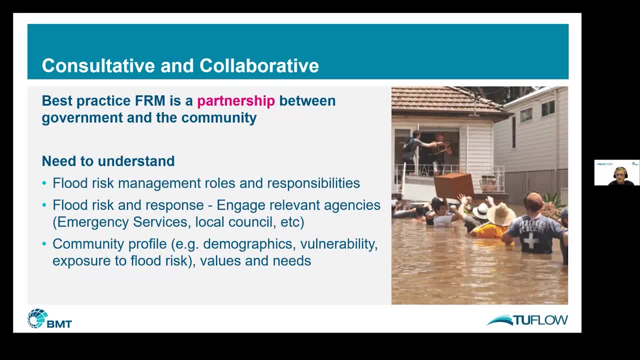 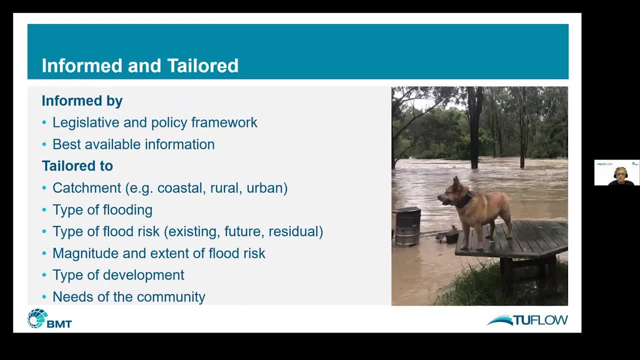 profile. so what's the vulnerability of the community, what do they value, what are their ideas and what are their needs? best practice flood risk management is also informed and tailored, so we should make informed decisions within the context of the legislative and policy framework and using the best information available at the time that we make the decisions. best practice flood risk. 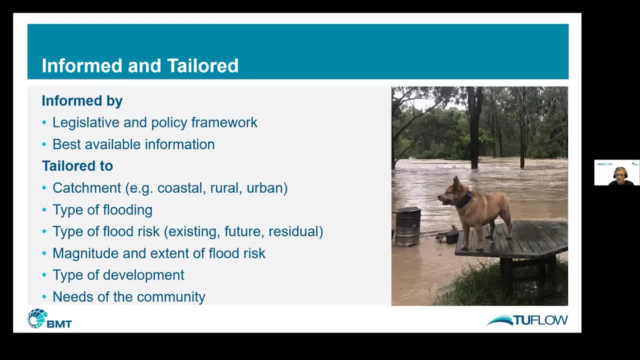 management should be tailored so it's tailored to the needs of the study area, considering the catchment, the type of flooding, the type of flood risk- you know, the magnitude and extent of the flood risk- and the types of development that are present or that may be there in the future. 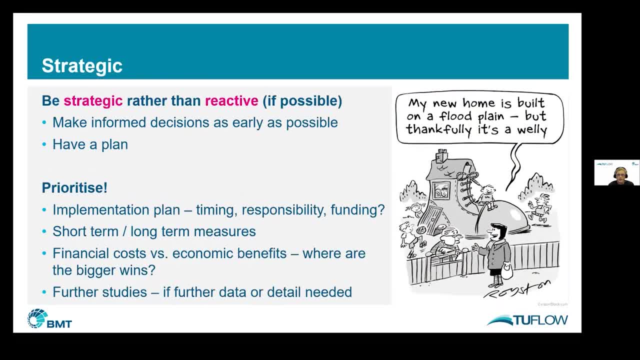 and also the needs of the community. an important component is also that best practice. flood risk management is strategic. so we employ a strategic approach rather than a reactive approach. make informed decisions on development within the floodplain by considering the flood risk as early as possible. i mean in. 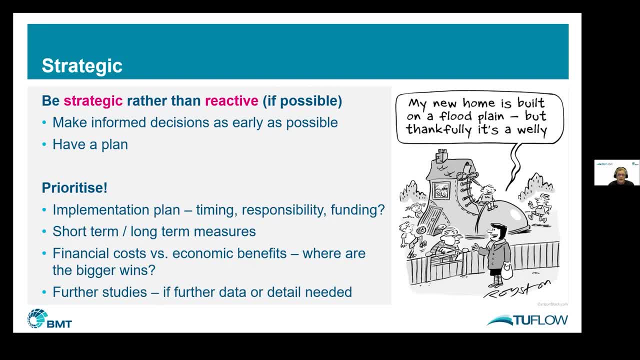 doing so we could create risk responsive settlement, land use policy and zoning. and also, it's always better to have a plan than no plan. and in terms of prioritizing, we should prioritize flood risk management, considering the scale and of the existing risk to the community and the scale of the potential growth in risk, for example, new 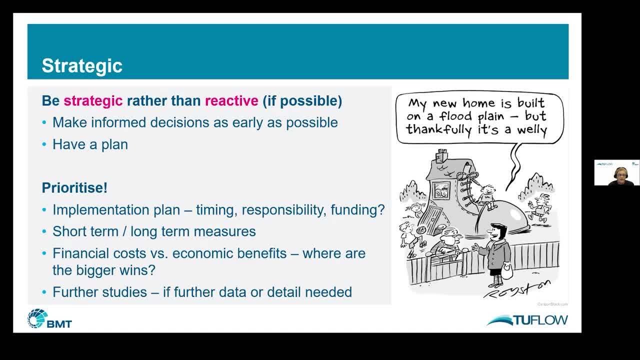 development within the floodplain. we need to have an implementation plan, so what are our time frames, who's responsible and where is it going to be funded from, and then we can think about what can be done in the short term and what can be flagged for longer term implementation. 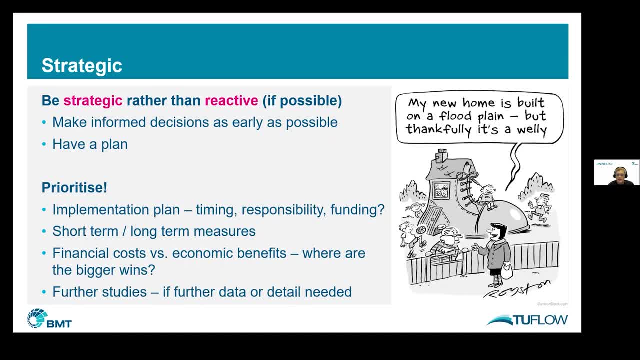 in terms of financial costs, think about where there are the biggest gains in terms of economic benefits and then, I suppose, at the end, prioritizing what further studies and outputs are needed. so, for example, gathering further data in areas of greatest development pressure or future growth areas, or, if you want, 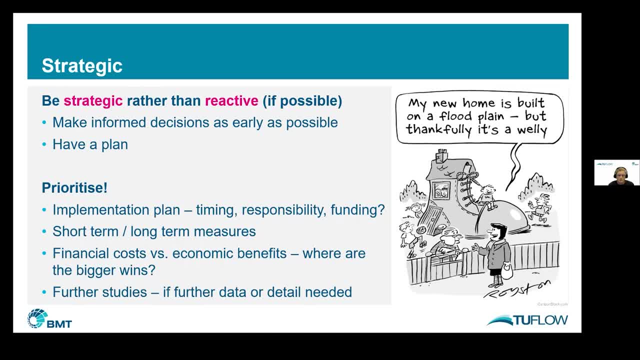 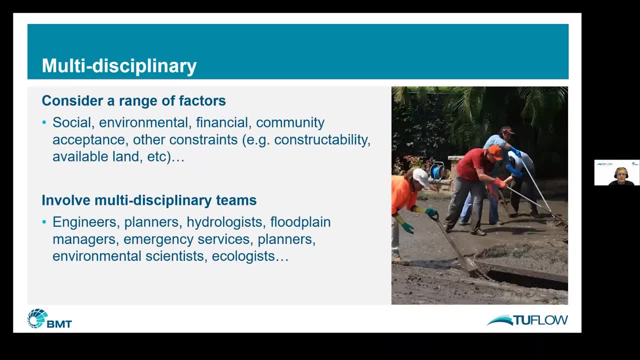 to consider climate change factors in further detail. Our best practice flood risk management is multidisciplinary, so we need to consider a range of factors: social, environmental, community acceptance. are there other constraints about constructability? are there land constraints? do we have available land to build these works? and ideally we involve multidisciplinary teams. 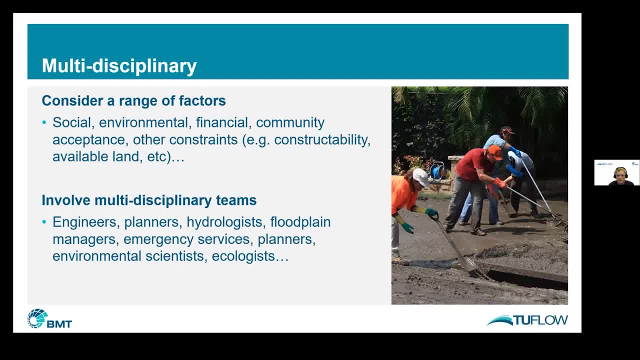 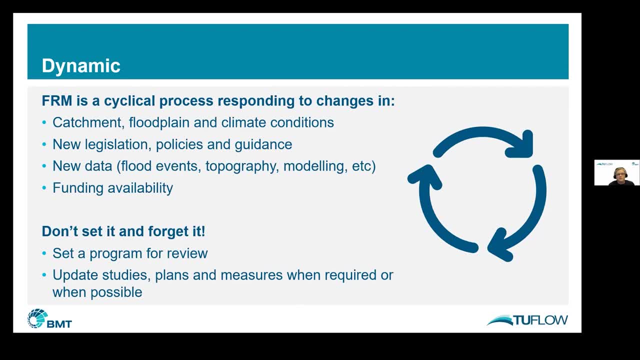 so those specialists that have the greatest knowledge in their areas of practice. And, finally, best practice. flood risk management is dynamic. you know flood risk management plans are living documents, so it's really a cyclical process that we can adopt to respond to changes in catchment, floodplain and climate conditions. or 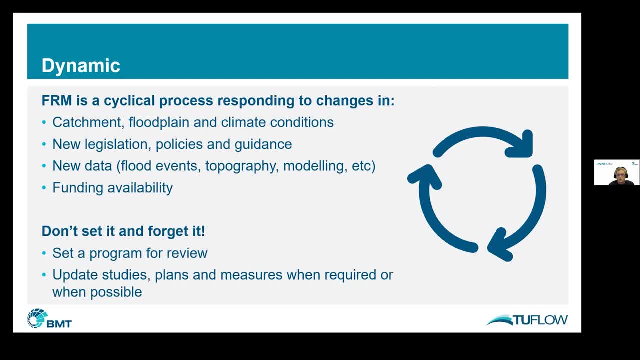 changes in policies and legislation. if new data becomes available- you know terrain data, new modeling outputs- we can consider that we can update plans to incorporate these and also there might be new funding availability. that means that implementing some of the measures because of the climate change factors are dynamic. you know flood risk management plans are living documents. 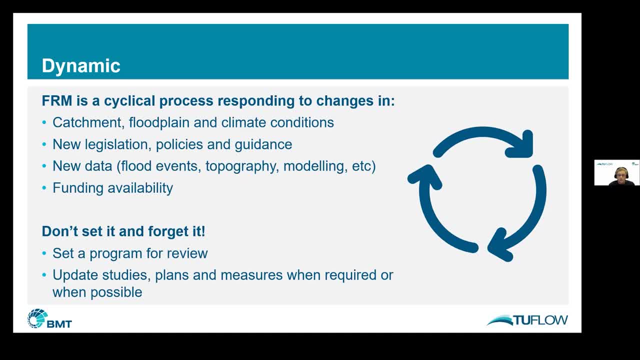 that means that implementing some of the measures because of the climate change factors are dynamic. you know, flood risk management plans are living documents more feasible. and finally, don't set it and forget it. so you know you get to the end of a study or a plan, give yourself a pat on the back, you've written the report and it gets put on a shelf and gathers dust. 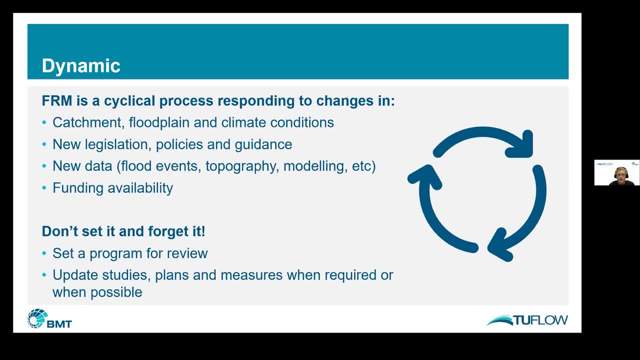 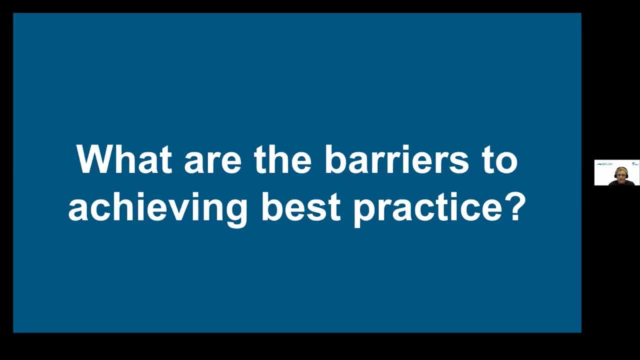 you know that's not best practice- set a program for review and update studies, plans and measures when required or when possible, But I suppose is what I've presented- an idealized view of flood risk management. can- I suppose is what I've presented an idealized view of flood risk management, can we simply create a best practice checklist and tick all the boxes as we go or, in reality, are there barriers to achieving this best practice? 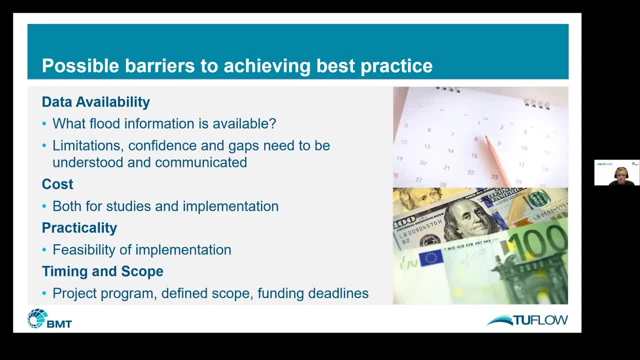 From our experience, we can be bound by barriers and constraints in the process that are imposed by data availability, cost practicality, timing, project scope and funding, And that's really where an understanding of the fundamentals or ideals of best practice principles is needed to guide us in the right direction. 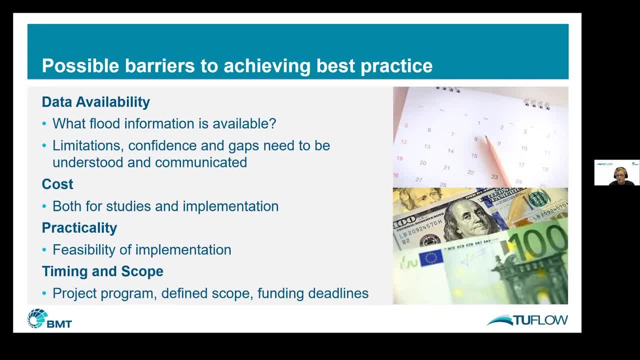 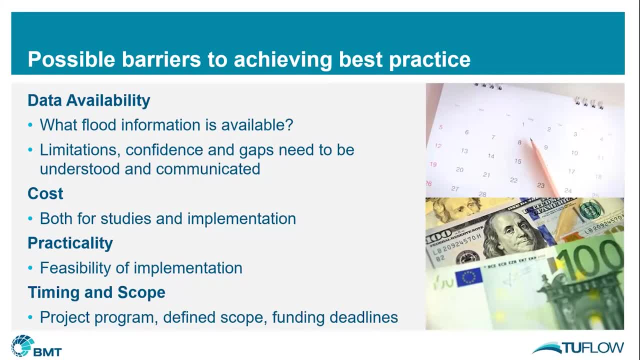 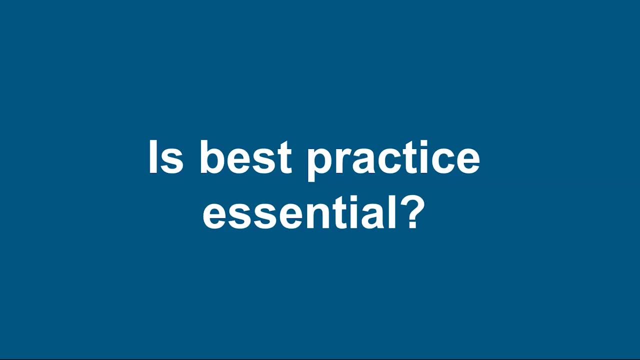 And that's really where an understanding of the fundamentals or ideals of best practice principles is needed to guide us on the best possible possible within the confines of reality. I'll now pass over to Carrie to continue our presentation. Thanks, Jackie. So Jackie identified some barriers to best practice, but I guess the big question is: is it essential? is that something we have to do? 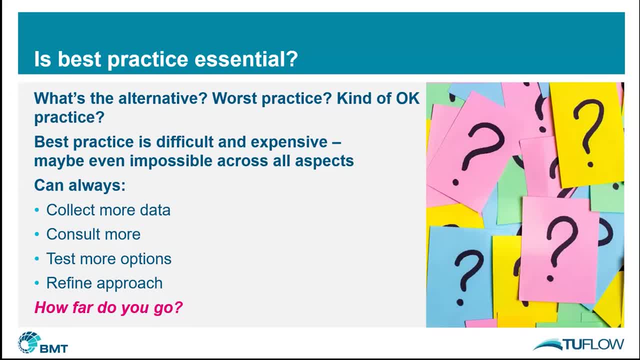 So I guess, if we're not doing best practice, what's the alternative? surely we want best practice, we don't want to do worse practice, kind of okay practice, but Those barriers are in place. best practice is really difficult and really expensive and there actually isn't the finish line. you can always get more data. 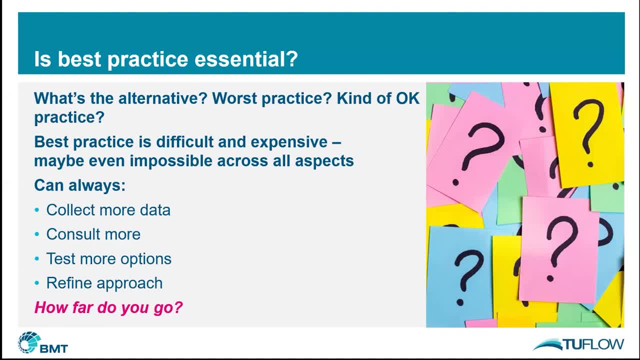 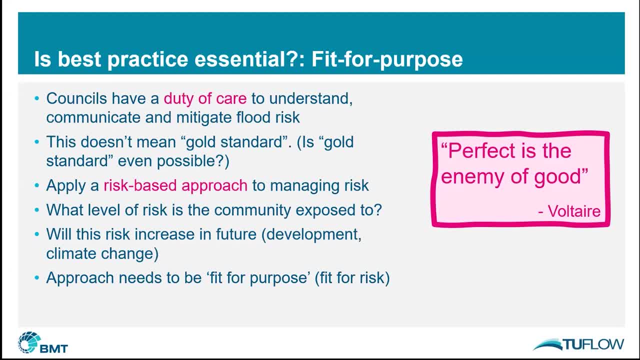 And then you know sod's luck: there'll be a flood in the middle of the day. And then you know sod's luck, there'll be a flood in the middle of the day. But also thinking about where that will change in the future, if there are some locations that are more 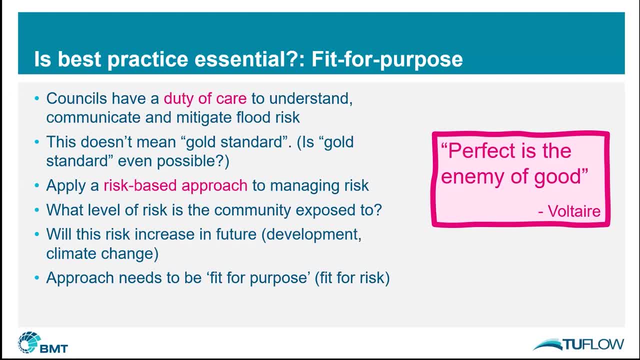 vulnerable to the impacts of climate change or changing conditions due to development, And you need to think through all these things and decide a fit for purpose approach. and decide a fit for purpose approach. Now we're going to come back to this poll question. 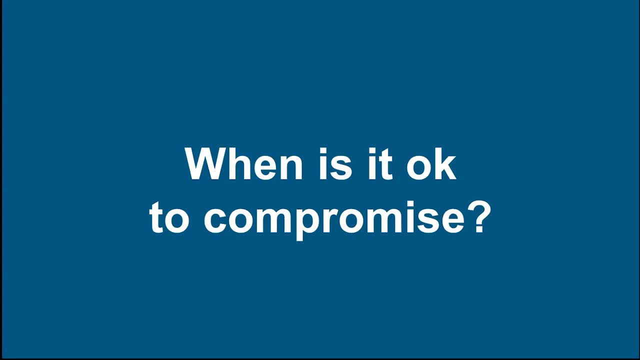 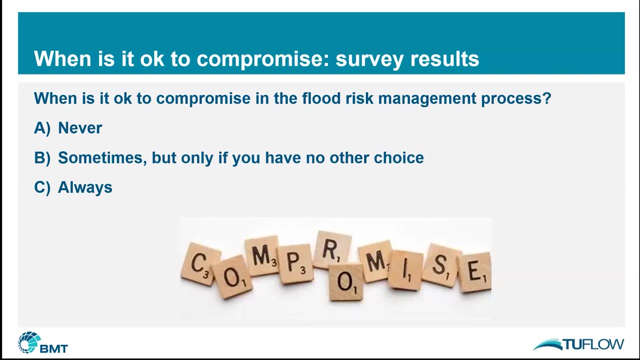 that we asked right at the study, so I hope everyone's had a go at answering that: When is it okay to compromise in the flood risk management process? So we asked: never, sometimes, but only if you absolutely have to, under duress or always, and that the answers that Trevor gave. 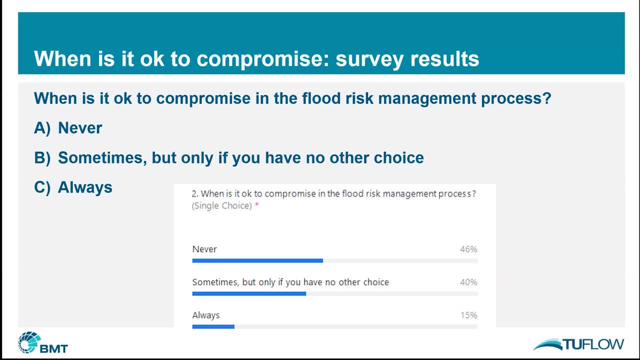 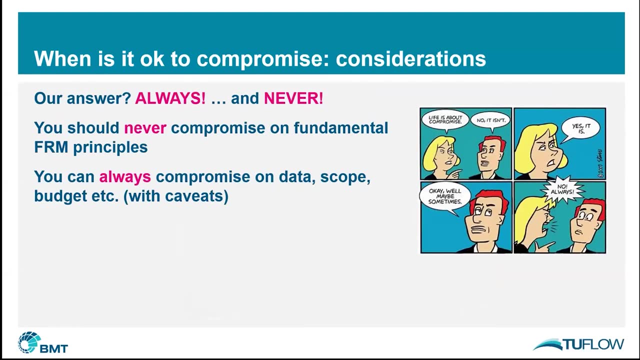 back. they're pretty evenly split between yes or never, and always so 46 and 40 percent. so very different answers not many people went for. sometimes you're all pretty certain in your answers and then quite split down the middle. so our solution is both. you're actually both right. 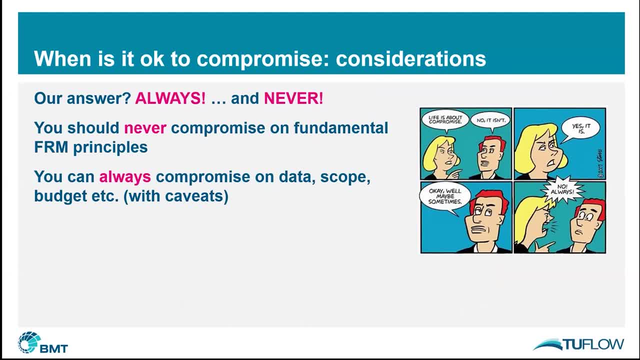 in our view, our answer is always and never. so I'll explain that a bit further. we feel that you should never compromise on the fundamental flood risk management principles. so those principles that Jackie went through in terms of your approach being informed and tailored strategic, consultative dynamic, those are things which you should really hold to your heart and stay true to through the 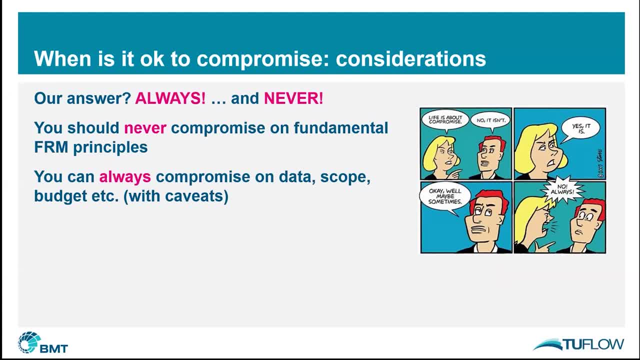 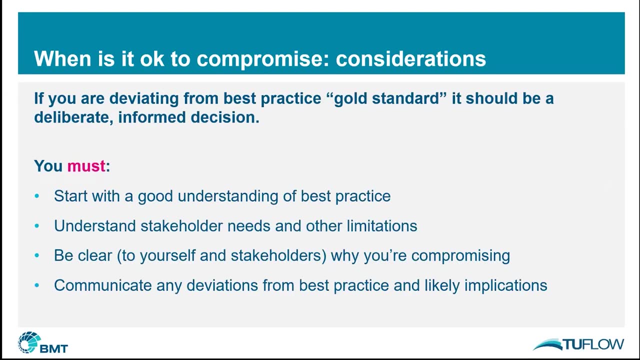 process. but you can always compromise on the process, on the data, the scope, the budget. but there are caveats and do not proceed on this without listening to the caveats. first, make sure you listen to the rest of the presentation. so if you're going to deviate from this best practice, this gold standard approach, you need. 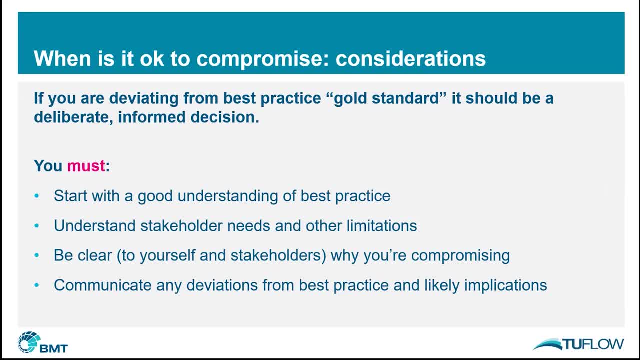 to make sure that it's deliberate and informed, that you know what you're doing and you're choosing to make that decision. and that means you start with a good understanding of what good looks like, what is best practice, and then you start with a good understanding of what good looks like. 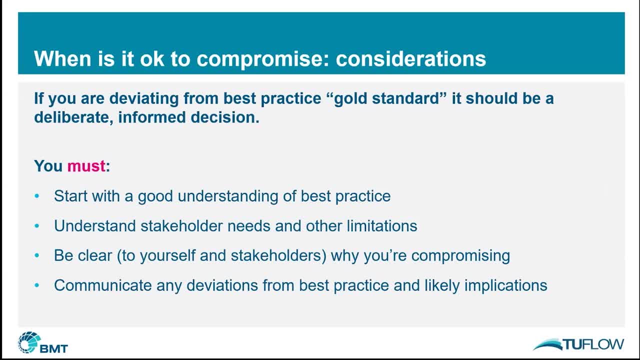 what is that gold standard? and then understand the constraints you've got, understand your stakeholder needs, any limitations on the study, and then be really clear, both to yourself why you're making the decision, but also to stakeholders, your clients, the council, to whoever is involved in the study, on why you're choosing to compromise, why you're not achieving gold. 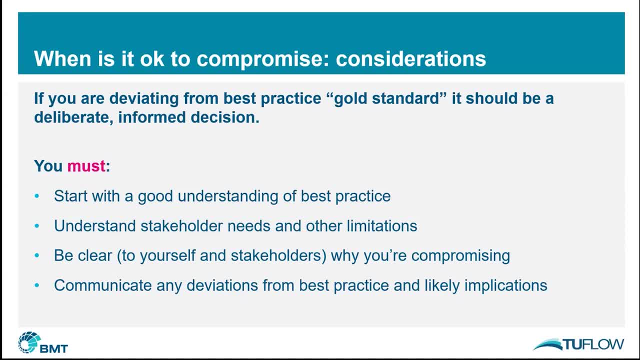 standard in this case. so be clear in your understanding and then make sure you communicate it, not just why you're doing it, but what you're doing and what you're doing and what you're not doing, and depending on how yourителей are doing and what the impact you'll expect, the 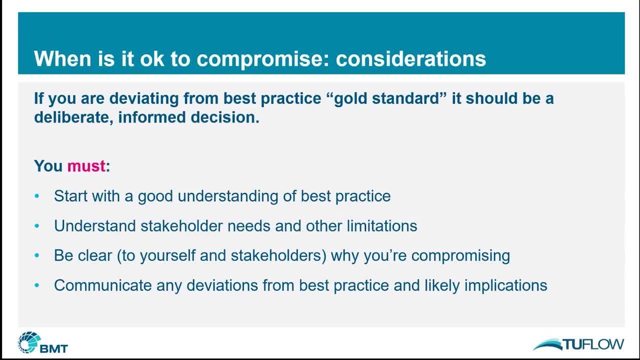 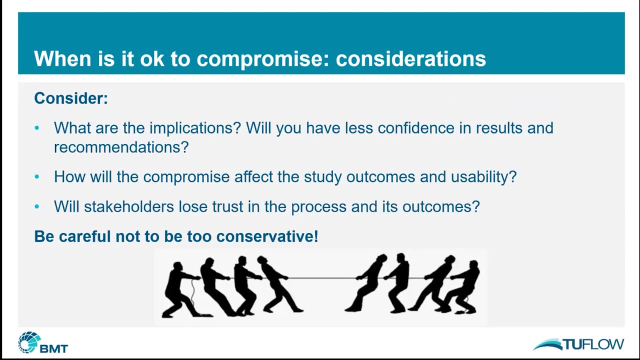 implications will be how it will impact your study, and that can be hard to know at the start of a project, but you can make your best guess and you can go back and you can refine it as you get some more information throughout the project. some of the things, though, you should consider. what are? 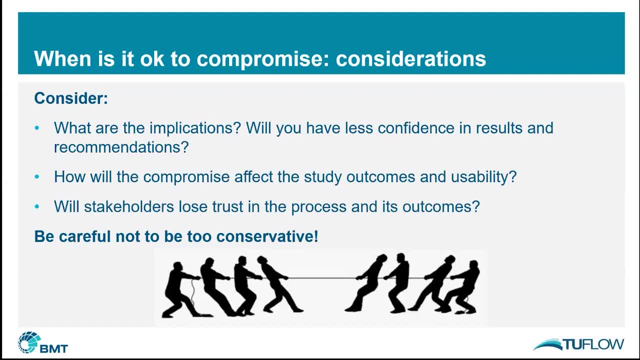 those implications? if you choose to compromise, if you're using less than perfect data, if you're using a smaller budget than you'd like, if you're rushing a study more than you want to, if your as you'd like it to be, what are the implications of doing that? Does it mean that there'll be less? 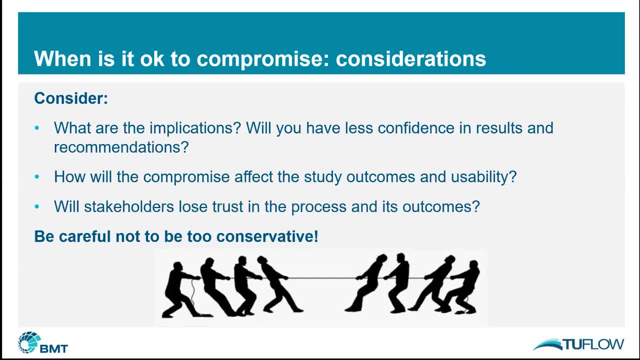 confidence in your end product, in the process and in the results and recommendations, And how will that affect how the study can be used? Will it meet its required purpose? If you've understood why the study was needed in the first place, you can now come back and say, okay, does. 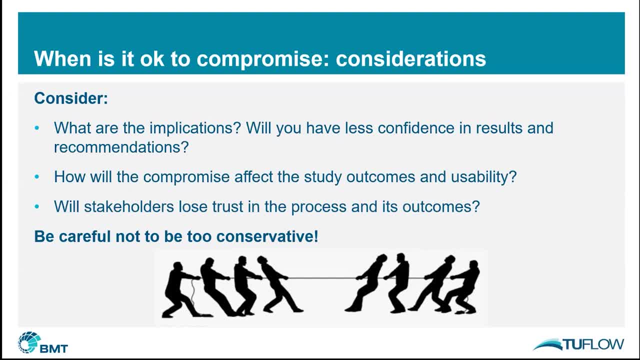 our fit for purpose approach, deliver an outcome that meets those original identified needs, And here's a big one. Will the stakeholders lose trust If you do something that's too rushed and people feel it's a shoddy job? they're not going to listen to your recommendations. 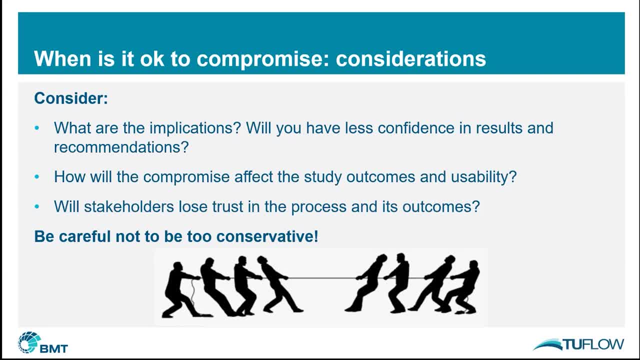 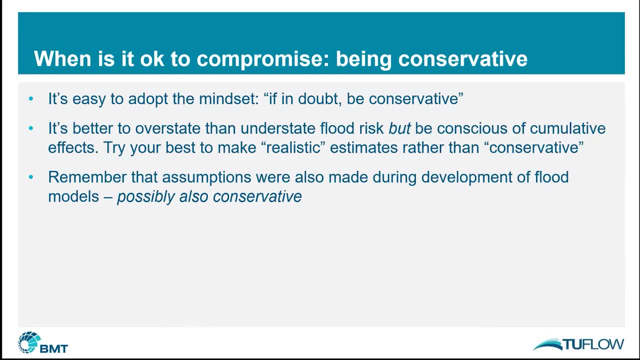 They won't have faith that you've done the right thing. And finally, I'd urge you to not be too conservative. So this is, I think, something that I got really stuck on early in my career was being conservative. You don't want, you think you don't want- any flood risks. So if there's 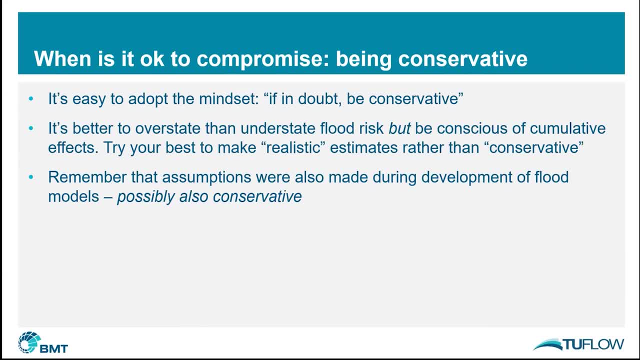 any chance that you're going to be too conservative. you don't want to be too conservative. If there's any chance that it might be one way or another, choose the conservative option. if in doubt, be conservative, But if you do that for every single decision. 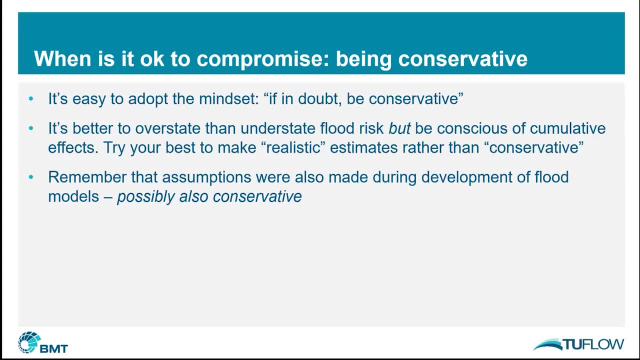 you run this risk of kind of cumulative decisions: more conservative, more conservative, more conservative- and they build up. So instead it's better to try and make realistic estimates. understand your uncertainty, but aim more towards realistic, knowing ultimately that the way you respond to your assessment can be a little bit more conservative. And remember: 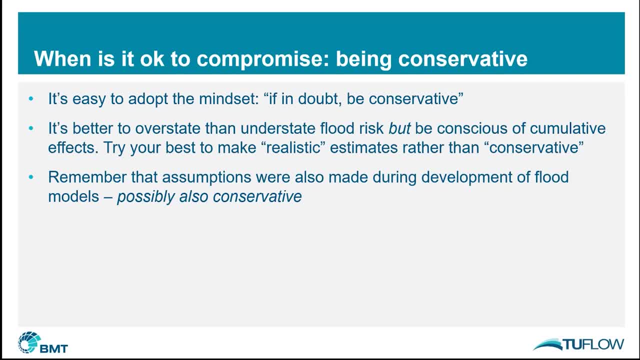 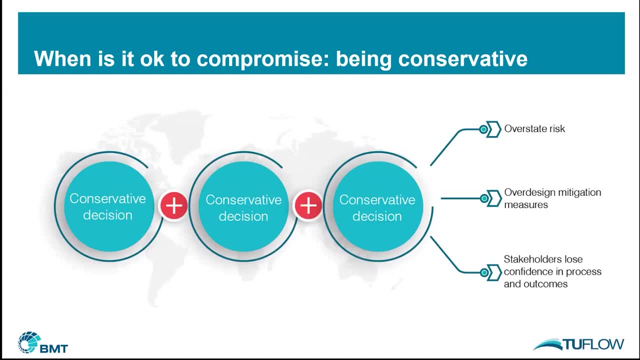 of course, that the flood model inputs to the study. that was also full of assumptions. They might have been conservative too, So here's a little schematic. If you add up those conservative decisions, some of the big outcomes are: of course you end up overstating the risk. 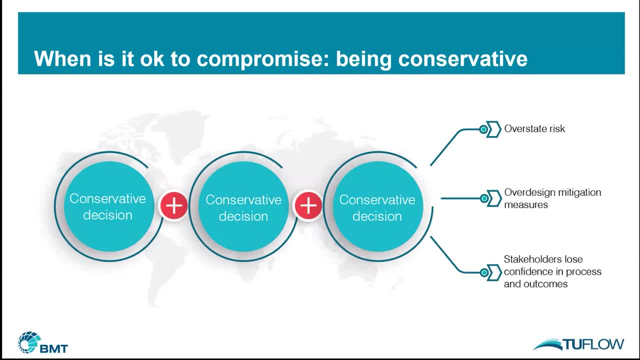 possibly by a long way, And from there you then over-design your mitigation measures. That might be more flood warning infrastructure than you need, or it might be a higher bridge. It could be a very expensive decision to be over-conservative, And once again stakeholders can lose confidence. 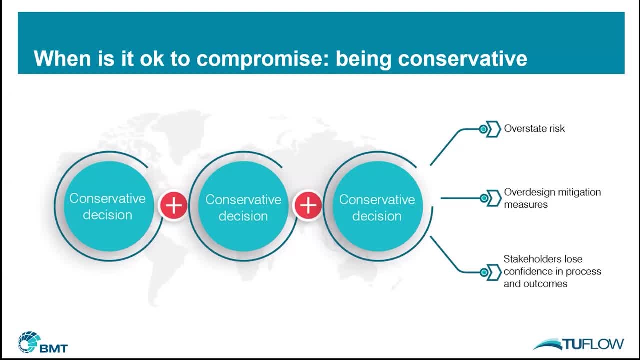 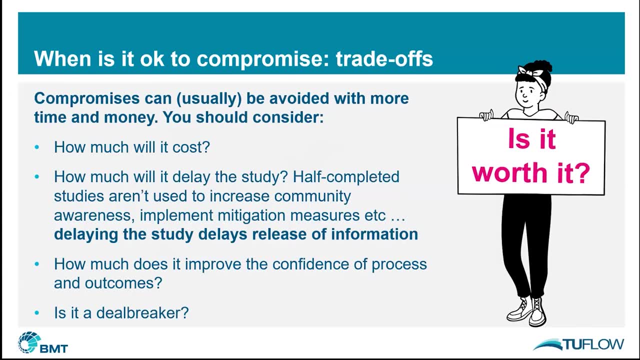 in the process and the outcomes They say. that doesn't reflect our reality. This isn't the scale of the risk in our catchment, So be really careful on that issue, Excuse me. And if you are going to compromise, be conscious that there are trade-offs, So you can always buy your way out of compromises. 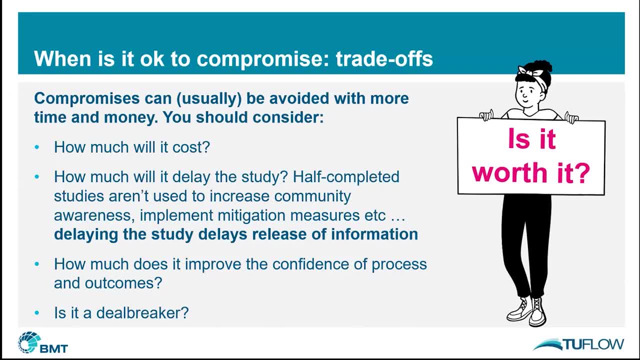 If you have enough money and time, you can get better data, You can increase your scope, You can do all these things. but there are trade-offs. So think about how much does it cost. What's the financial outlay to reduce this compromise? And here's a big one. 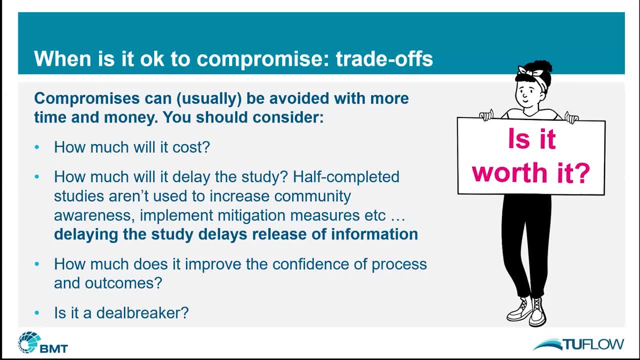 that I think we don't spend enough time thinking about How will it delay the study. So if you want to go back and refine your data, refine your process. you know, keep getting stuck in consultation lips that might delay your study over an entire storm season During that time, 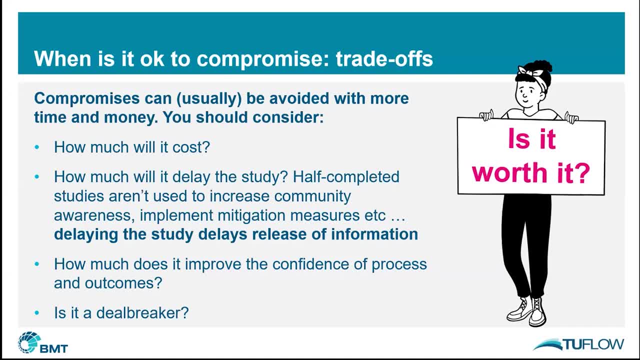 we haven't got flood information out to the community. They don't know that they're in a flood risk area. People might be buying properties without having good flood information. There might be infrastructure designed without this information, So be aware that when you're. 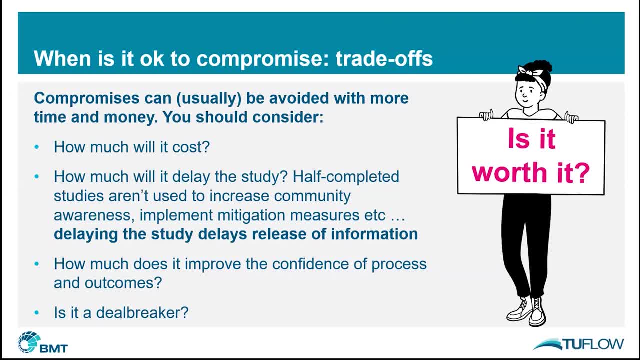 delaying to improve, to reduce your compromise, you're delaying the release of information and delaying the start of action, And I think that's a really big thing to keep in mind Once again, be thinking about how it improves the confidence of the process. 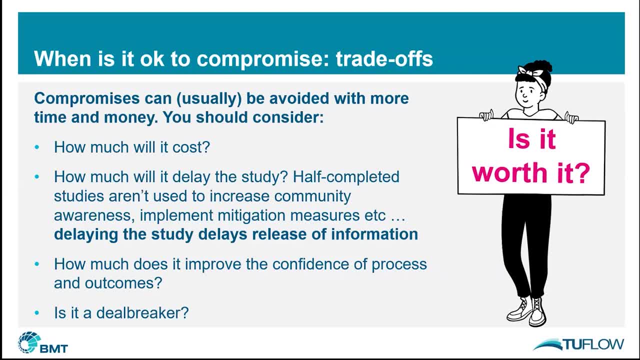 and the outcomes, And then this one will vary significantly from study to study. Is it a deal breaker? Sometimes this could be political. It could be relevant to the geography of your area, Who knows? But you need to figure that out for your study. Is there anything that? 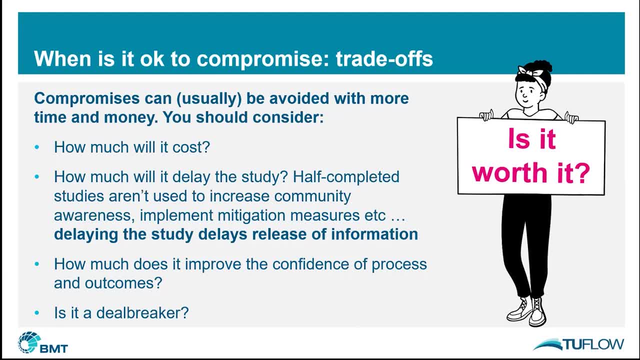 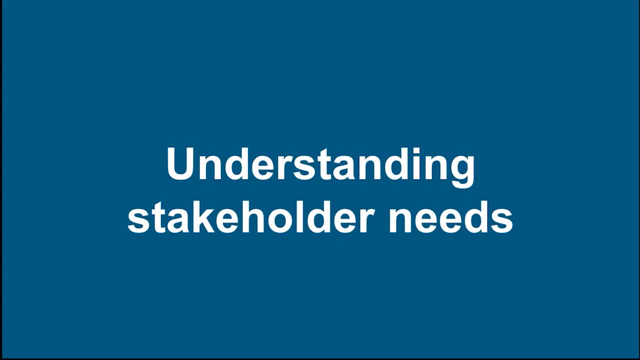 cannot be compromised in your study, that you have to keep in place. So I've talked a lot about reducing confidence in stakeholders, So I do think it's worthwhile spending a bit of time understanding stakeholder needs, And this is really a topic that can be a standalone session. 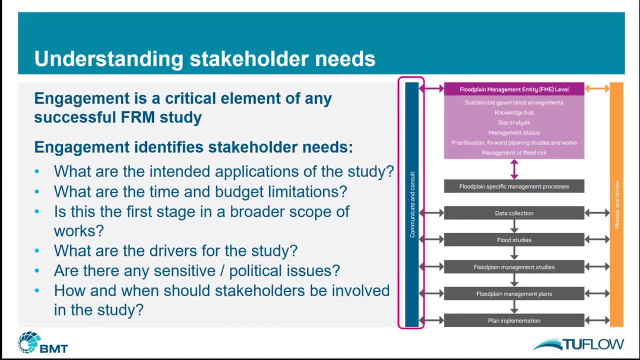 Engagement and consultation is a very big area and something which gets overlooked a bit sometimes in some of these studies. But if you see this little diagram to the right, this is from the National Floodplain Guidance in Australia called Handbook 7. And that, the blue vertical column, 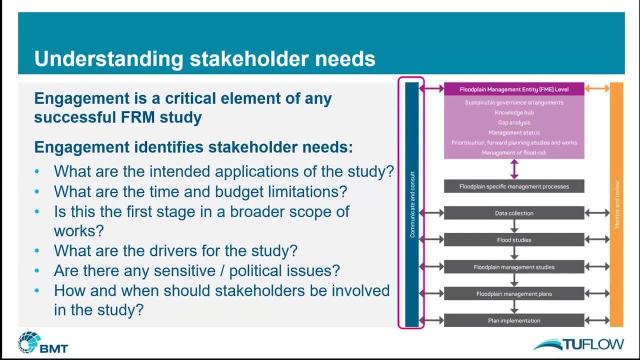 there it says communicate and consult And this is really important because it goes across every single stage of the flood risk management process. So they really emphasise how important it is to do all the way through And it has lots of benefits. You can understand what the applications are for the study. 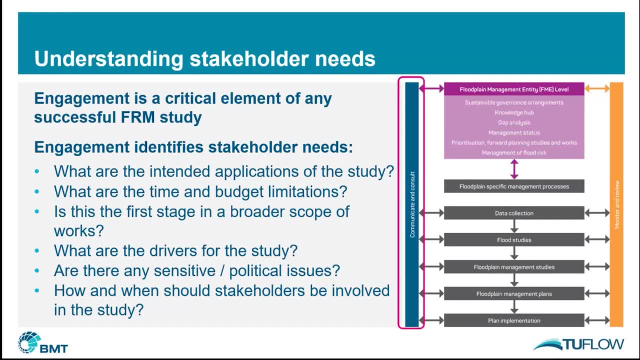 how it's going to be used, any time and budget limitations, Understanding where it fits in terms of a broader scheme of studies. Are there studies that have gone before it that inform it, Or will it be used for subsequent studies? You need to know where this sort of fits. 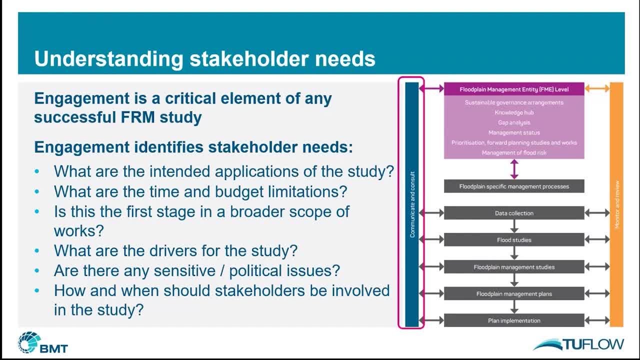 Why was the study commissioned in the first place? Is there anything sensitive or political in your catchment that you need to be aware of, And how will you consult during the process? How should you consult stakeholders and when? In what capacity Do they want to simply be informed? 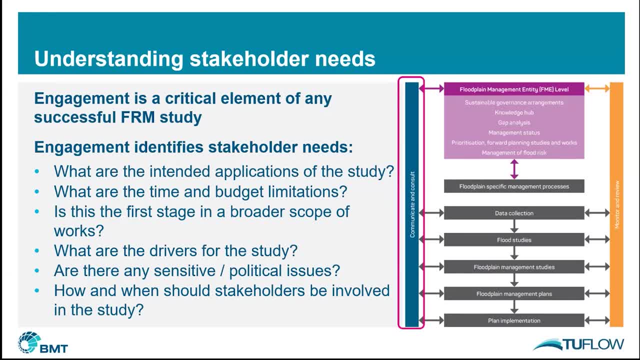 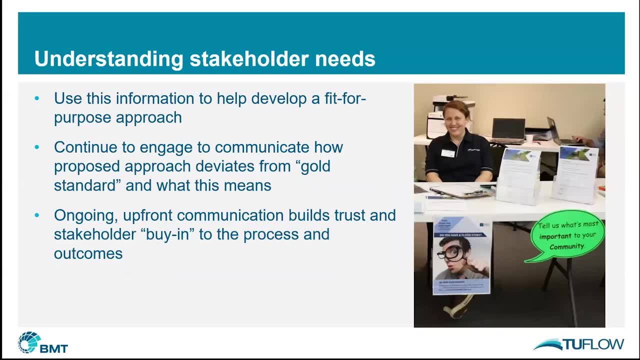 Do they want to be actively engaged in the process. Think about all these things up front And once you have a good understanding, you can use this to help develop this fit for purpose approach that you're going to apply, And then, throughout the the study, you can continue to go back to the stakeholders to communicate how you've decided. 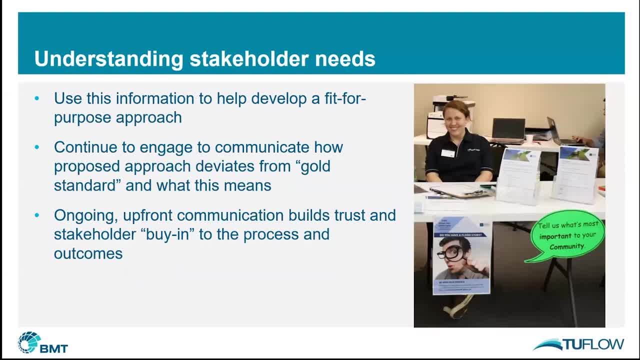 to deviate from this gold standard and what it means. And by doing this, by engaging the stakeholders correctly all the way, through treating them as a trusted partner, you build that trust and the stakeholder buy-in and they're more likely to accept the outcomes. 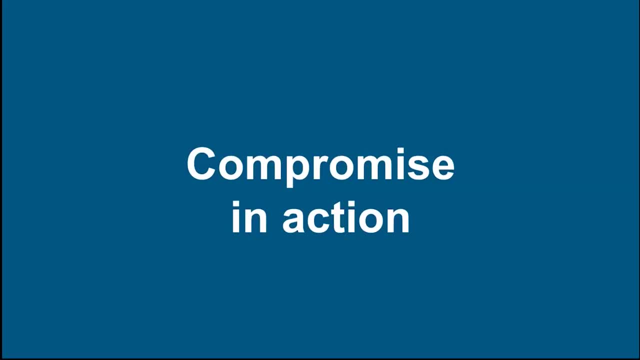 and your recommendations. So I've got just a couple of examples here to wrap up, and I think we've gone a little bit faster than we expected, but that just means more time for questions. So to start with, I'm going to use a really simple example that a lot of people who've done 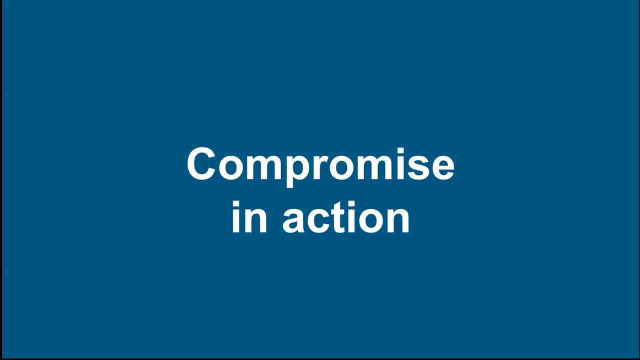 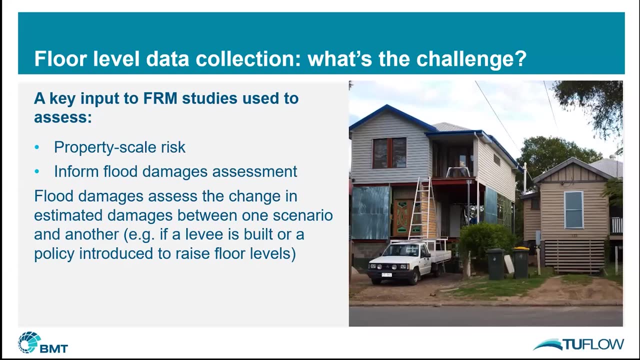 a flood risk management study would have been part of, and that's floor-level data collection. So floor-level data is a really big input to a flood risk management study and it can be used for two main things. One is a property scale risk assessment, so understanding what the risk is. 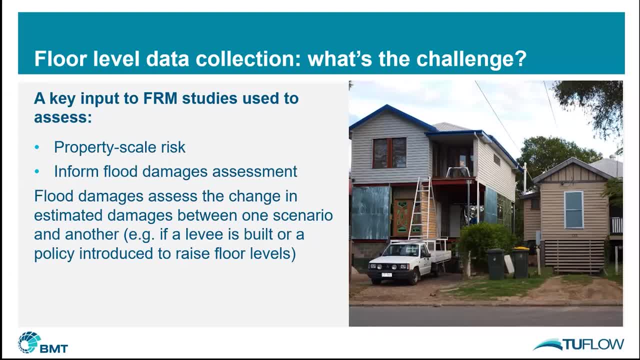 at an individual property site at house X, what kind of levels and hazards and velocities and risk rating So they have, but also to inform flood damages assessments. So these are the assessments we make in terms of base case scenario, the existing conditions And sorry, let's jump forward. 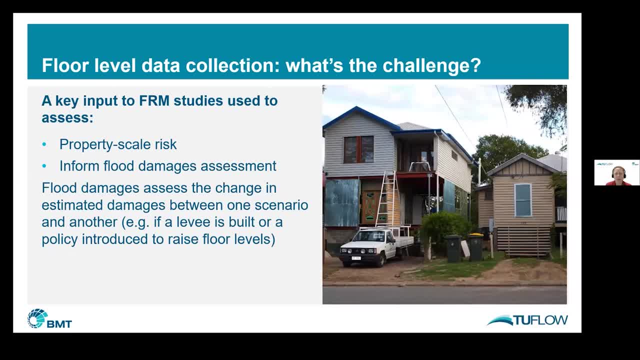 But also in developed scenarios, so we can compare and we can say: okay, how much do we expect the flood damages will change if we introduce some scenario that modifies the flood behavior or a policy to raise floor levels, something like that. So we need this floor-level data of the properties that are in the catchment to inform these types of. 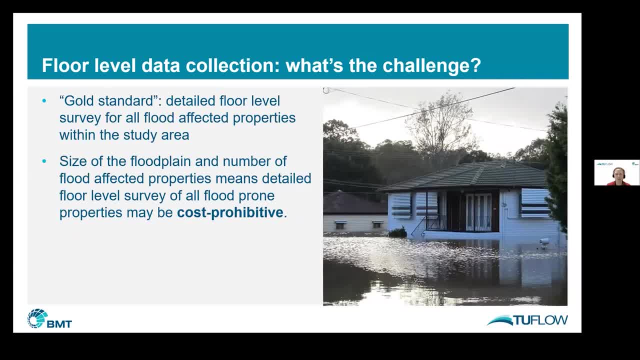 assessments. And to do this by the gold standard approach means that we go out with a surveyor to every single property in the flood plan. that means the entire probable maximum flood extent and we collect detailed floor-level survey, do a building footprint, we understand the ground level. 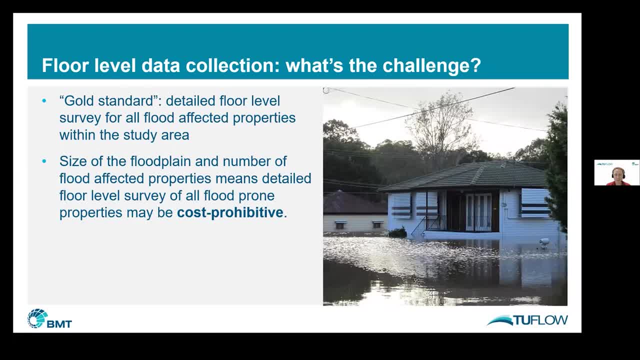 to the nth degree and the floor level, And I can tell you what. I've got quotes for this in the past and it is super expensive to the point where it's really cost prohibitive, except for the smallest areas. It's great data, very reliable, but very expensive. 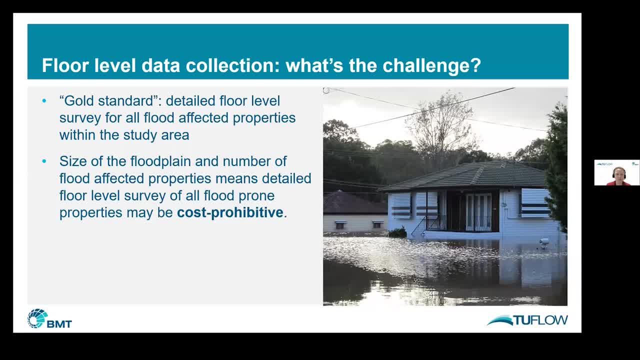 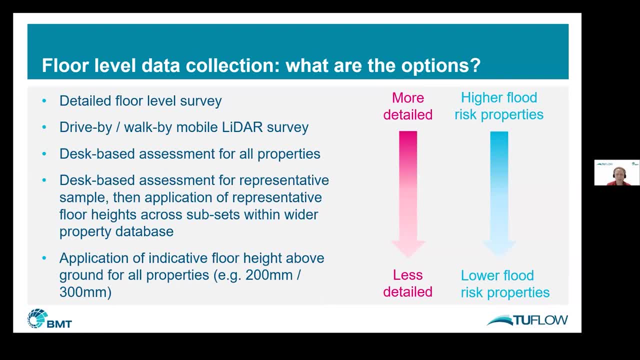 It's time consuming too, so it can delay a study. So there are options that you don't have to do that. That's the absolute gold plated, And so I've got a little list here which is going from more detailed at the top to less detailed, but 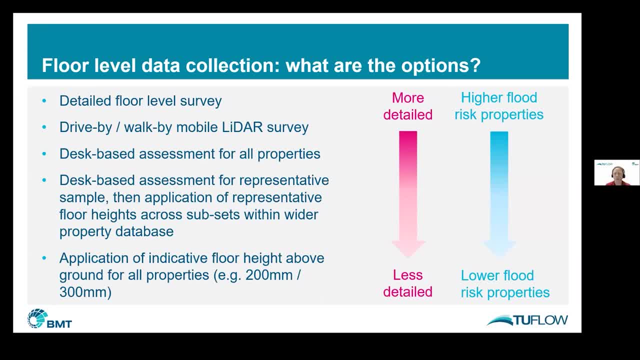 below. So you've got that detailed one I just described. but you can also do options where you drive past and you point a little laser at the top step, or you can use Google Street View, or you can use Google Street View and then kind of apply it instead of doing it house by house. 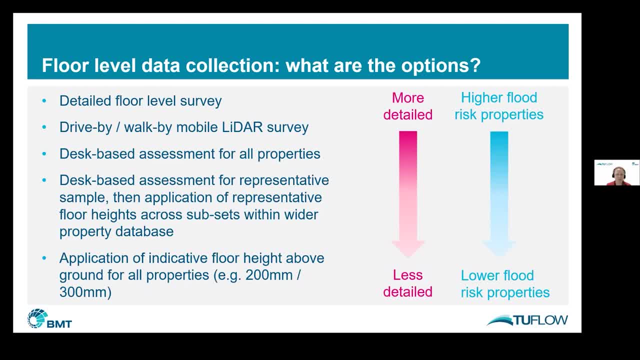 just apply it as suburbs. Or the coarsest approach is simply to just extract the ground level for every property and add some nominal freeboard, So 200 mils or 300 mils above ground level, and just assume that that's the floor level of your property. 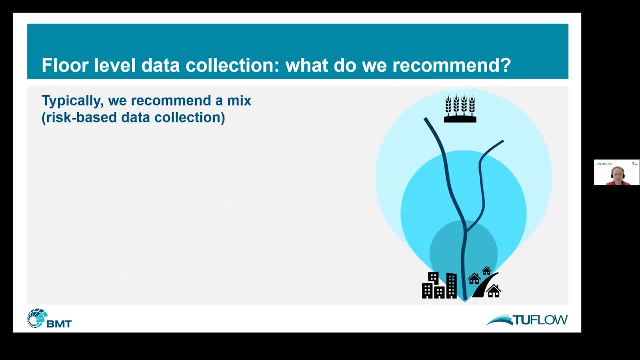 And typically what we do and what we recommend is actually a mix, So you'd say this is a risk based approach to data collection: The areas that are in the lowest risk, so furthest out in the floodplain, they're only likely to be flooded very infrequently. 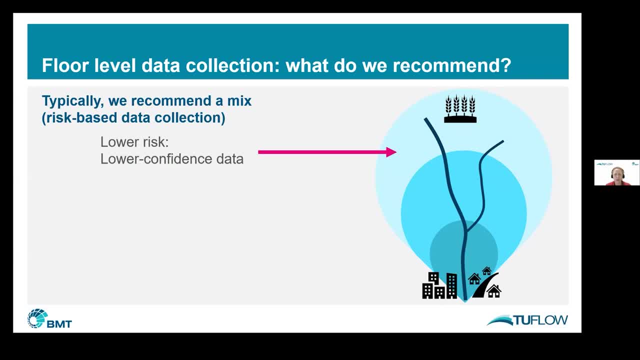 That's an area where you can use some lower confidence data because they're not going to be flooded very often. In terms of your damages assessment, it makes a much smaller contribution to your average annual damages where you're introducing the data, where you're introducing the data, where you're introducing 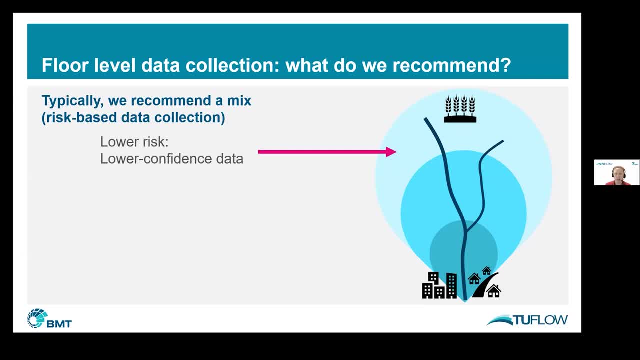 measures that you'd like to test. they're unlikely to be way out there at the edge of the floodplain But, conversely, in those areas which are subject to frequent flooding and there's a higher risk, you absolutely want higher confidence data, And this is a smaller 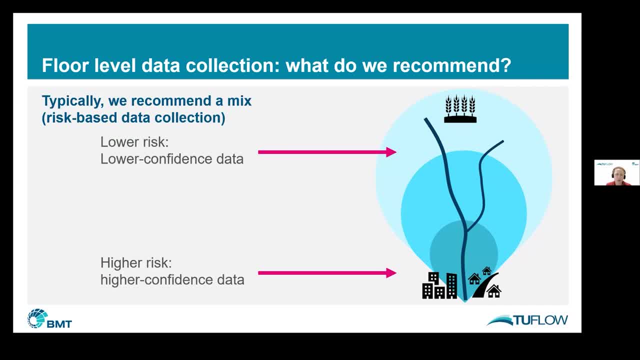 area. it's a subset of your floodplain, so hopefully you can afford to spend a bit of money and do a slightly better data collection process there. So by mixing and matching, we get this tailored approach to data collection and it's informed by a. 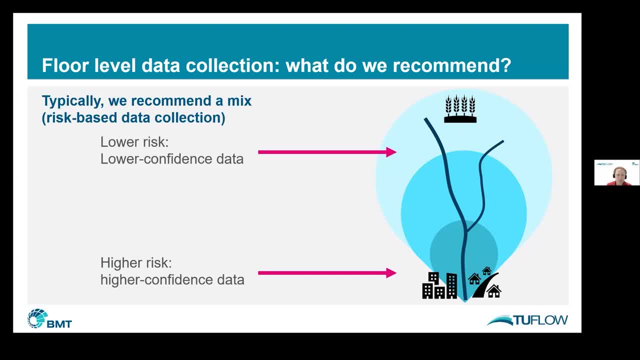 risk-based decision. So I think that's something we've done before and people may have done the same mix-and-match approach, but it's just thinking about why you're doing it in terms of confidence and compromise And when you're considering what to do. 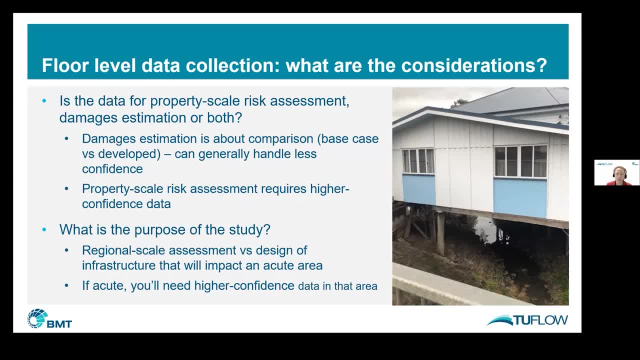 think about how that information will be used. Is it for that property scale assessment or damages? So with damages you can generally handle a bit less confidence in your data because it's being used for a comparison basis. But if you're going to be reporting information, 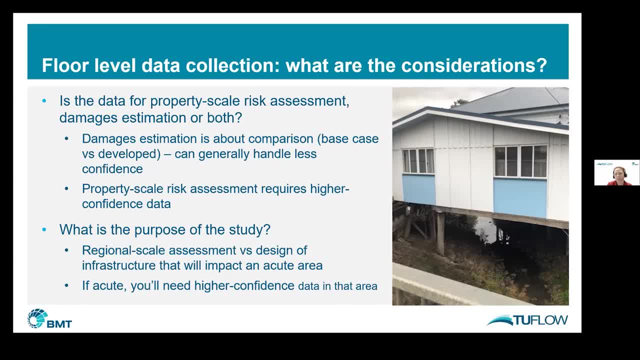 back to property owners at that property scale. you definitely want higher confidence data. And similarly, is it just a regional scale study? Are you looking at trends over the entire catchment Or are you thinking about introducing some infrastructure, some structural mitigation measures that will impact one particular area? In that case, you'd want some higher confidence data. 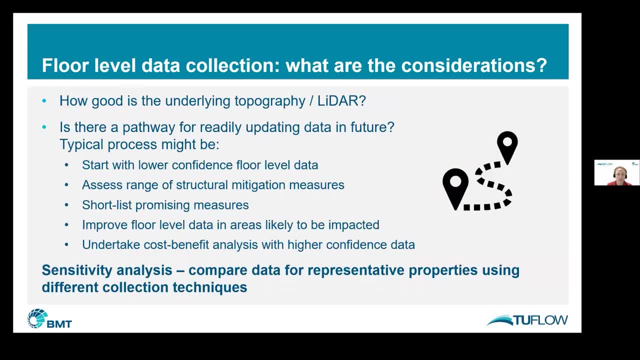 in that area that's likely to be impacted. So, in terms of those considerations, yes, consider how good your ground levels are, especially that final option if you're just going to stick a nominal amount of freeboard on top of your ground level, If it's rubbish data, to start, 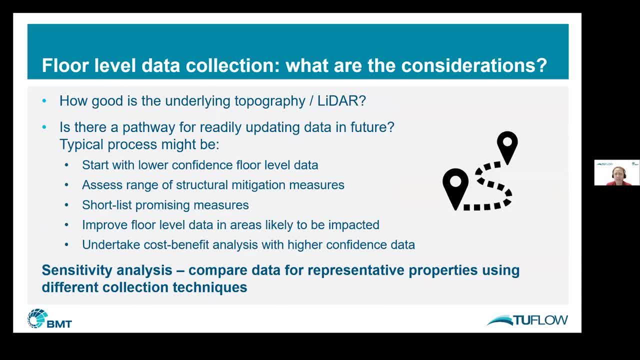 with. you're just sort of building bad upon bad. So really think about that and what it means for your study. But also this pathway, and this is something to consider: for all these options, Is there a pathway for updating it if you need to in the future, So what you might do, even within? 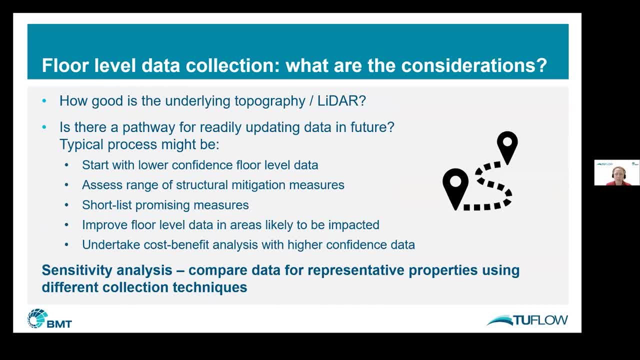 the course of one study is: you might start with lower confidence first and then you might start with lower confidence first. So you might start with lower confidence first and then you might start with lower confidence first. So you might start with lower confidence first and then you might start with lower confidence. floor level data. 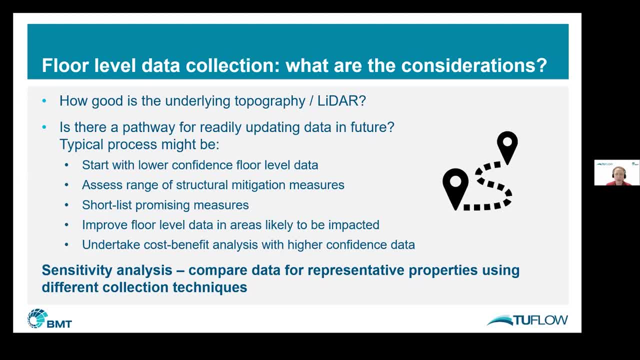 And then assess your range of structural mitigation measures that you're thinking about- short lists and promising measures- And then, if there are some measures you'd like to go forwards with, you can improve the floor level data in those areas where you might get impacts. 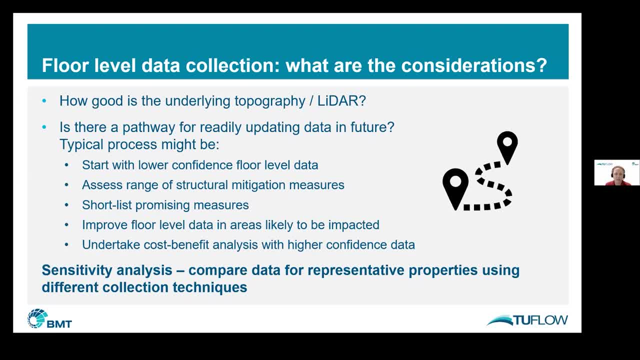 So if it's just a small area behind the levee where you're expecting adverse impacts, go out and collect better floor level data there and then repeat your damages assessment and your cost benefit assessment. So again, a risk-based approach to data collection. 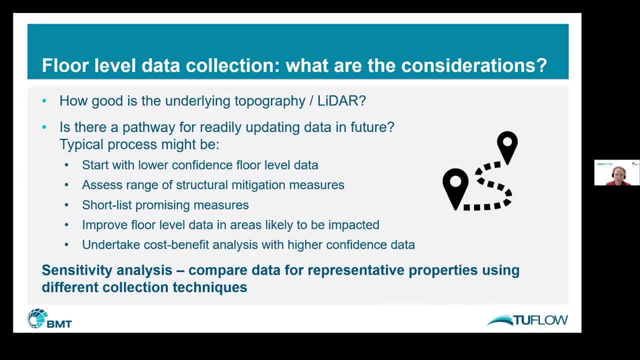 And finally, of course- and I think this holds for pretty much- you know everything- you can do a sensitivity analysis, So compare data. If you've got some good data, try your coarser approach for the same property. see how different they are. get a feel for how much. 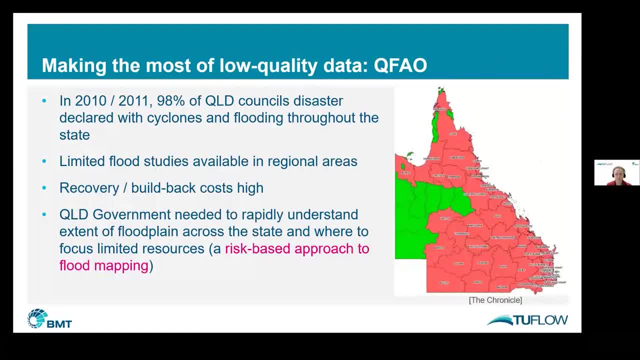 uncertainty you've introduced by compromising. So the next example I've got here is about using low quality data. So this is a Queensland-based example in the state where I'm presenting from. So about 10 years ago, in 2010 and 2011,. there was a massive summer of disasters, natural. 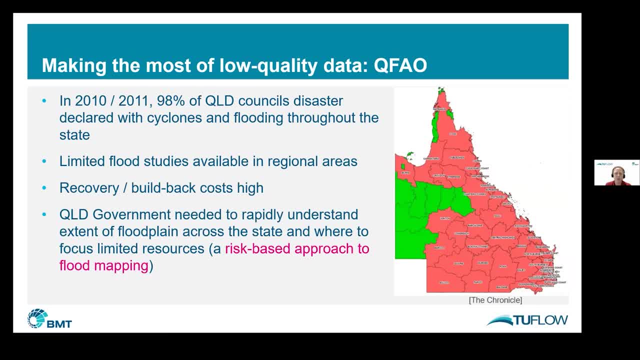 disasters throughout the state. So there were big cyclones. there was, you know, rain for months flooding up and down the state, saturated catchments, flash flood events, all these kinds of things. So you can see there on the map 98% of the council areas in Queensland. 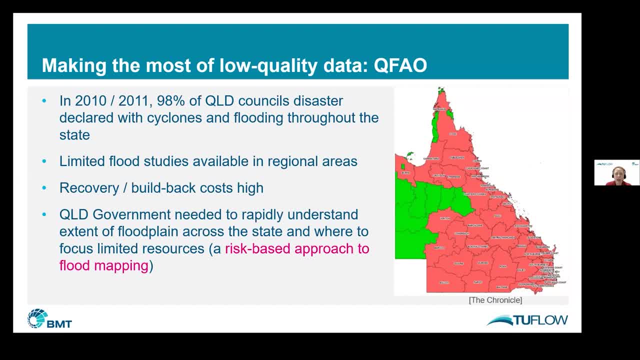 were disaster-declared. It was atrocious. And suddenly the Queensland government realised that they didn't have. you know, they didn't have. you know, they didn't have, you know they didn't have. well, not suddenly, I'm sure they're aware, but it became pressing that there weren't detailed. 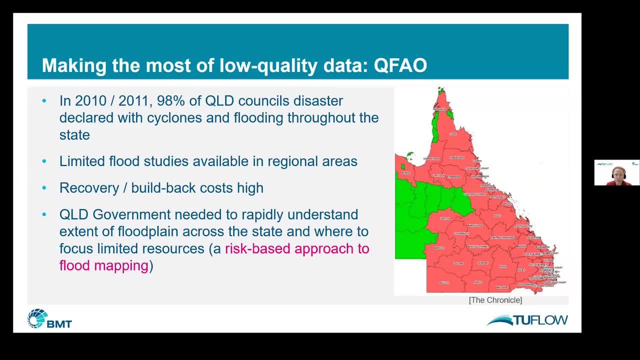 studies throughout the state, detailed flood studies- But unfortunately it happened at a time when there's also a lot of investment required in the recovery space- repairing infrastructure, all those build back costs- And so the Queensland government needed to come up with a way to quickly understand where there might be flood risk throughout the state. 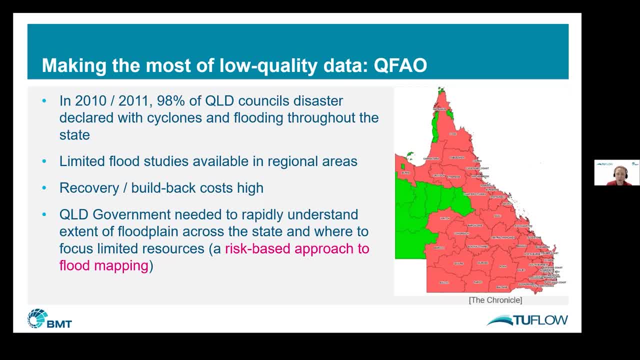 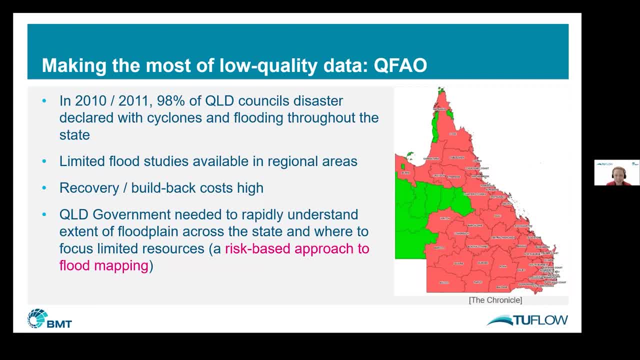 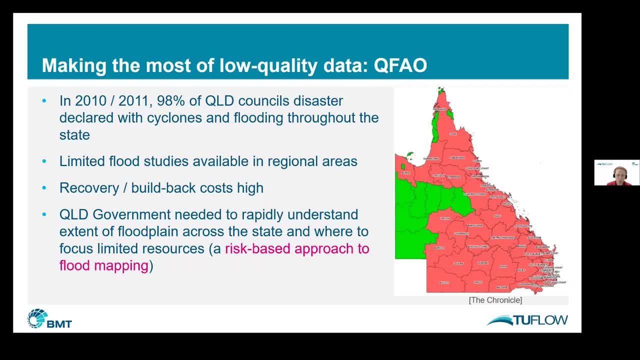 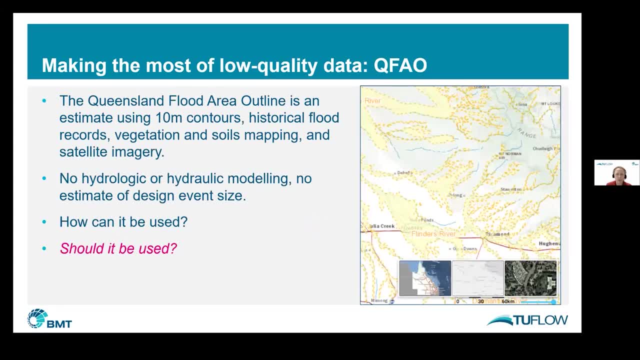 you might call a risk-based approach to flood mapping: Do something coarse to start with and then use it to identify the risk to go in and do some more detailed assessment. So what they produced was this thing called the Queensland Flood Area Outline, the QFAO. 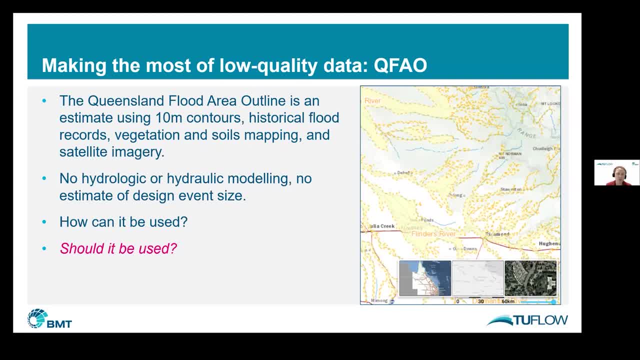 And it actually isn't based on any hydrologic or hydraulic modelling at all. it's a GIS desktop exercise using contours, flood records, soil mapping, satellite imagery, those kind of things. You can see an example there on the right and it's available online. 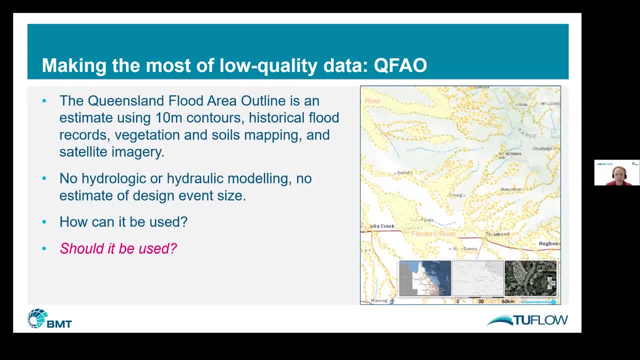 if you'd like to have a look at it, And this is a really regional area. I'm showing that image there. There's no way there would otherwise be flood studies in that location, But we know its origins and we know it's actually low-quality data and the government themselves know that. 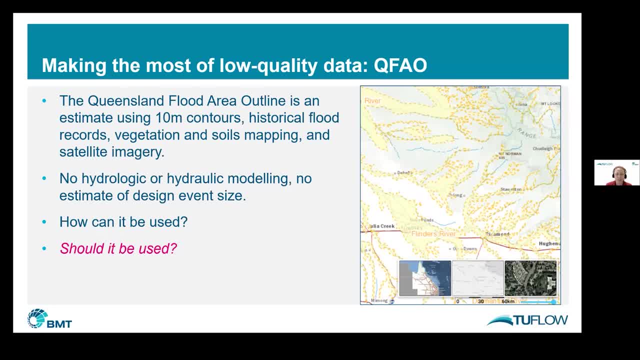 I'm not slurring the Queensland government there at all. It's just a first pass And the question is: how should it be used? And in fact, should it be used at all If it's such low quality? should we just ignore? it Is something better than nothing in this case. 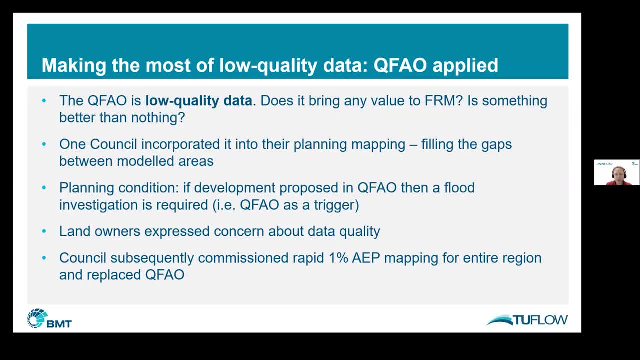 So there was one council who did introduce at least one council. It was a large regional council with lots of town areas. They had been terribly impacted in the floods And gone through a process of developing good, solid flood modelling in their town areas. 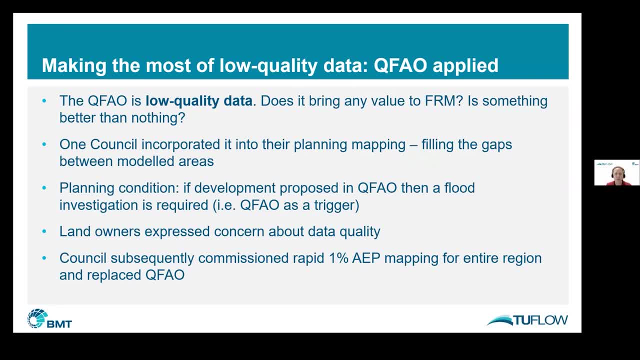 But they had the spaces between the towns, the farmlands, where farmers were wanting to build things that would impact flooding, like levees, earthen embankments and farm dams. But there wasn't already a flood model there, And so the approach the council used- and it was an informed 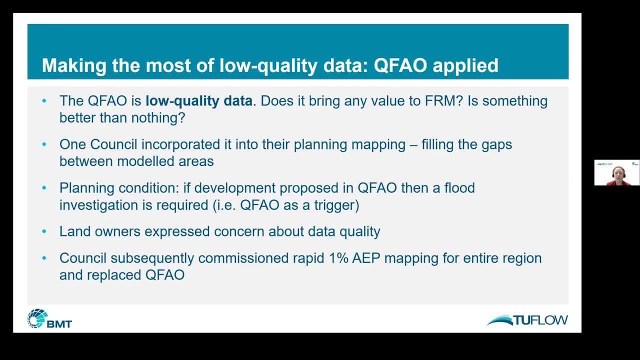 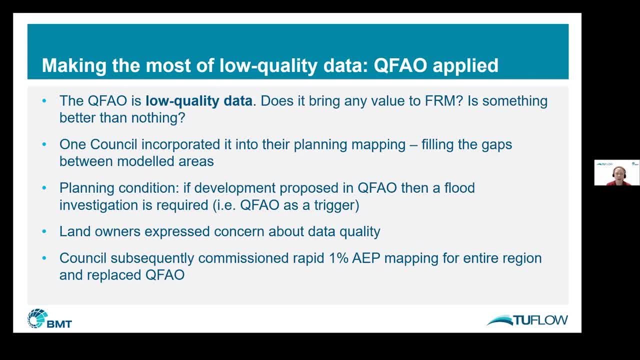 so that if you were in that QFAO area- QFAO area between the detailed flood models and you wanted to develop in a way that would impact flooding- it was a trigger to say, okay, you have to go and do a detailed flood investigation of your own. But when they took it out to the community, 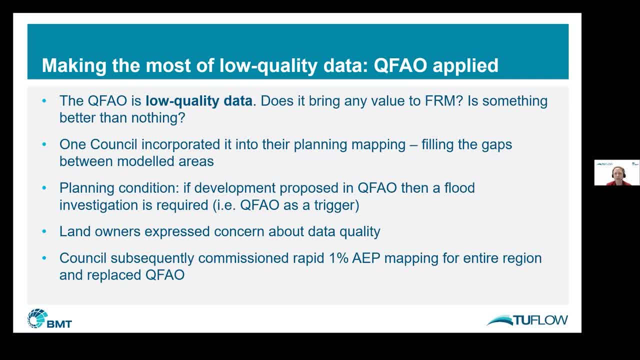 the landowners expressed some concerns. They felt that it wasn't good enough quality to be, to be sensible, to be useful for anything, And so they went back to council and you know, council eventually refined their approach. They went back and they commissioned some, some 1% sort of rapid 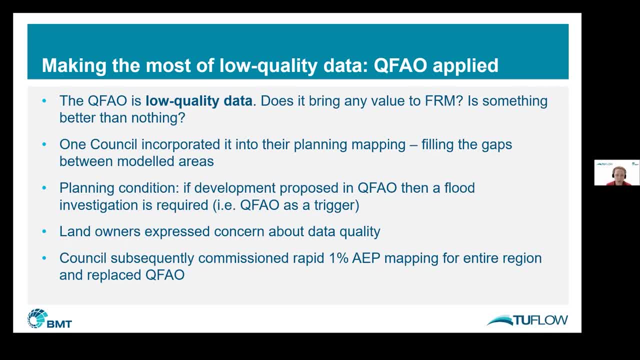 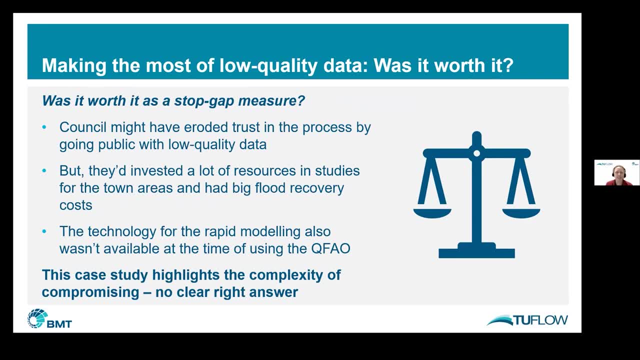 mapping for the entire region, which ultimately replaced the QFAO. So was it worth it? It's not an easy answer. actually, It's because they might have eroded the trust in the public by going out with this low quality data. but what were their choices? You know, they didn't have any further. 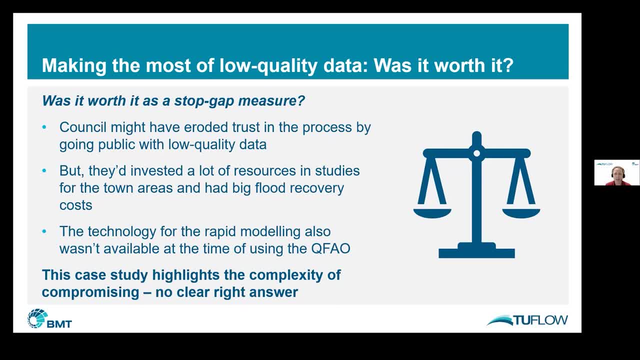 budget at the time to do that, And so they went back and they commissioned some- some 1% sort of time- to do detailed modeling between the towns. There was no driver for it. It's a low risk. There might've been hazard out there, but there wasn't a lot of exposure. but also that the 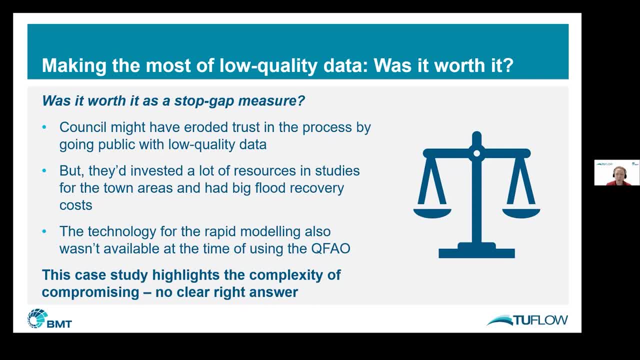 modeling that ultimately replaced it, the technology for that that, the GPU modeling- it wasn't available at the time when they first introduced the QFAO, So they they didn't have that option available to them And you know, I think they did the right thing in terms of 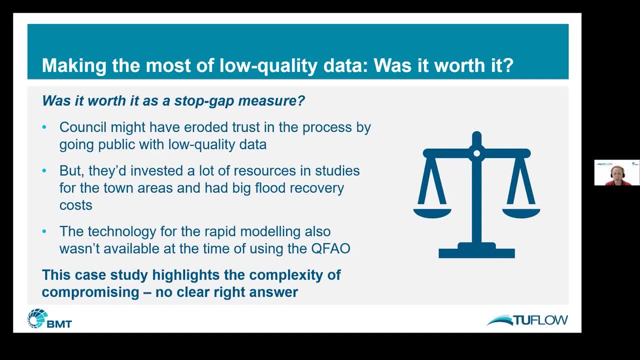 of going out to the community, listening to their concerns and being prepared to treat their response as dynamic and updating it when better information was available. But overall, I think that was a really complex situation And this is what happens with compromises And it's what happens with flood risk management studies. all the time This is 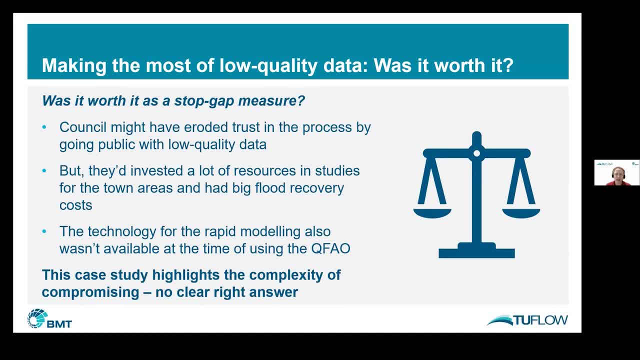 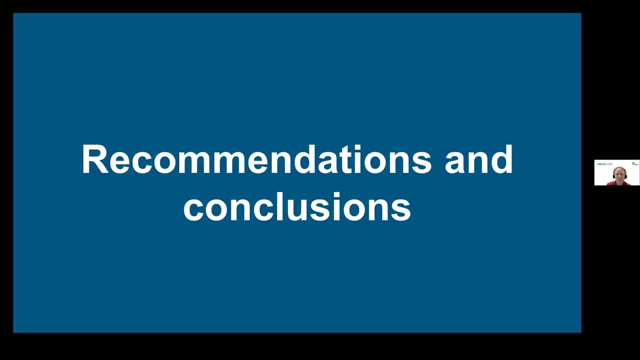 one particular case study, but this type of thing always happens And if you're involved in flood risk management, you'll be having to make these decisions all the time. So I'm just going to wrap up now after our examples. So I'm going to wrap up now after our examples and I'll see you in the 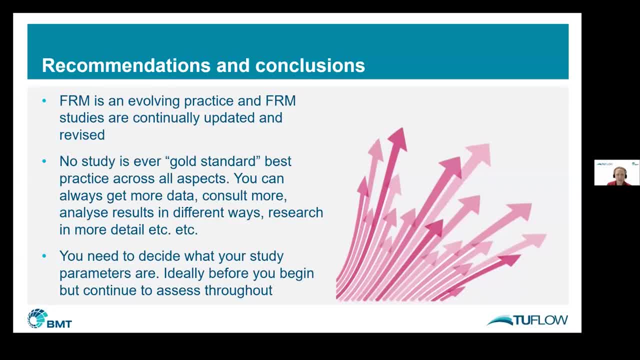 next few minutes And just to give you a few recommendations to take away. So, as as Jackie mentioned, flood risk management is evolving and studies are always being updated, So don't see things as a static document, set it and forget it. Gold standard is a nice idea, but it's really. 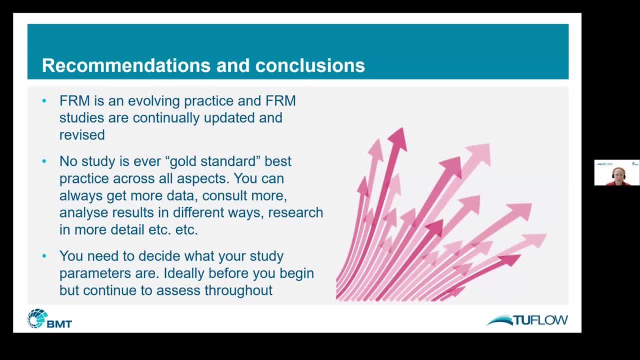 really impractical. You can always do more You can. Sometimes you should try for it And sometimes you need to just keep moving on, Otherwise things will never get done or implemented. You should think about what your study parameters are, All those points I raised earlier about why. 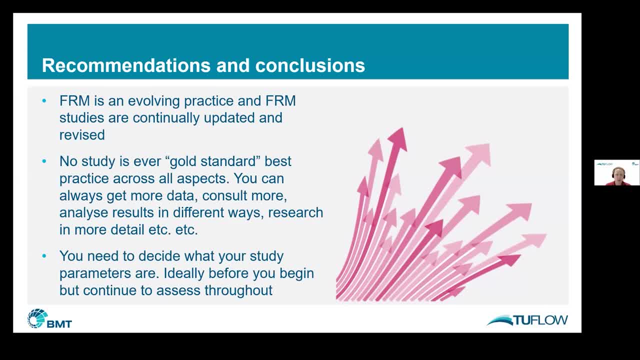 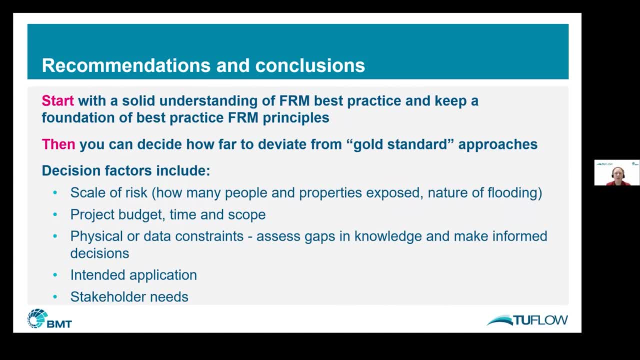 you're doing the study? what are the limitations of their political issues and so on? Think about that before you begin the study, but continue to assess it throughout. Make sure you start with a really solid understanding of flood risk management principles and best practice. So the principles: 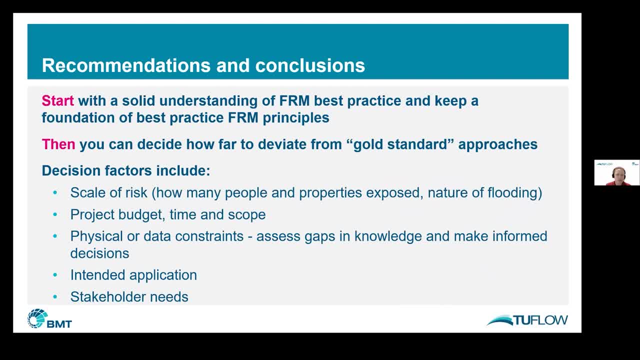 that Jackie outlined the best practice in terms of technique and good quality data and scope and things like that. Once you have that understanding, you can start to think about what your study is going to look like And then, once you have that understanding, you can decide how far to deviate. 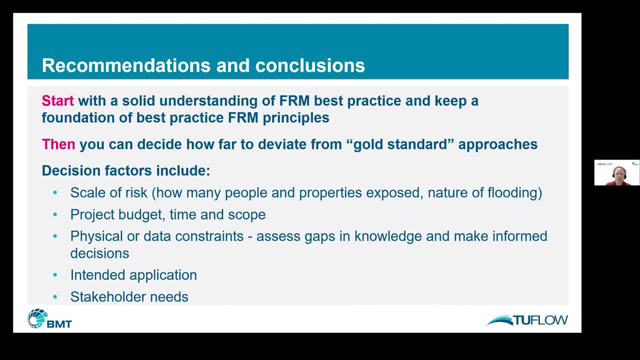 from those gold standard approaches. So always keep the principles, the best practice principles, ongoing in your study. but the approaches, the data, the scope, the timing, think about how you might need to compromise those to be able to move forward, And the things to think about will be: 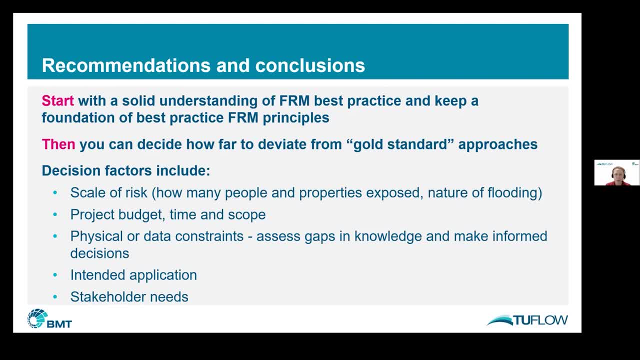 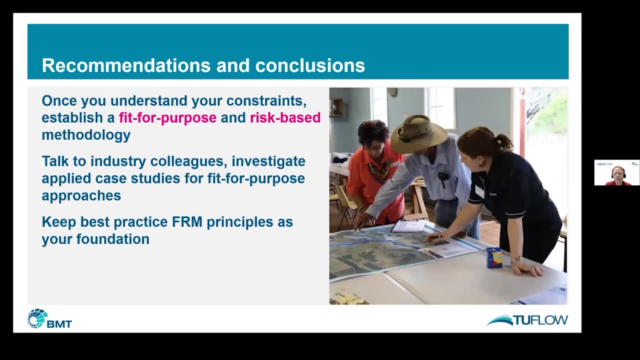 that scale of risk, how many people are in the floodplain and exposed to what level of risk, your project budget, time, scope, any constraints in the data, what the project is going to be used for and what do stakeholders need out of the project. Once you understand that, you can then 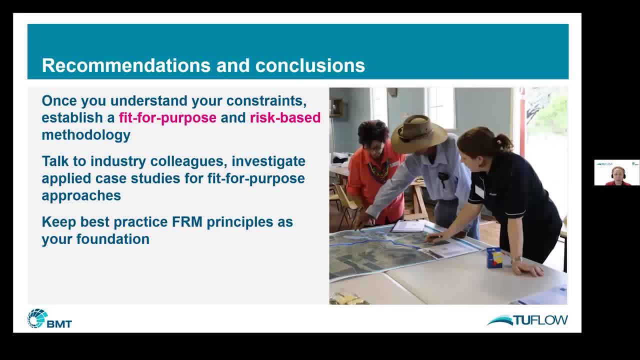 establish your fit for purpose and risk-based methodology. And a really good place to get ideas for this is looking at other case studies. go back to conference papers when people present what they did on their studies. It's a really good resource If this kind of best practice gold standard thing. 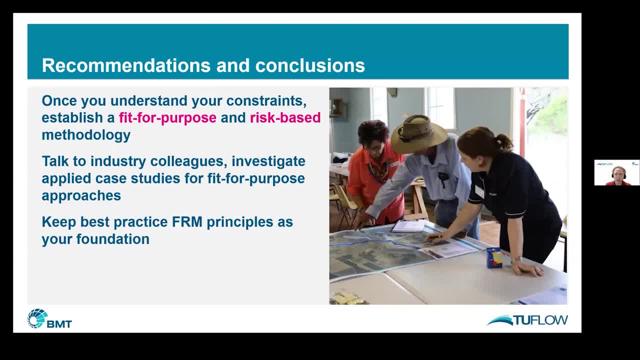 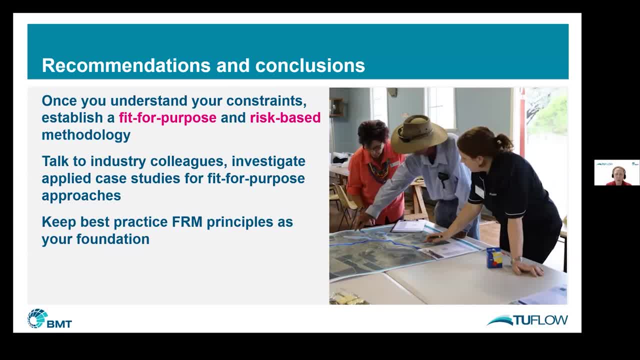 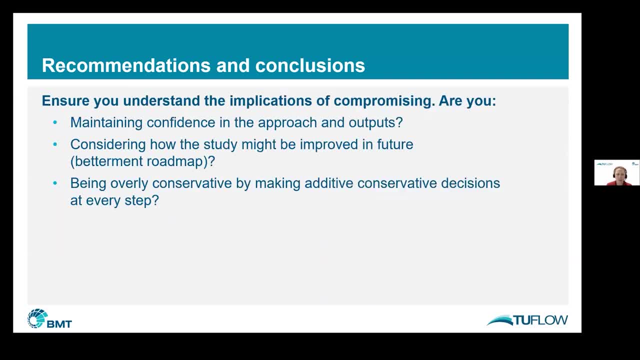 So use that resource and think about how you can use other people's approaches in your own study area And, of course, keep those flood risk management principles as the foundation all the way through. Think about this issue with compromising, the implications of it and the 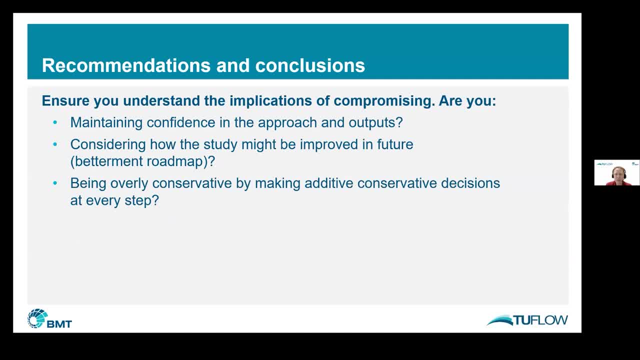 confidence in your outputs And I think something which we're starting to see more in flood risk management is not just an implementation plan. It's an implementation plan, It's an implementation framework, but a betterment road map, recognizing that you couldn't do everything the way you wanted. 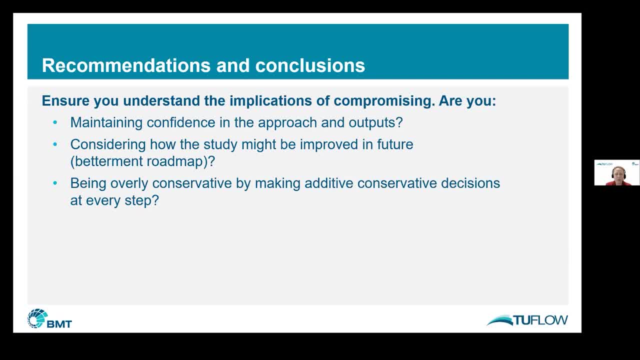 to right now, often because of budget constraints, but you know you want to move towards it in the future. So you say, okay, let's break this into little chunks of work. We can do this right now And it's useful as a standalone piece of work, But we can also see that it's part of a process that, if 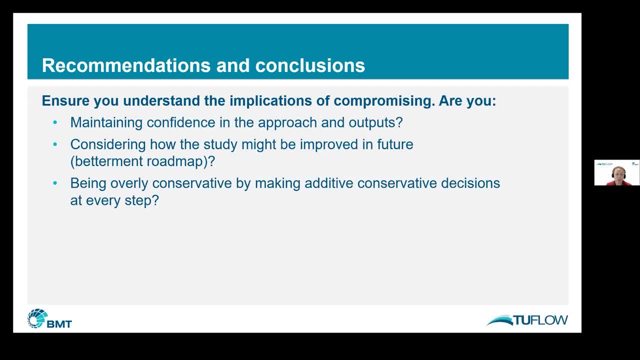 we do this, subsequent steps, we'll develop a really good outcome. So think of that in terms of a roadmap of works And this issue of being overly conservative, And so I think this is something that's quite important And that's something that we were trying to kind of discuss in a different context. 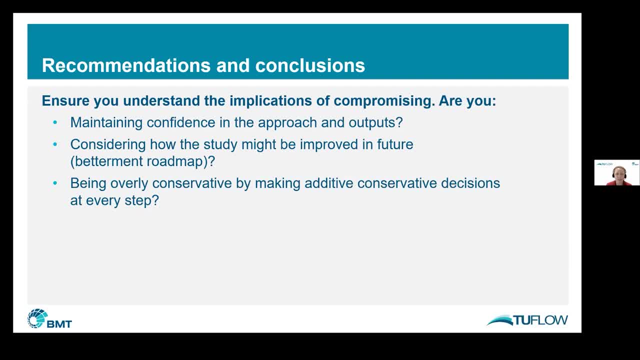 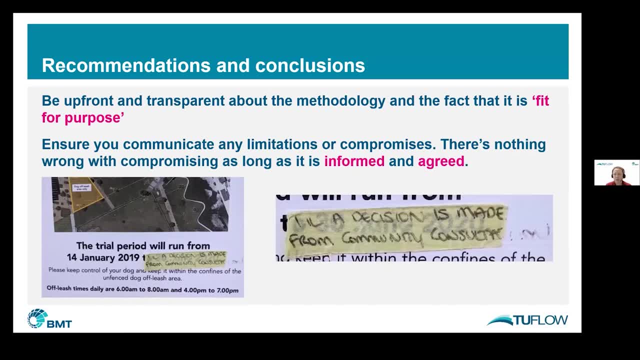 but it's a really good one And we see as an example of a process where we want to do it. we go back and we- and this issue about being overly conservative- keep that in mind. So, overall, I think our big push is that you need to be upfront and transparent about what you're doing and the fact that it's fit. 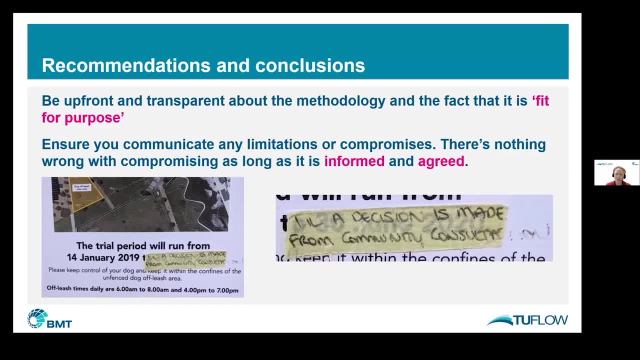 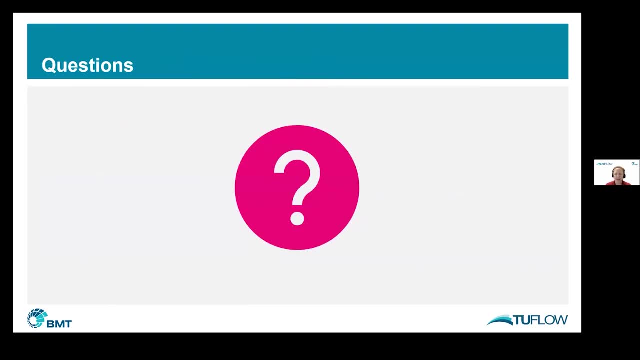 for purpose and that you communicate anything you've had to do in terms of limitations or compromises. It's okay to compromise and you'll need to just make sure that it's informed and agreed And that's all. Thank you very much for joining us. I think Jackie and I will take 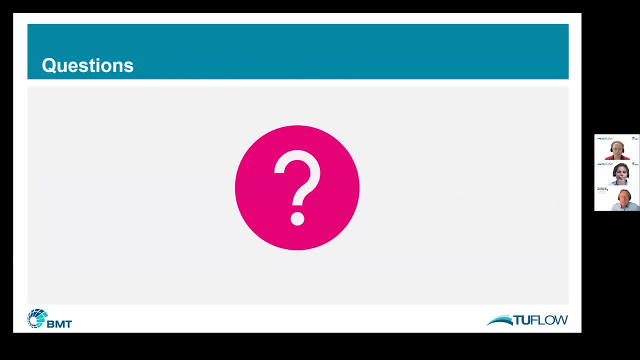 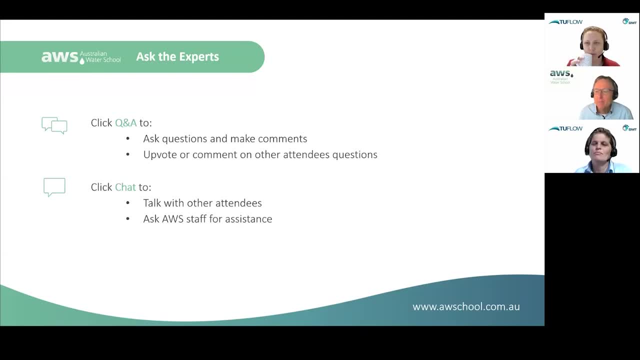 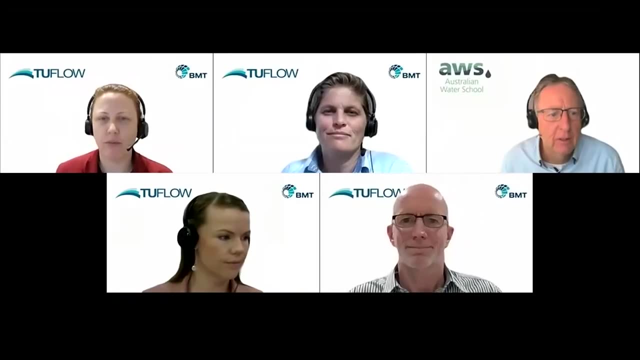 questions at the moment. What a fantastic, what an absolutely fantastic presentation. It's just big picture with heaps of complexity and Carrie Jackie, absolutely brilliant. Come on screen, Bill Tegan and Jackie. Are you there? Yes, she is. 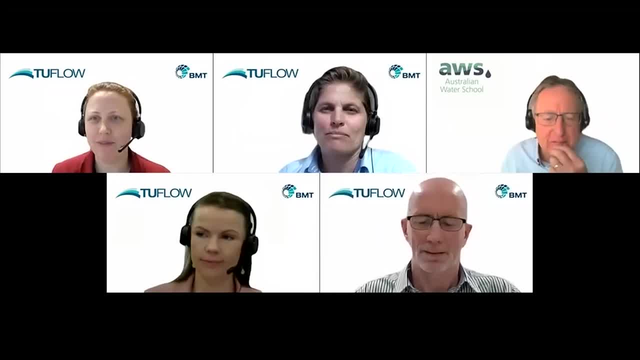 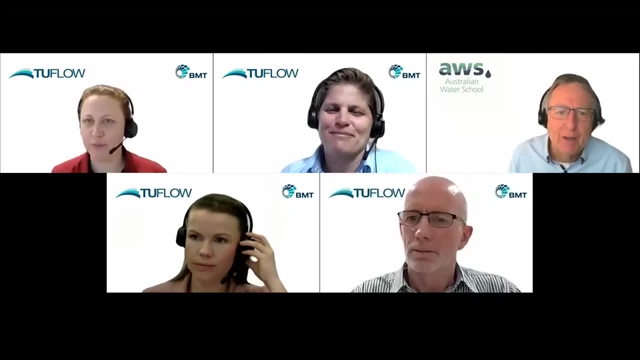 And I'm going to hand over to Anne to chair this next piece. Thank you for your questions, everyone. It's brilliant. Where would you get five of the best flood risk managing professionals in one place at one time? Right here, Australian Water School webinars- and it's free, But look. 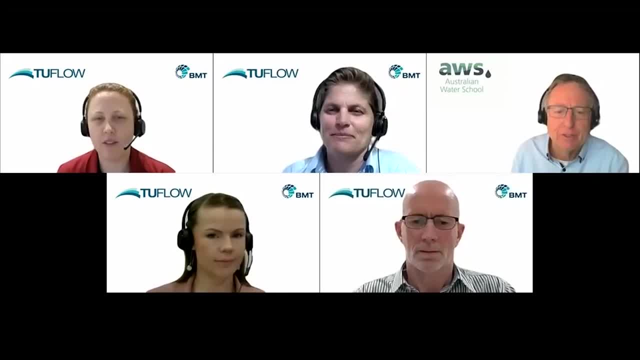 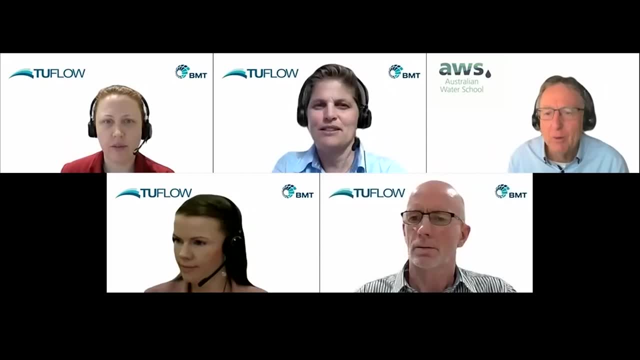 this hasn't been easily come by this experience of professionalism. No more words from me. Anne. take us through some of the questions that have been pounding through the Q&A icon while they've been speaking. Thanks, Bill, Thanks very much, Trevor, And the questions are really wide ranged and stuff, But I thought 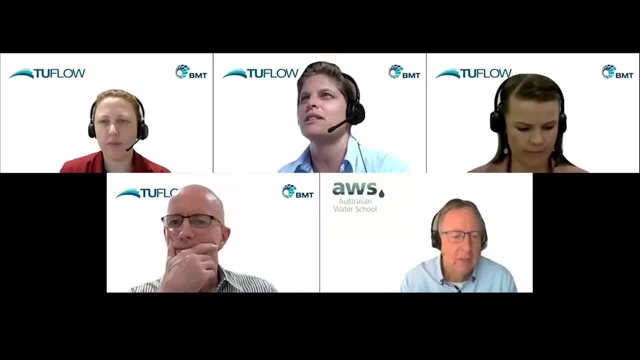 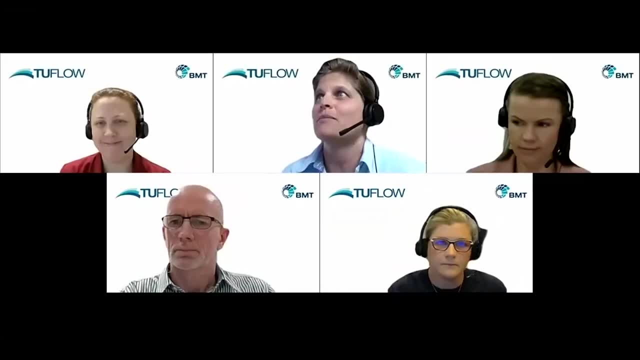 it really one that got a lot of interest. is is for Jackie. So here we go. When should we consider strategic retreat versus investment in mitigation? I thought that was a really interesting one, So I'll hand over to you, Jackie. 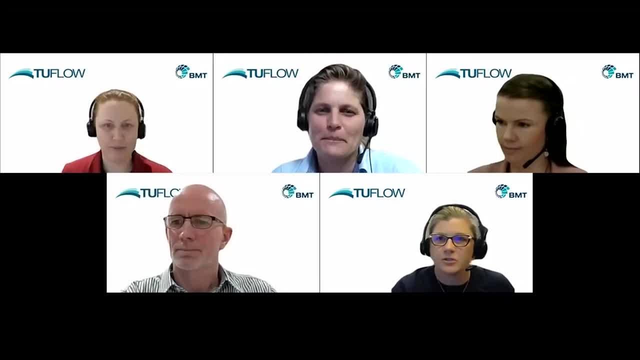 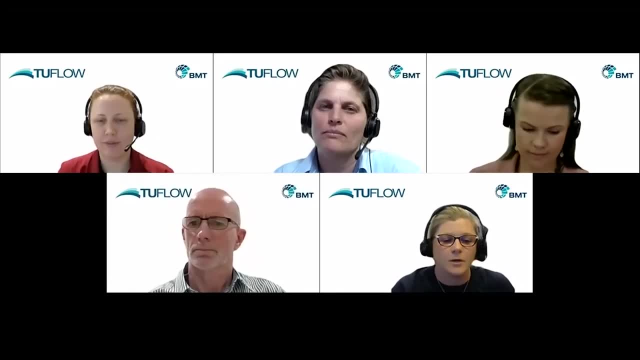 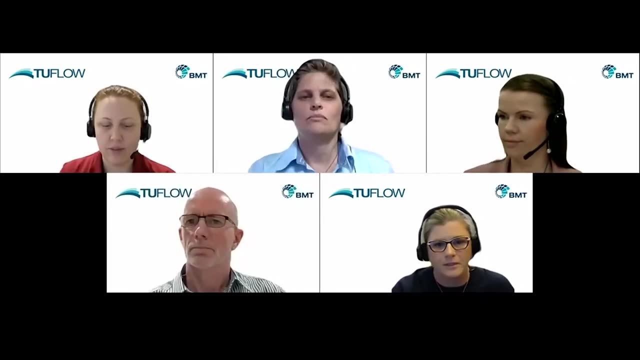 Thanks, Anne. I suppose in terms of this question it really depends on a consideration of the type of development in an area and also the type of flood risk. So in my presentation I discussed existing risk, future risk, residual risk. So from my perspective it's really that residual risk. 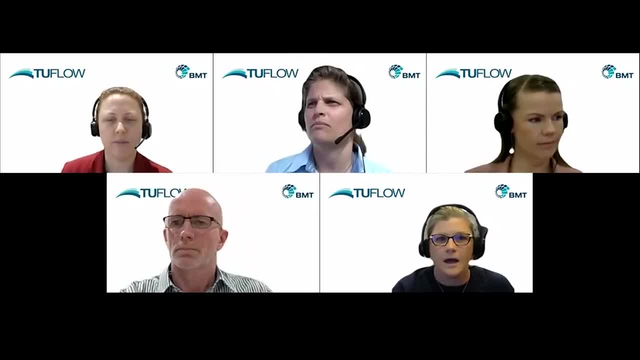 that's possibly the most important component in answering that question. So you know, in the risk hierarchy we talk about, you know, avoidance and we talk, and then we also consider risk to life, risk to property. So it's really 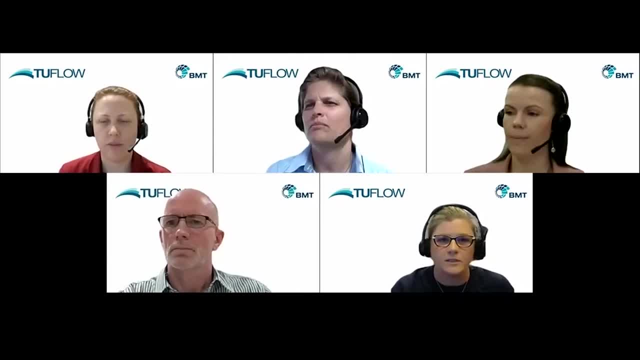 I suppose when that risk to life from the residual risk becomes intolerable or unacceptable, you know we really want to ensure the community's safety. So you know, if there's a, if the type of development, say residential or vulnerable uses, and your residual risk is just. 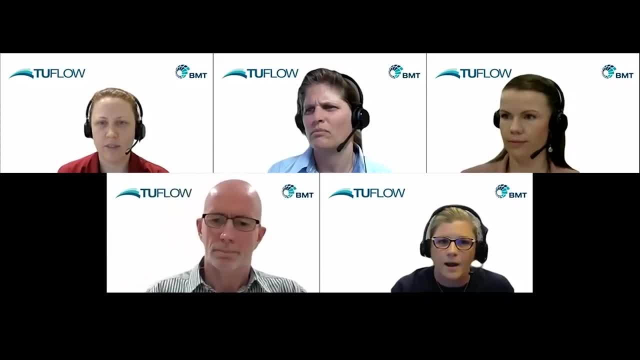 too great. people can't evacuate. people are going to be trapped by, you know, a probable maximum flood. you know that's really when you would definitely start to consider strategic retreat and moving people away from that high flood risk to more areas of acceptable flood risk. 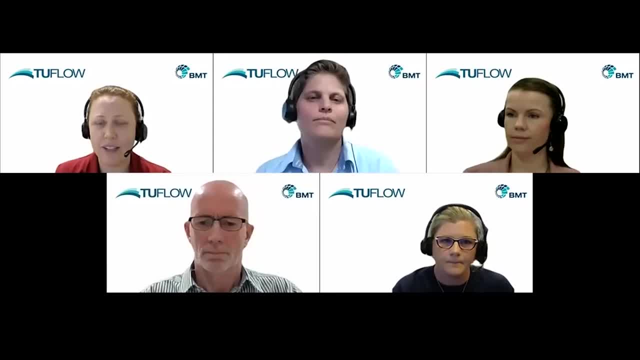 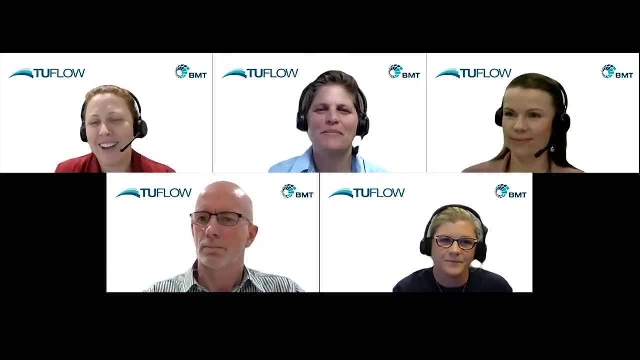 I'm not sure if you have anything to add, Carrie, Yeah, I do, And you know I've got my favourite planner on the line. I saw her there, so she would kill me if I didn't jump in- which is that it should be considered. I think more and more in. 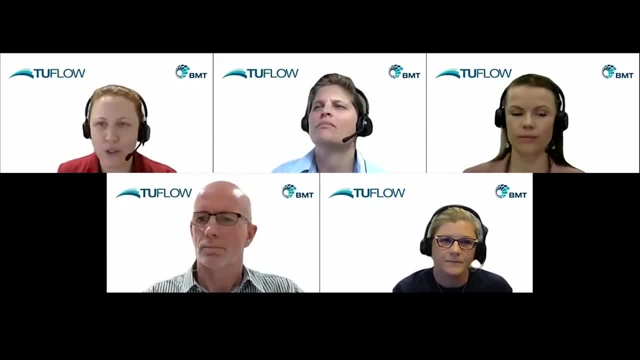 strategic planning. So East Coast Australia has had a terrible summer of floods And there's been a lot of discussion, more than we've ever had before, about retreat in terms of flooding. It's been around in terms of coastal inundation for a while, But in flooding it's been really around the edges in. 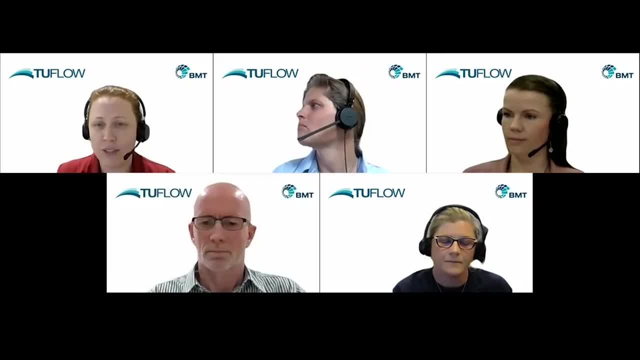 terms of a few property buybacks here and there. The federal government's recently released a lot of money for property buybacks, But that's you know, just house by house. I think that if good strategic planning is done, then you can understand where there are areas where development should. 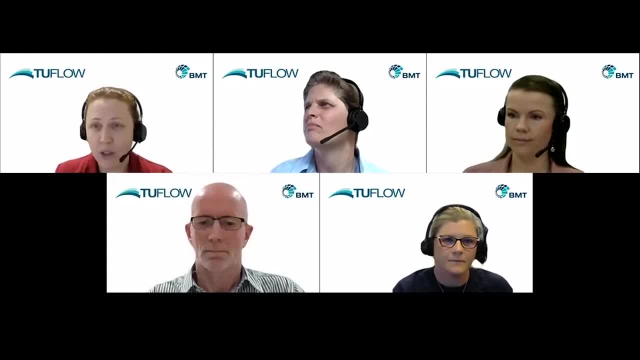 never have occurred in the future, And you could either seek to back zone in areas where there's a very high risk, so that new development can't be put in there, so that density can't increase, and you should be thinking about a transition settlement pattern. 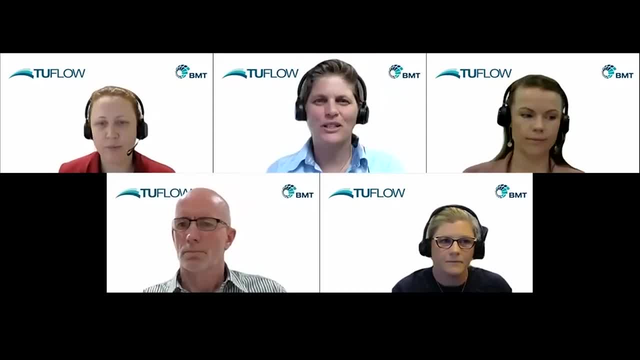 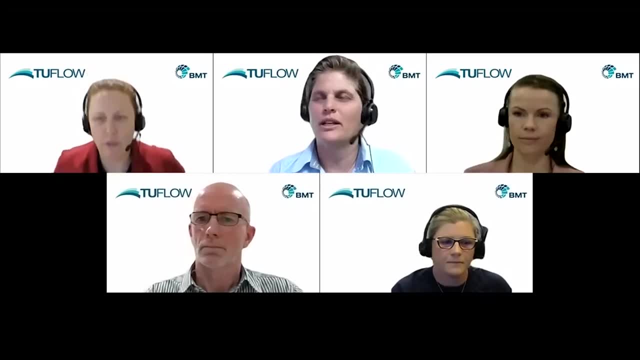 Thank you both. I think that covers that question in a lot of detail. Thank you very much. We might move on to the next one. Another one I got and might be one for Jackie: initially cost and benefits to underpin a business case. 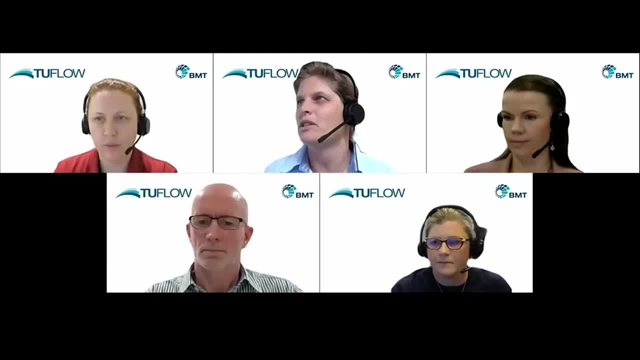 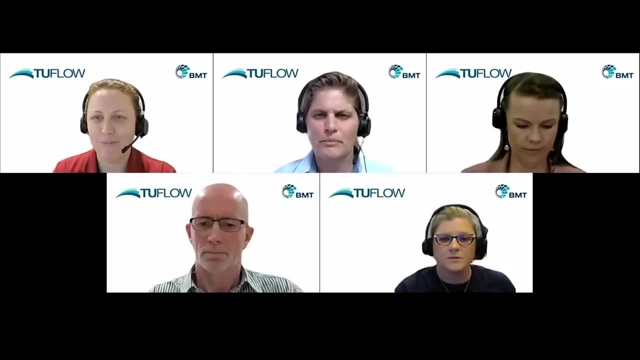 So how do we get reliable indications of indirect and intangible impacts? Thanks And yeah, well, I suppose this is the type of question, this topic, something that we struggle with a lot in flood risk management, because there's so much uncertainty in terms of. 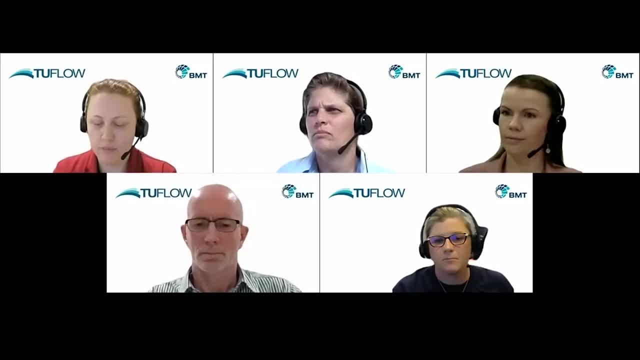 you know your intangible consequences. So I think it's really important to look at the costs, your impact on the community. you know your health impacts. you know people's suffering and you know mental health impacts of flooding And you know we've seen that a lot. 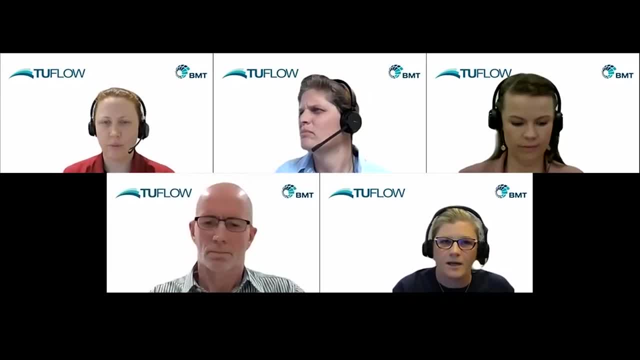 You know it's the ongoing effects. It's people who can't find accommodation and people who are stressed, you know, because they're constantly worried that their property will be flooded again. So I know, in New South Wales, you know, we have a manual that we, you know. 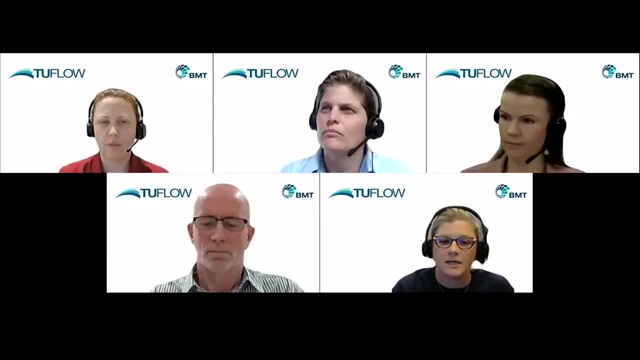 use as best practice guidance when we're doing studies. you know, and it's really, I suppose, where, yeah, when, can you overcome the uncertainty and actually quantify what the cost is? And that's really difficult And there's different approaches that people adopt, you know. is it better to? 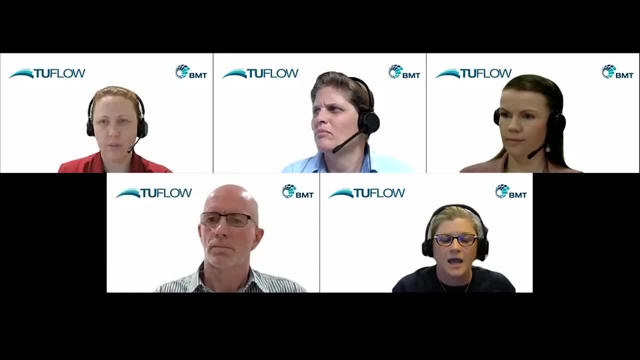 include something that's uncertain. It kind of talks to Carrie's point: Are you better to include something that might be, you know, low reliability because it's so assumed, Or are you better to not include it at all And you know if you're doing a cost benefit, is it? you know what are. 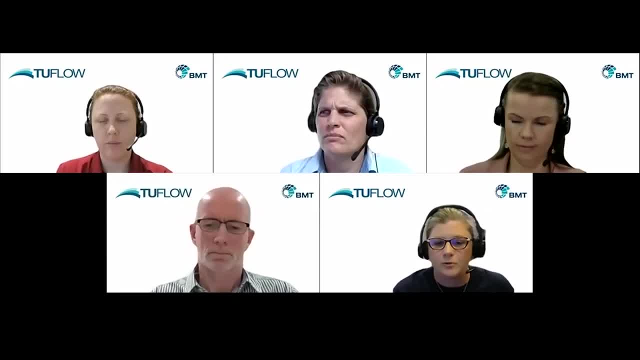 the comparative costs. So you know, if you're comparing apples with apples, you know, I suppose, does it matter, Will it change things a lot. So yeah, where do you draw the line? But I suppose in all areas you need to look at what your best practice guidance is and what they recommend you. 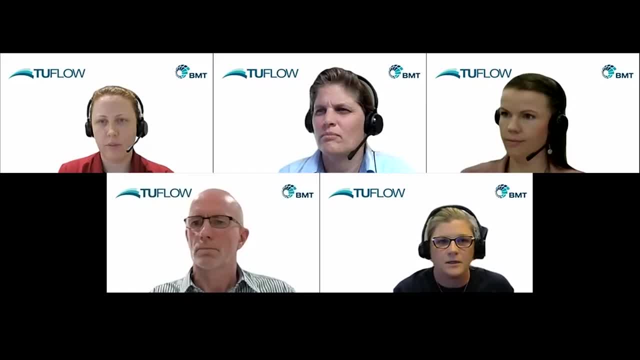 adopt and how you calculate those damages. A few extras I'd add on In terms of indirect. more and more people are starting to collect data after flood events. So historic building back damages. So if you go to councils, what they've had to pay to repair roads. 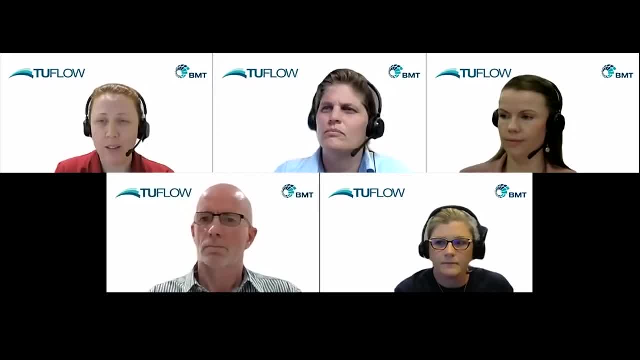 and collect that data and you could start to develop some factors, which is often how indirect damages are calculated In terms of intangibles. I think there's more and more evidence that we are grossly underestimating intangible damages, That they're much bigger than we expect And that because of that, there are decisions that 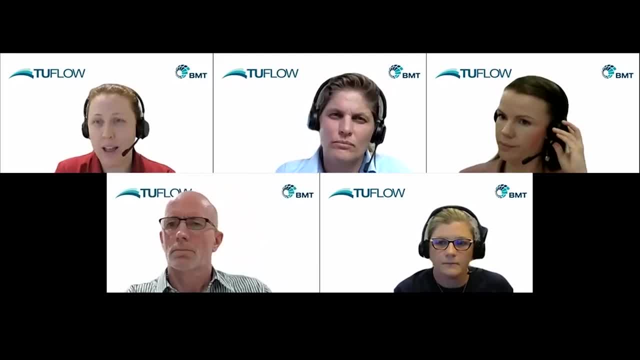 we've made in the past where we've said the cost benefit analysis doesn't stack up. You know we're not proceeding with something when actually, if we included the intangible damages, we could see a lot of value. If you would like a particular resource for the Brisbane River, 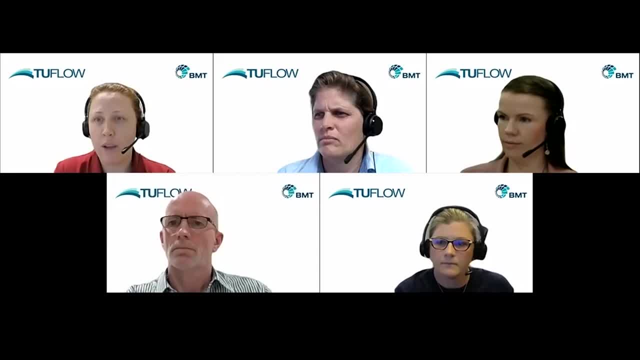 Strategic Floodplain Management Plan. it's online. We did engage an economist to do some research here on the intangibles and uplift factor And that varies by flood size. So if you're looking at the intangible damages, there are some numbers there that you could use yourself if you wanted to. 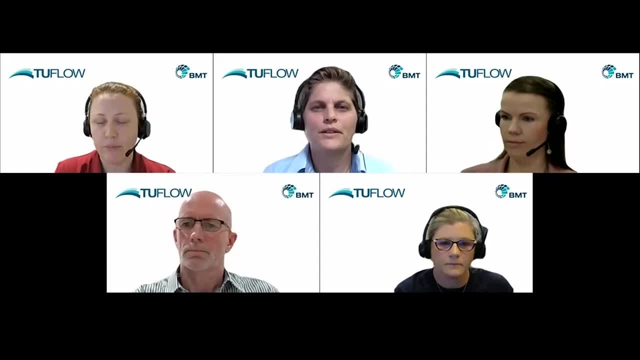 apply it in your own study. Thanks very much, Kerry. That's really good, That's great. I had a quick one. I think that's more for you, Kerry, But I thought it is still interesting to get back to And the question would be: is there a risk of inconsistency in approach when using more specific 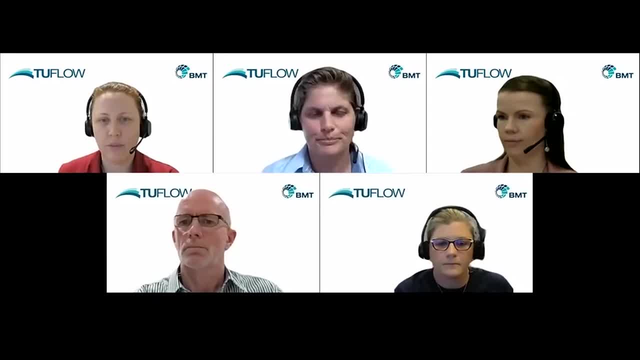 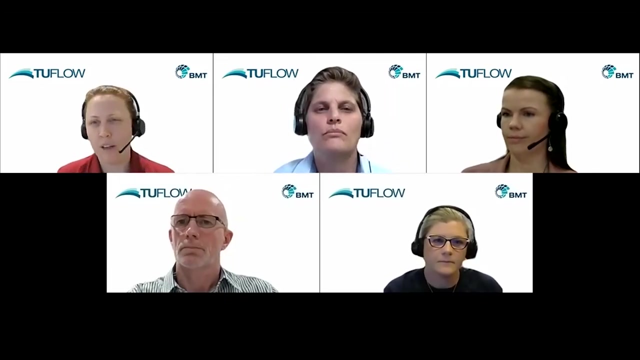 floor level for higher risk areas. There may be some risk, but I don't think it's probably a big concern. Yes, if you do it in just one particular patch, looking, as I mentioned, for infrastructure, But we're really looking at this. 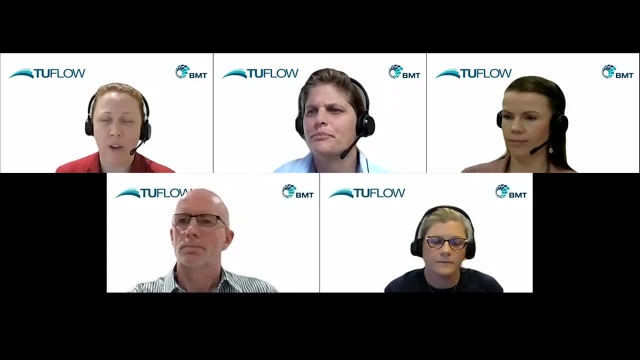 for a comparison's sake. So the example I gave, where you're collecting a bit more data after, say, a levy assessment, looking at properties that are impacted by the levy, you're using it to inform a cost benefit assessment. I think, as long as you accurately. 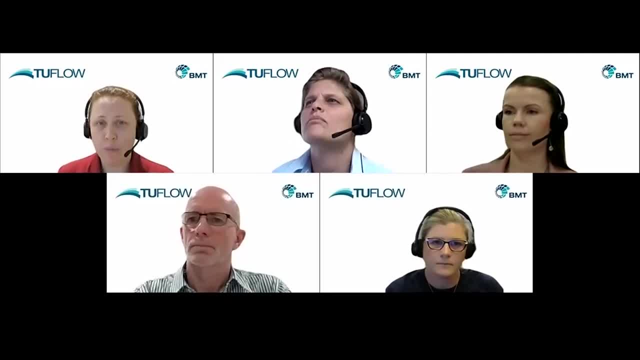 report and communicate where your data sources are from. identify that in the future, there are other areas where you might want to improve the data. I don't think that it will be a big concern to mix and match the data, And it's certainly been done a lot in the past. 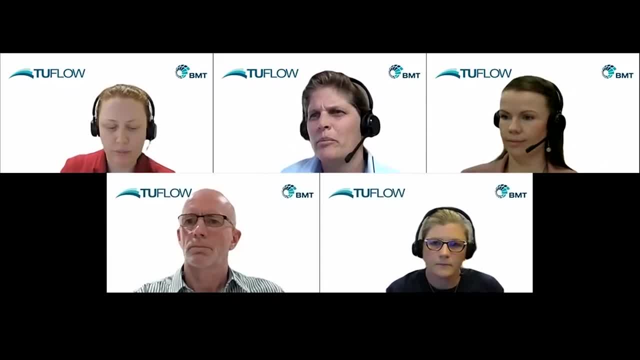 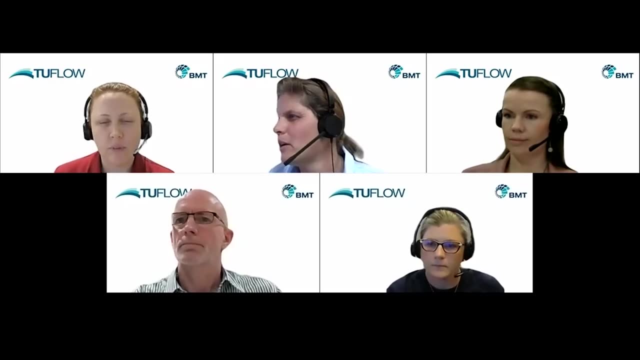 Thank you, Kerry. Yep, I think that's really good. One more here which had two more thumbs up. Thanks for a well considered presentation on best practice flood risk management. As practitioners know too well, flood risk management plans are developed with a constraint on budget and time. 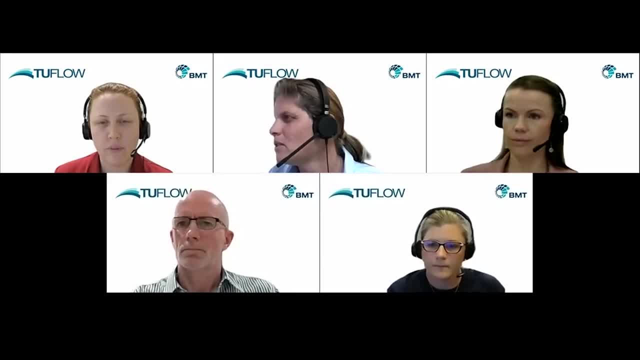 frames but still need to meet best practice expectation of the community and government policy On the issue of land lose planning. what do you see as a minimum standard of a flood risk management plan so that future risk is contained, including the impact that the plan has on the? 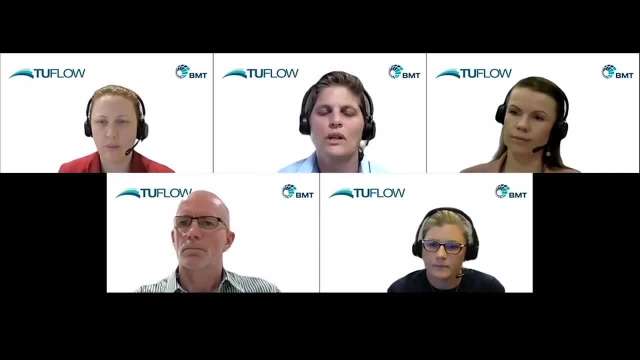 community. I think that's a great question. I think that's a great question. I think that's a great question: the impacts of climate change. Maybe that one can go to Jackie initially. Thanks, Anne. Yeah, I suppose that we're seeing climate change impacts, you know. 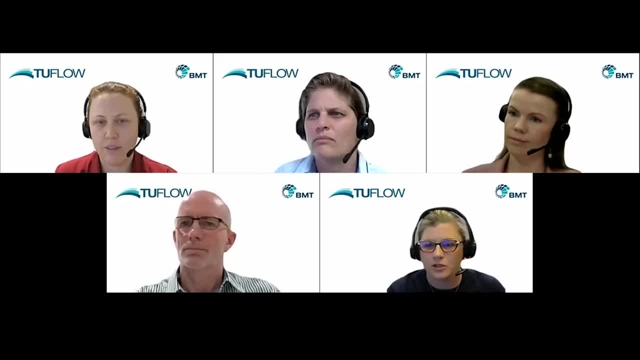 considered more and more. It's obviously an emerging topic And it has been for a while. So, you know, within flood studies, we consider climate change, we consider sensitivity To climate change And you know, I think I know in New South Wales that you know. 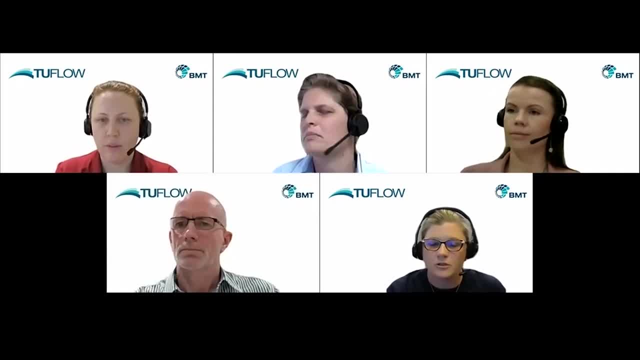 councils develop their own land use planning and policy, and different councils have different approaches. So, from my experiences, some councils that already include consideration of climate change in their, say, their flood planning levels, Whereas others just consider, you know, the sensitivity of 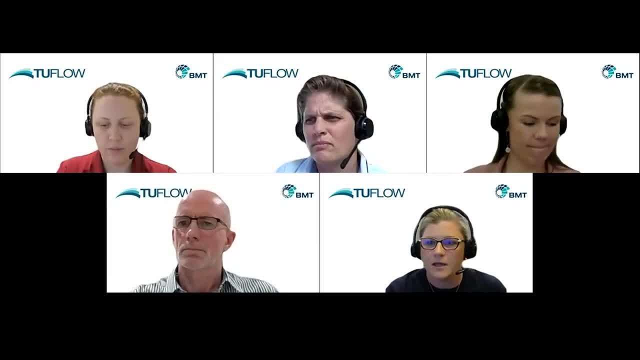 the, the, the flood risk to climate change when looking at land use planning and policy and looking at new development. So you know it's considered, but it you know a lot of councils are still relying on that non climate change impact flood risk. But I think, yeah, I mean it's obviously, it's a hot. 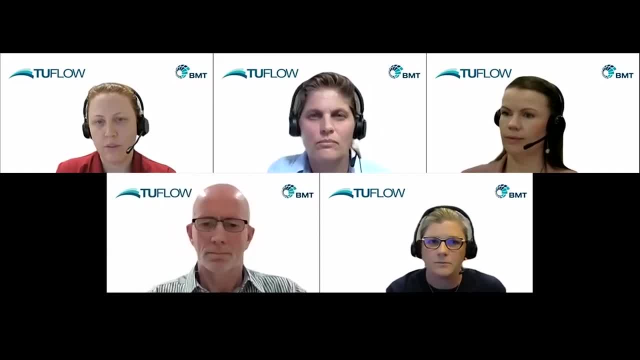 topic at the moment And I think more and more as best practice flood risk management progresses, you know we'll start to see it incorporated within the planning and policy at local government level. But, but, but, I agree with all of that. I think that that flooding is actually a little bit slow to to implement issues around climate change. I think. 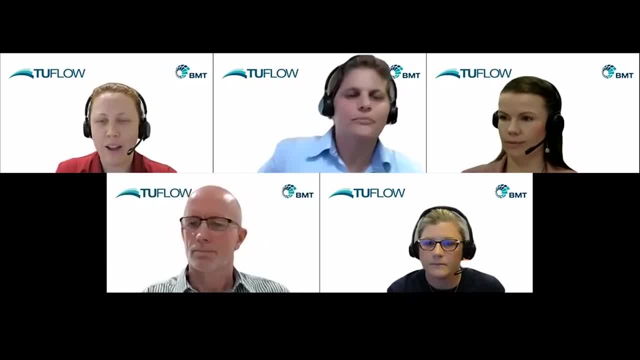 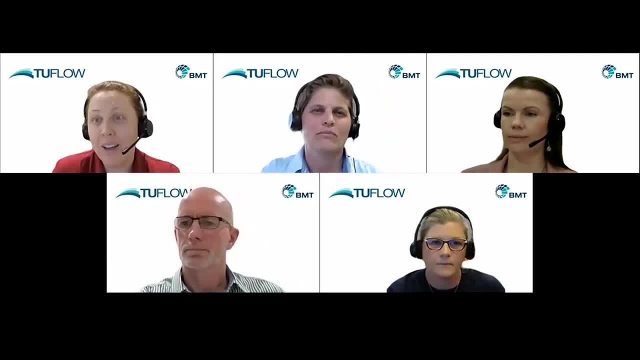 For one reason. it's it's not like a progressive creep up like you might see in sea level rise to say that flooding occurs more often and with more intensity or great, but flooding is already so sporadic so it's really hard to talk about climate change in the flooding space sometimes. 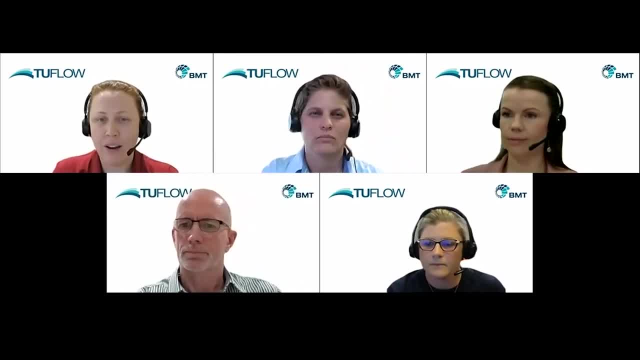 So it's really hard to talk about climate change in the flooding space. sometimes I think that that as practitioners, we should really be trying to do a bit more and thinking about how we are using that information. But there is often the case. 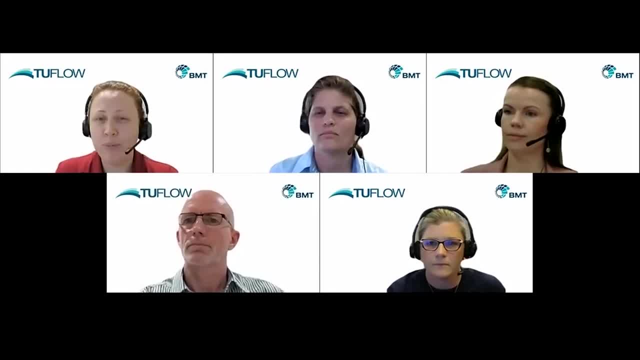 that we kind of do a sensitivity assessment, show the maps and move on. I think we could be doing better in terms of integrating and looking at areas that will be particularly vulnerable based on old design standards and how that will change with future conditions. Thank you both. 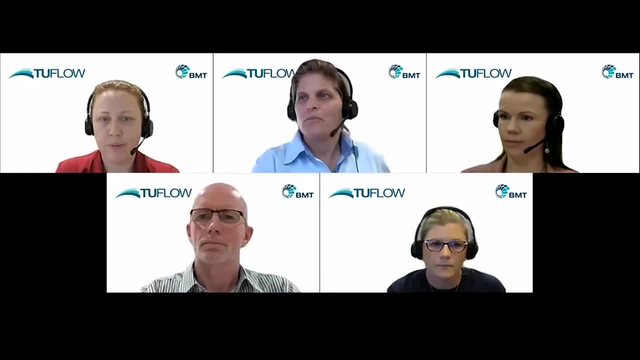 I think that's really sums it up really nicely. Just wanna say to everyone thank you for attending, And I really love having these questions coming in and being able to answer them, And it just demonstrate also that attendees are coming from a range of different countries. 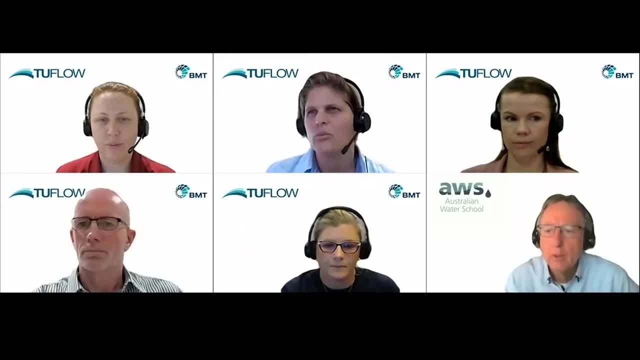 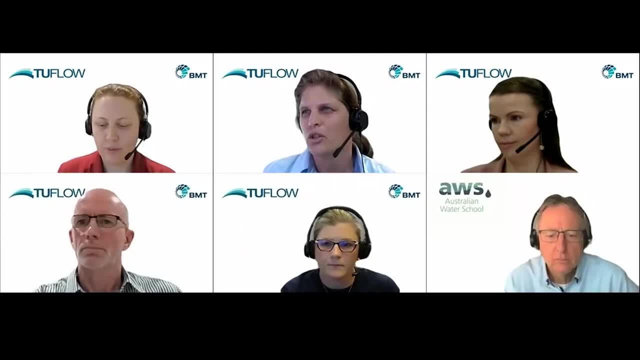 So I think it's really, really, really good We might try to get in one more here and go for this one- How the fit for purpose approach could be considered when integrated solutions are emphasized every day. To me, this is the person. 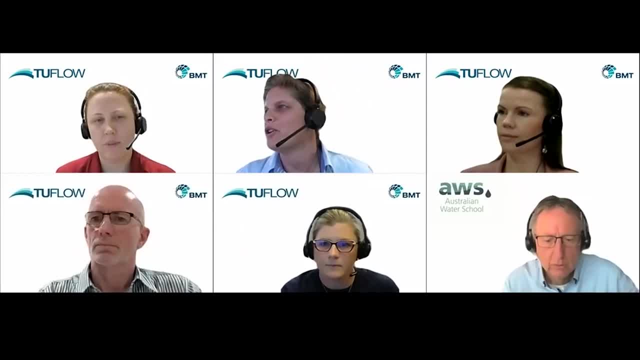 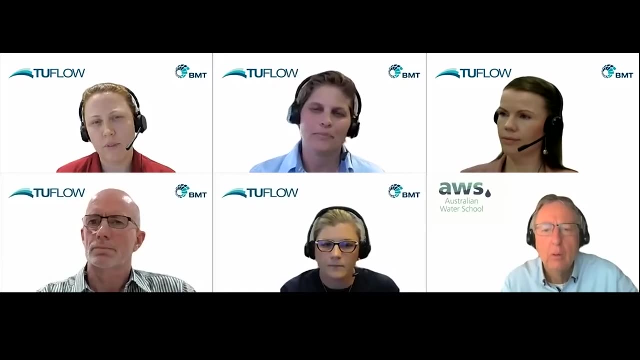 to me, resilience and sustainability can be compromised if we focus on the purpose only. I'm interested to hear on your thoughts on this. So I repeat, how the fit for purpose approach could be considered when integrated solutions are emphasized every day. Maybe, Jacqui? 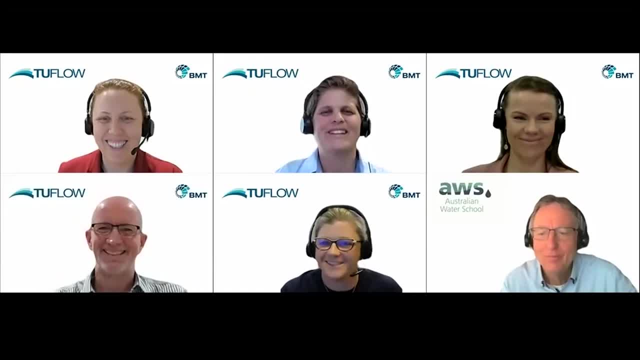 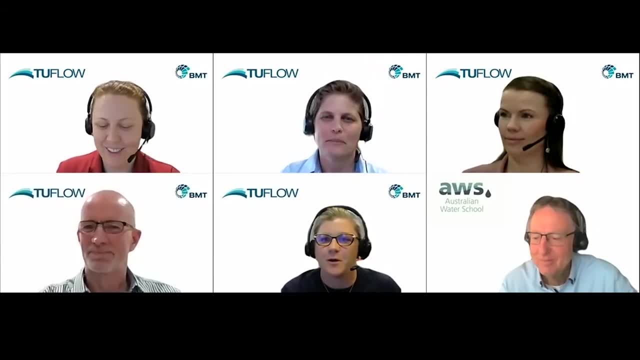 Thanks, Anne. I feel like I'm your favorite to throw to first. We've got a routine going, I suppose, really. yeah, I suppose a lot of our talk was about that fit for purpose approach. So I suppose, first and foremost, you need to be tailoring your approach. 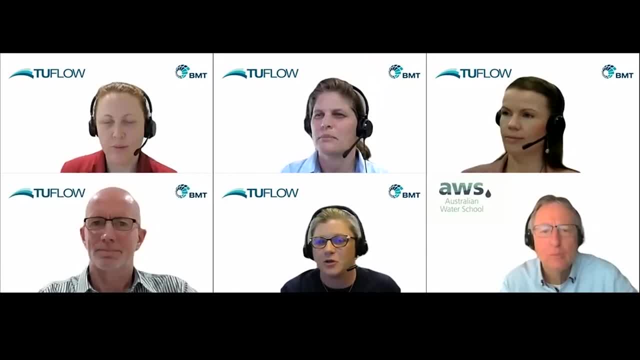 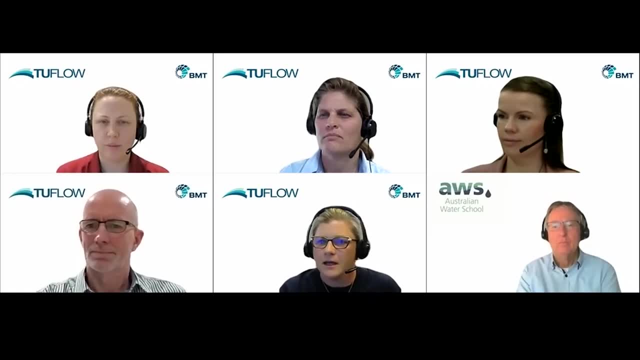 to the actual project that you're doing, And those things like the needs of the project, the needs of the client, the community, the needs of the catchment could be considered when integrated solutions are emphasized. Yeah, I suppose if you're using 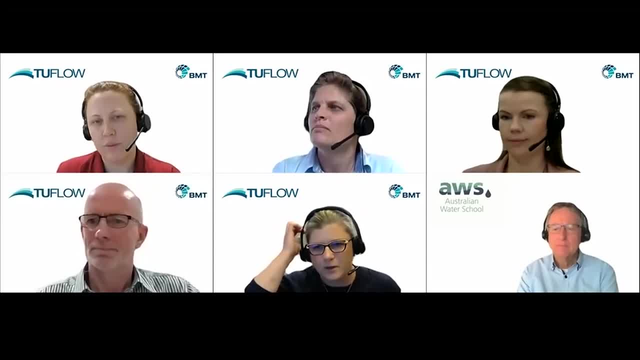 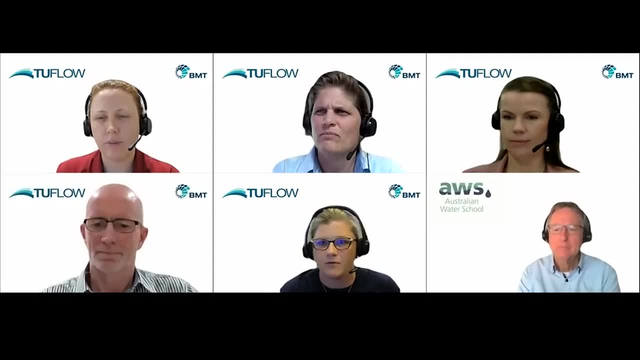 those underlying best practice principles. you know that's where you're trying not to compromise. So, really, you know that community resilience is the overall aim of the best practice principles. So hopefully, if you're, you know, trying to apply those within the realm. 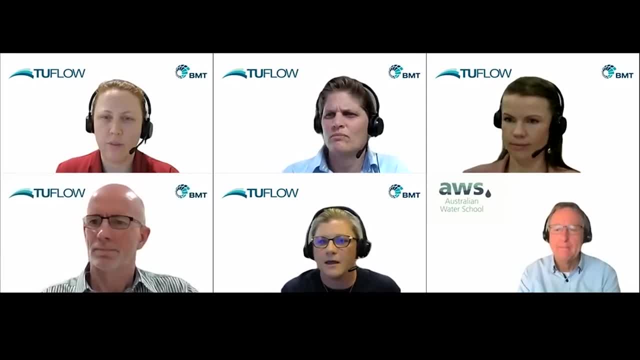 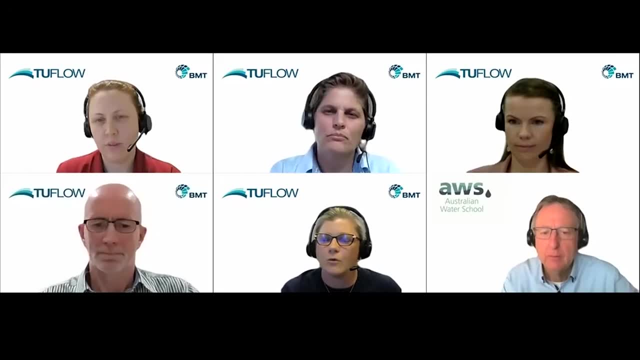 of this fit for purpose approach, you're not losing that focus on resilience and sustainability And I suppose recognizing you know that we can try and be all things to all people, um, but sometimes that's a bigger challenge perhaps, um, so I suppose we need to perhaps focus on on what we're trying to achieve. 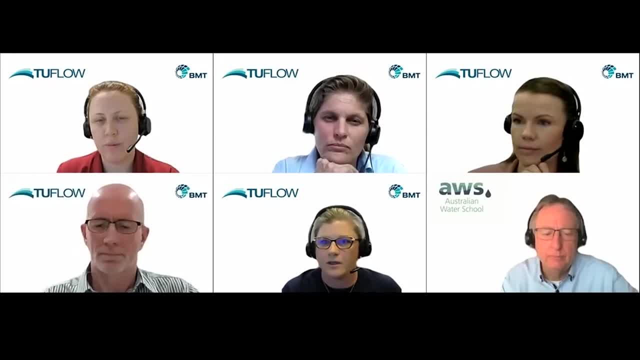 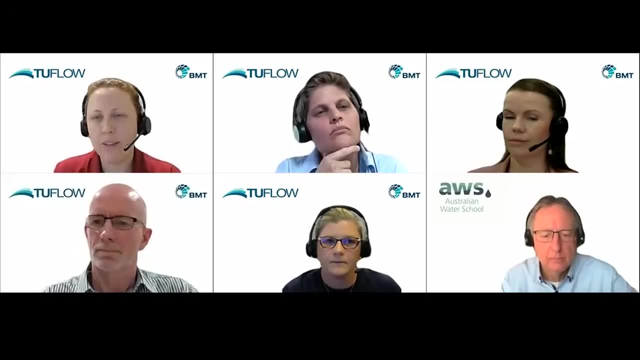 with that plan and, yeah, not try and be everything to everyone. Carrie, did you want to add anything? yeah, I mean, I'd build on that. I think it's pretty much what you're saying, but it's up to you how you define your study, how you set the boundaries, the parameters, um who you include as stakeholders. 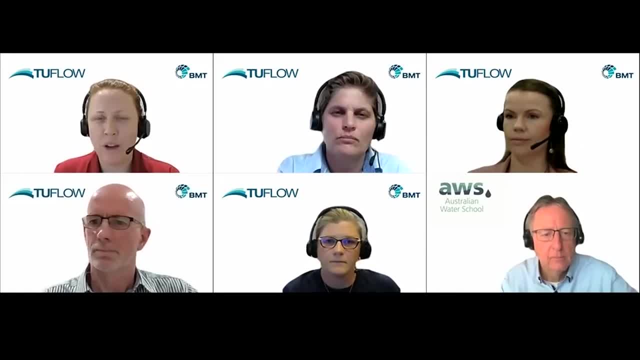 what you want to achieve for the outcomes and when you're going down to assessing measures. your multi-criteria assessment: um, if you have an idea of what good looks like if one of your measures is improves community resilience. if one of your measures is one of your criterion is is 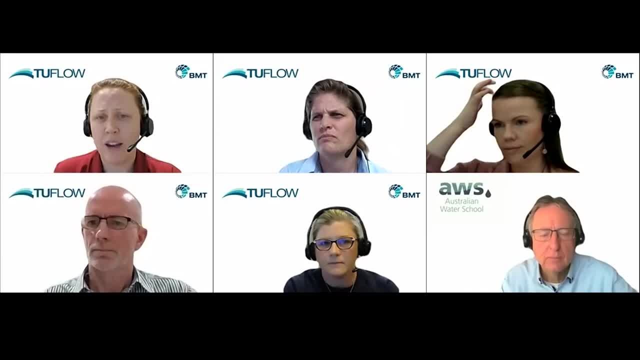 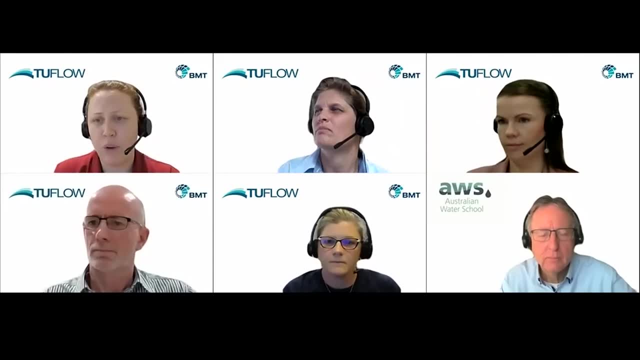 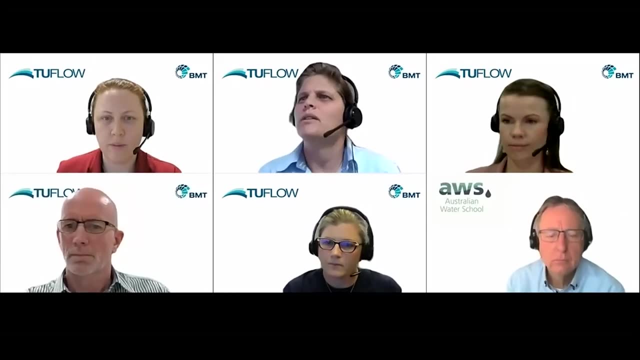 improving community resilience. if you've got criteria set up that it works with with other factors, that there's environmental benefits, that there's sustainability benefits, so you can set up those, those metrics and that framework to support your overall goals. let's go back to this one um, which has been sitting there since. 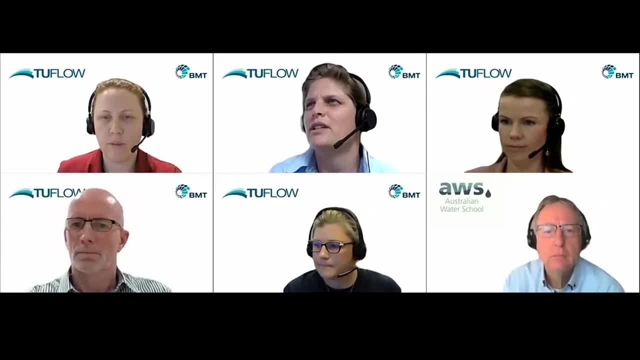 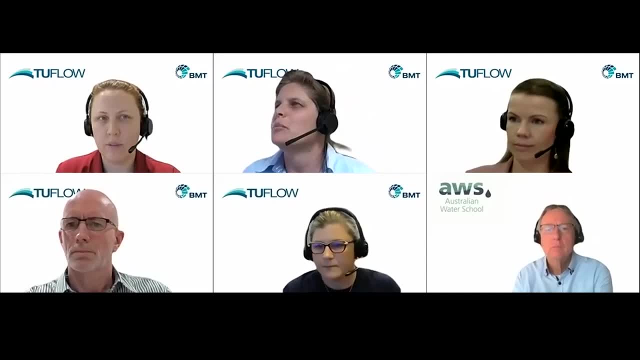 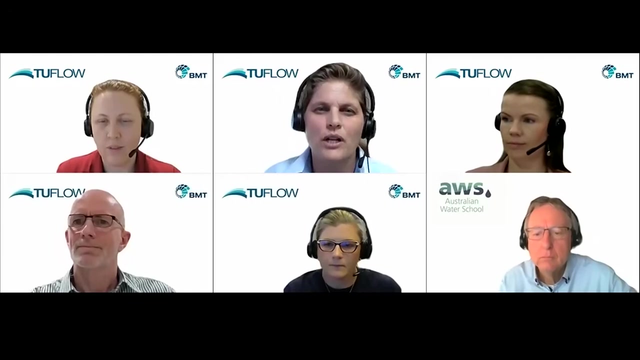 the start, when modeling flood related overtopping dam failure scenario associated with an extreme rainfall event, for instance the PMP event, what background flood AP would you recommend and adopting for the catchment downstream of the wall? um, maybe that could be something um for carry, but I thought I'll jump. 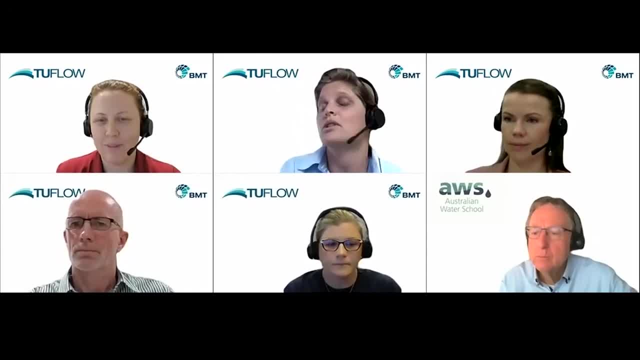 in there a little bit as well. I think it's important to to consider two scenarios: one upstream of the dam, one downstream and obviously needs to be a smaller one, not the PMP as a smaller event such as the 100 year event or something like that. um, yeah, I think the main thing I'd add. 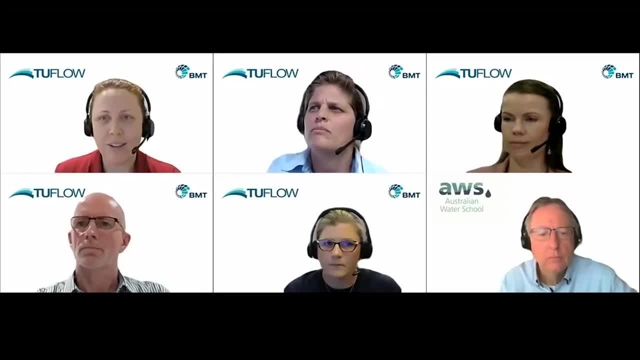 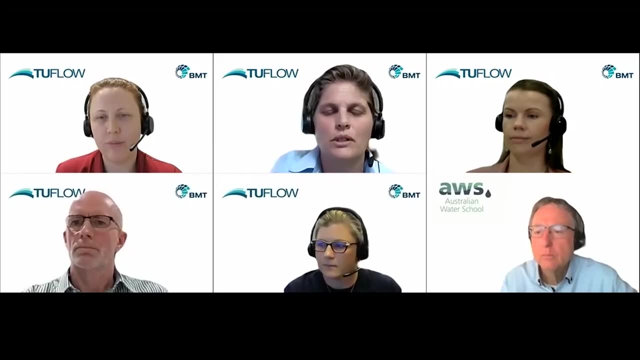 is that dam um scenarios are often strongly controlled um in terms of what you have to apply, what you have to model, so definitely refer to your local guidelines and legislation requirements. yeah, in Australia we we certainly have um, have um, um strategic guideline on that as well. any final comments, uh, from anyone? 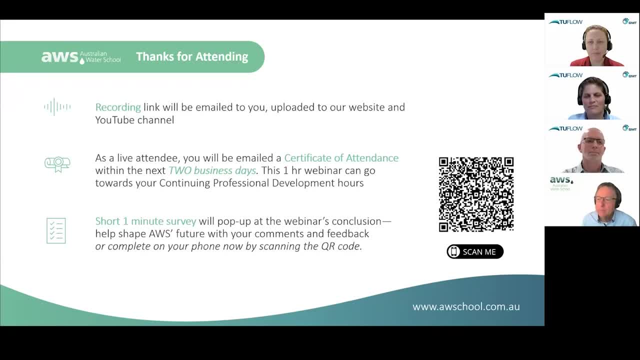 Bill Tegan, Jackie Carrie and all good. thank you all for attending. it's great to have you on the other end of the screen. yeah, thank you. Thanks to the Australian Water School- A great pleasure- And thanks Joel and Sam at the other end of backing this all up.